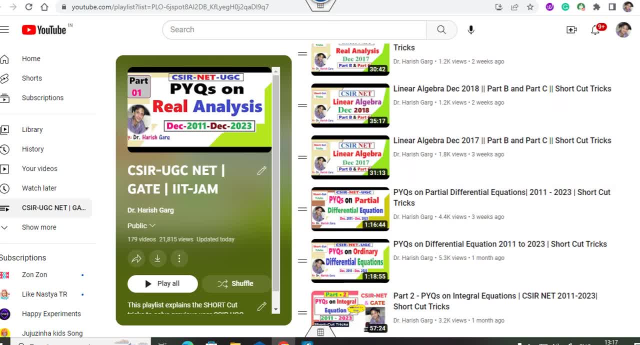 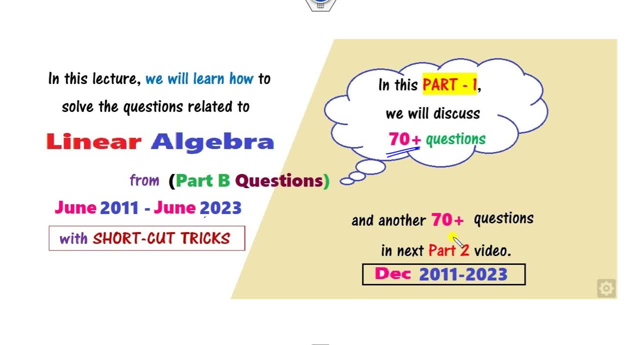 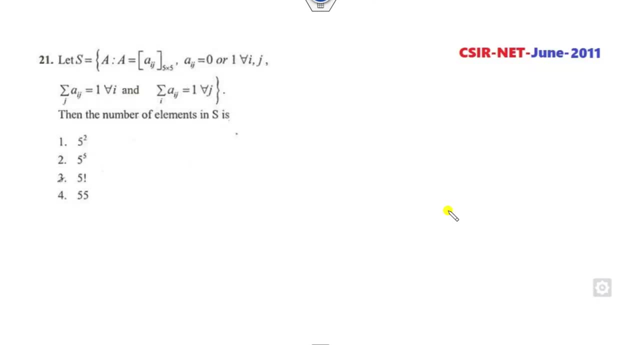 You can see the shortcut fix in as well. So let's start with this video. We will cover the 70 plus question in this part and the next 70 plus question related to the December 11 to 23, in which we will upload it after this video. So let's start with this one. So remember, whenever you are solving the linear algebra question, read the statement very carefully. What is given to you, A, is a 5 cross 5 matrix. 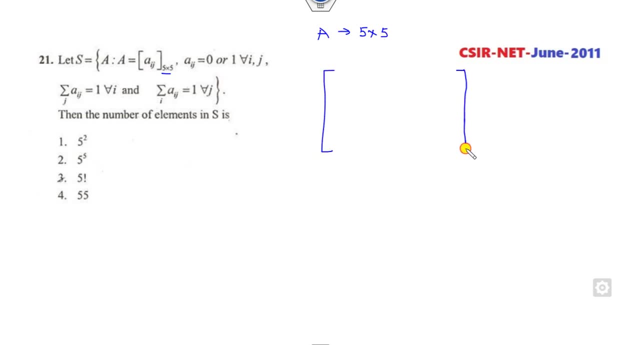 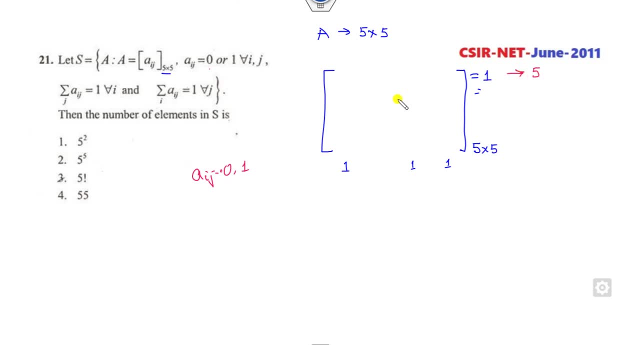 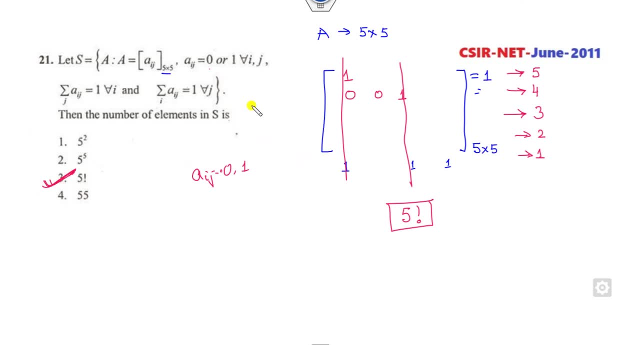 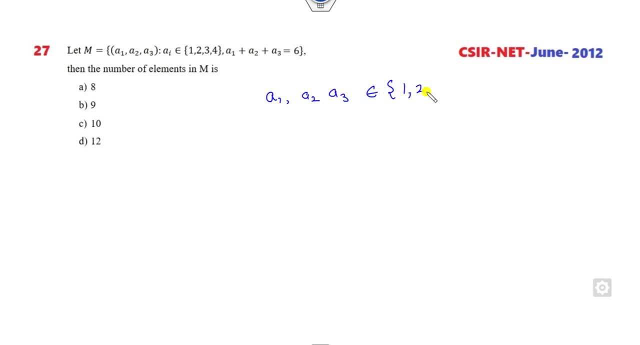 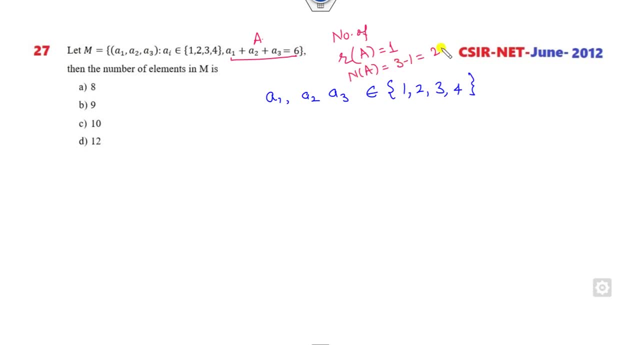 of this matrix you can see 3 minus 1, 2, so you have the two independent vectors. now, if I can choose, what is the choices of the a1 a1? you can choose either the 4, you can choose either 3. you can choose either 2 and you can choose either 1. so there are four choices for the a1. now what are? 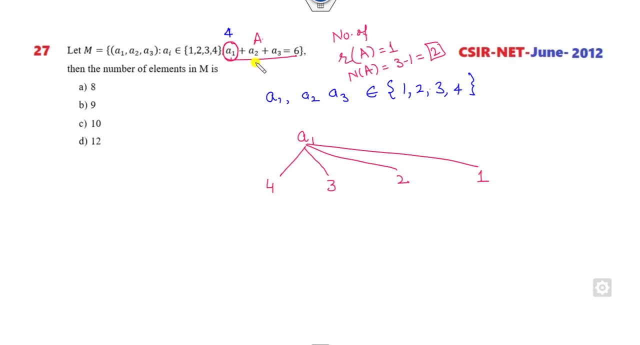 the choices for the a2. if you take a1 as a 4, it means this sum will be my 2 and since none of the number is my 0. so what are the those values? both is my 1 comma 1, so that means there is a 1 choice. 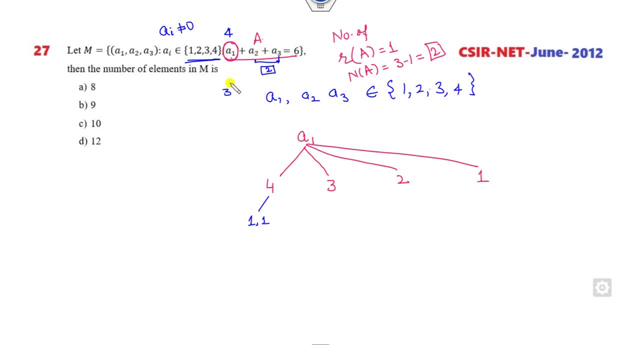 for them. when you take a1 is 3, the sum of them will be 3. so what are the choices? either you can take a2. this is a choice for the a1. what is the choice of a2? either you can take 1 or you can take. 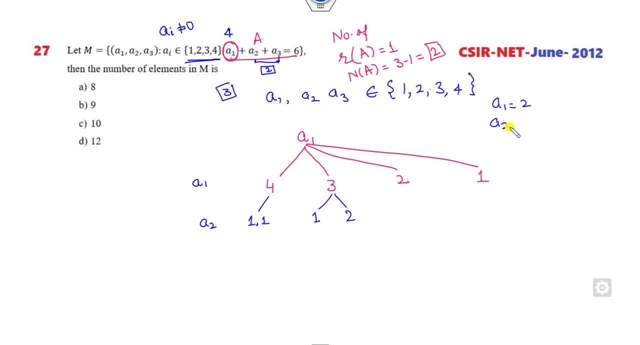 2. if I take a1 is my 2, then what is the choices of the a2 plus a3? it must be my 4. so what are the choices for that? either you can take a2 as a 4 or you can take a1 as a 2, either you can take a2 as a. 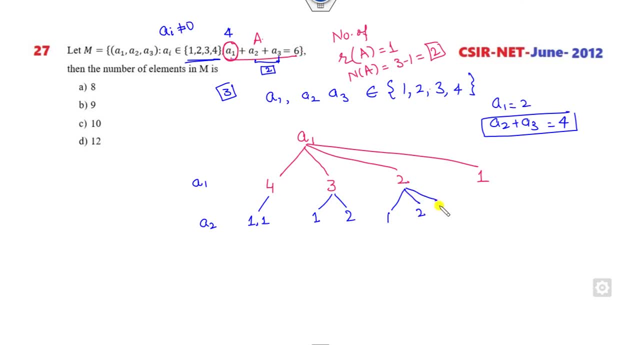 1. either you can do as 2 or either. but you can never take as a 3, because if you take as a 3, what will happen? it is possible also, if it is 3, then other value will be 1 as well, if you take. 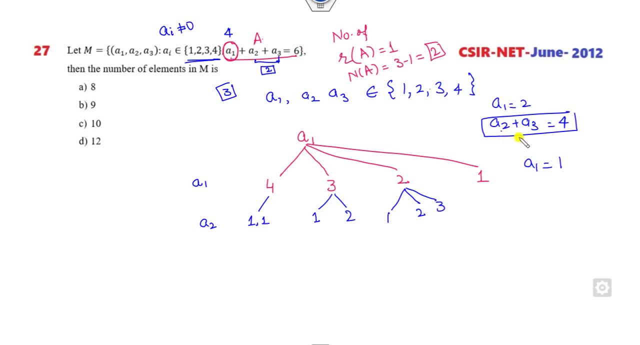 a1 is my 1. what? what are the choices for the a? what is the a2 plus a3, it will be 5. so what is that? it could be 4, it could be 3, it could be 2. so how many choices you have. or it could be like: 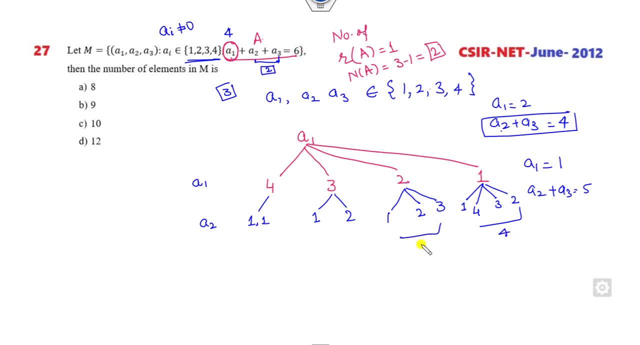 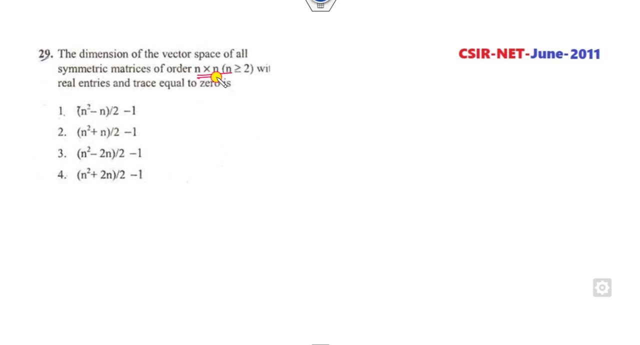 of 1. so how many choices you have? 4, 3, 2, 1. so 4, 3 plus 2 plus 1. so 4 plus 3 plus 2 is the right answer of this problem. look at that dimension of the matrix. now here is given to you n cross n. 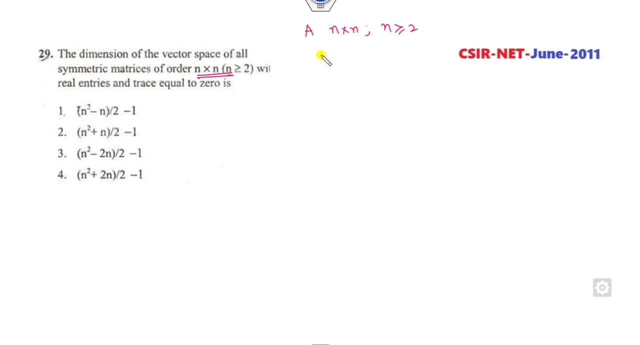 so what is the shortcut tips for you? you always choose the value of the n as per your convenience. here the simplest way is you can choose 2 cross 2. fine. now, once you said 2 cross 2, you have to find the dimension real entries. trace is my zeros. if i call this is my a, there is no need to find. 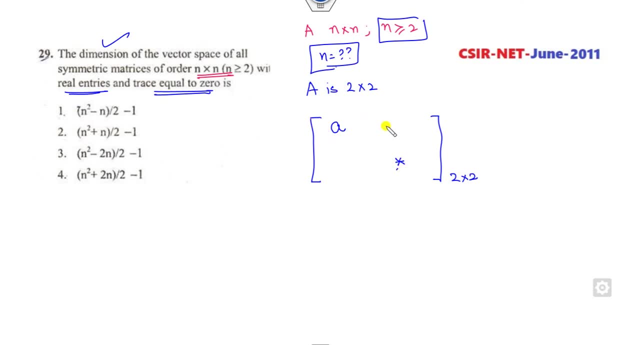 this value, because you know this value will be minus a and you know this is symmetric matrix. if this is my b, then this number is automatically. you can compute as a b. so how many unknown vectors in this 2 cross 2. that is my 2, so that means you can check what. 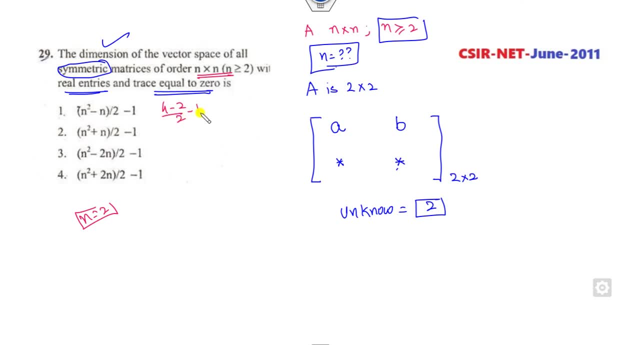 will happen if n is equal to 2, so it is 4 minus 2 over 2, which is not equal to 2 because my so this option is cancelled. 4 plus 2 over 2 minus 1 is a 2, so there is a correct answer: 4 minus 4. 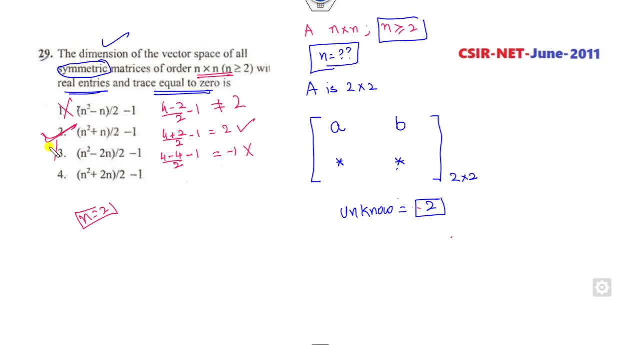 over. 2 minus 1 is minus 1, which is not equal to 2. cancel out 4 plus 4 divided by 2 is 3, which is not equal to 2. so right answer is only my b is the correct answer. simply, you can choose any of the pair. you can choose 3 cross 3 as well, but the simplest way is: 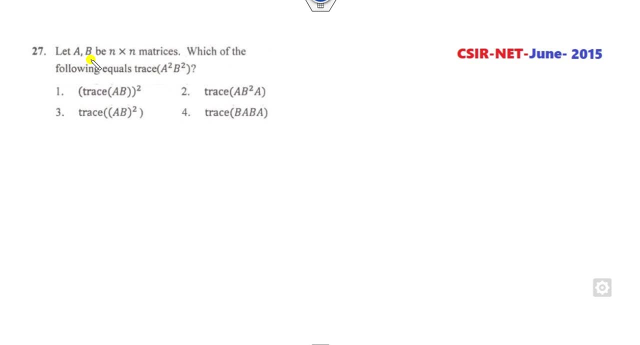 2 cross 2. okay, look at that. a and b are my n cross n matrix. so again, you can simply choose as my 2 cross 2. so if i take, a is my i, because nothing is given to you. so what is the meaning of that? 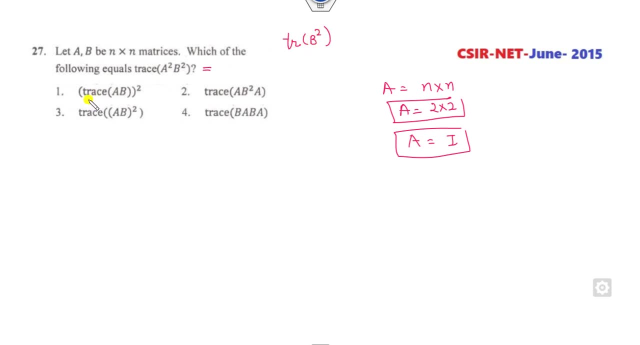 this will be my trace of b square. so look at that. the first answer option will be trace of a- b. if a is my i, then a b will be i, so it is a whole square. that's a wrong statement. why? because we know if b has the eigenvalue this, then the b square has the eigenvalue this, then what is the? 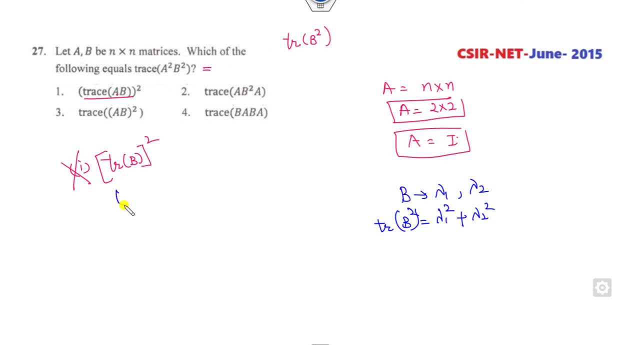 trace of the b square. it is this one, but trace of this is here, so it is not equal to this, this pair. so the first option is cancel. when a is equal to i, this is a trace of b square. that's the same, but we can never say it's a correct answer whenever you provide the example counter. 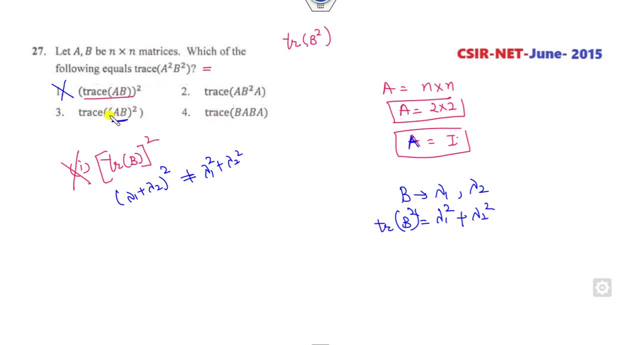 example, your target is to discard them. this is trace of b square, again same. this is trace of b square, again same. so it means nothing is to be discarded. now what is that? if i consider a is equal to b, both are same. so this is my trace of a raised to power 4. this is again a raised to. 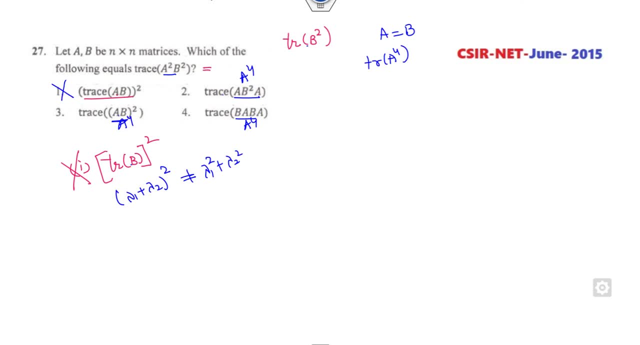 power 4. this is again a raised to power 4. this is again a raised to power 4. so, again, this example does not give you. then what is the tips for you? so we all knows trace of the a, b, c, which is nothing but my. you can change them to be here: c, a, b. remember this is applicable only for the three. 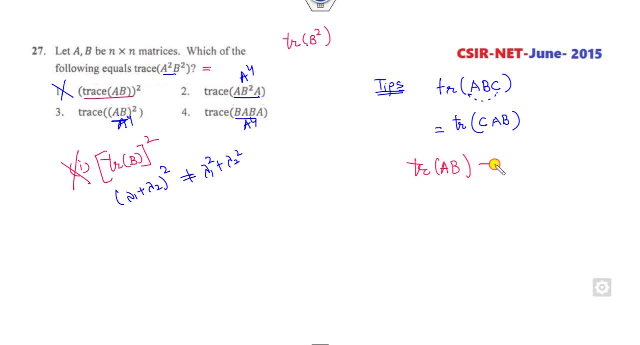 case, the, the, the, remember. this is not true. you can't say for the two, you can't say you can change them to be here. this is not true. this is only applicable for three or more than three. so now what will happen? if i write a square as a, a, a, b square as a, b, b, fine, now i can change them to be here. so it is a, b, a, a, b. 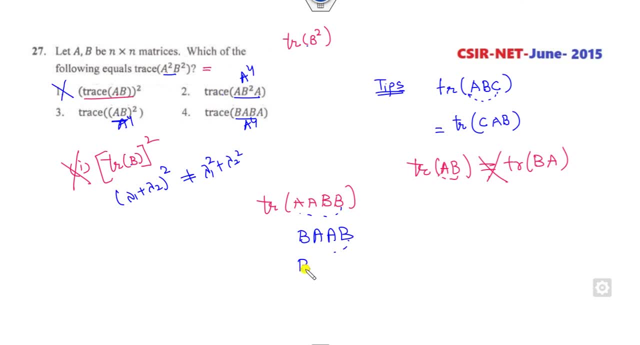 is there any pair? no, again, i can change b b a a, is it anyone? no, this is a b b a, not match. again, we can change a b b a. is this match a b b a? so this is the right answer of this problem, if you. 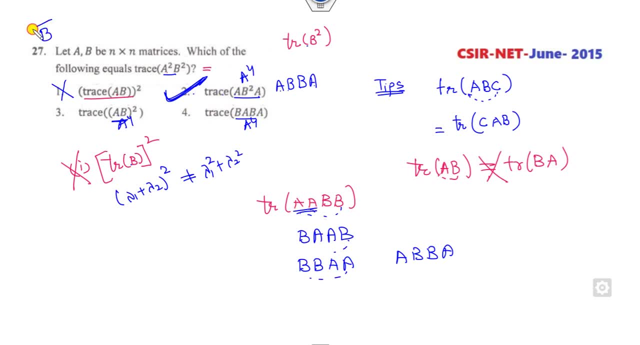 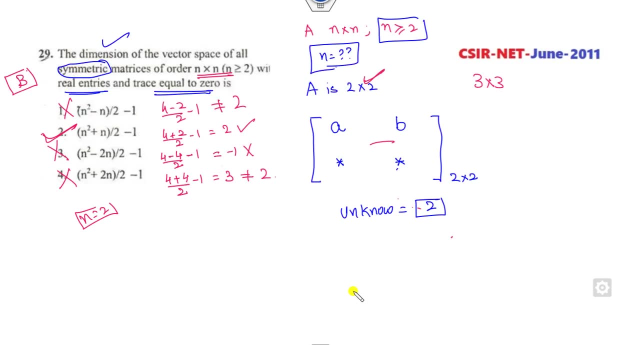 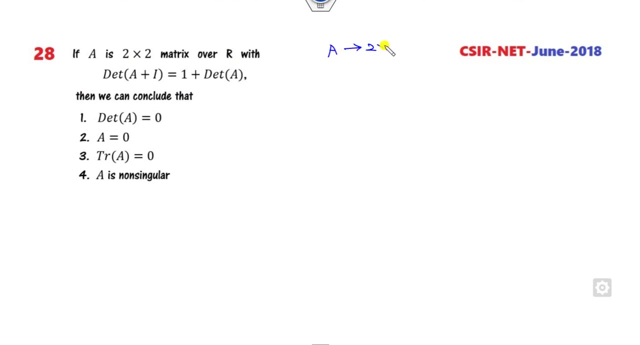 want to again change, then it's again the same. so this is the right answer. b is the correct answer: rest. all options are cancel. okay, now look at this next question. a is the any two cross two matrix such that this will be here. that's very simple. whatever. whenever there is a matrix, you can think about the eigenvalue. 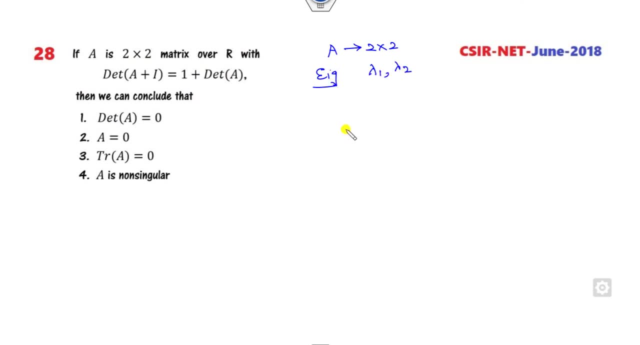 what are the eigenvalue of this? i can simply take lambda 1, lambda 2. what is the eigenvalue of the a plus i? this is my eigenvalue of the a plus i. now you can substitute here. what is the determinant of this? there is a product of the eigenvalue which is one plus of. 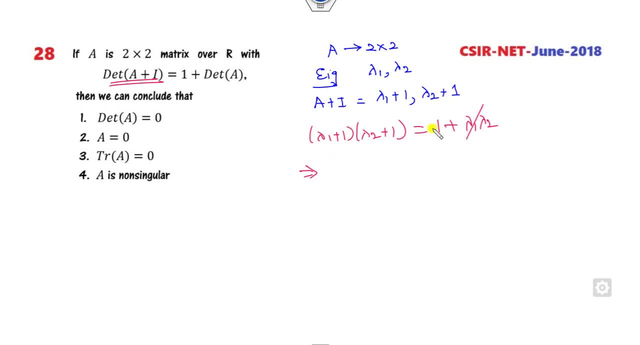 you here now. if you open them, this will be cancelled. one will be cancelled. the only pair will be here. what is the meaning of that? this is trace of a. is my 0 is the correct answer. okay, now look at this one again. it's a n cross n and n is my 2, so i can simply take: is my 2 cross. 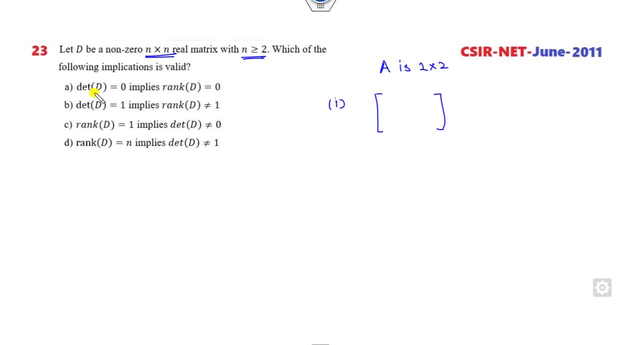 2 matrix. fine, now think about the first option. determinant is my 0. so what? what you can think about that? this is my 2? cross 2 clearly says that the determinant of this matrix is 0. satisfied. what is the rank? rank of this matrix is my 1, which is non-zero. first option: cancel out. 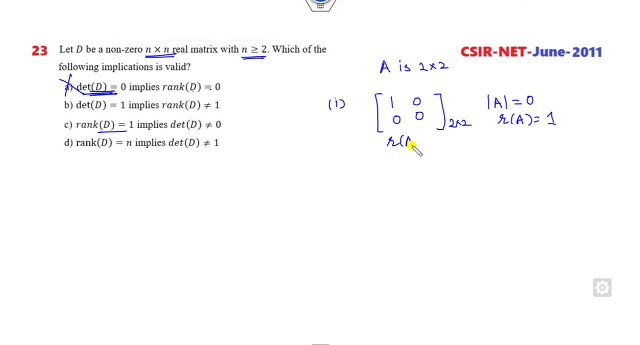 again, you can see the rank is my 1. this again, example satisfied. what is the determinant? the determinant of this is my 0, but he said non-zero. this option also cancel out. then think about: the determinant is my 1. so this is the example where you can see the determinant is 1. what is the rank of this matrix? rank is my 2. 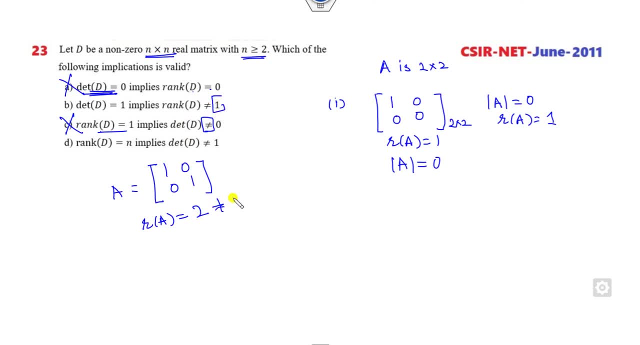 but it said not equal to 1. that's also correct, not equal to 1. so we can't see anything. look at that. i have taken: n is my 2, rank is my 2, so again you can see: rank is my 2. determinant is not equal to. 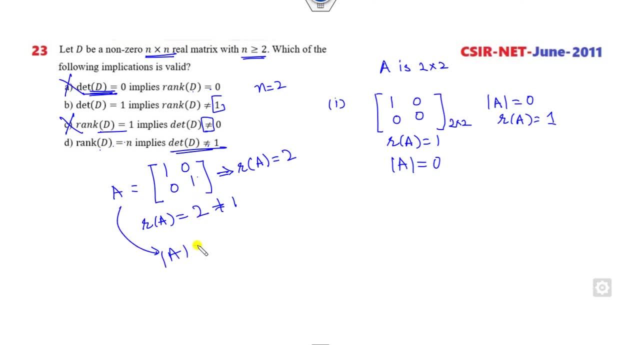 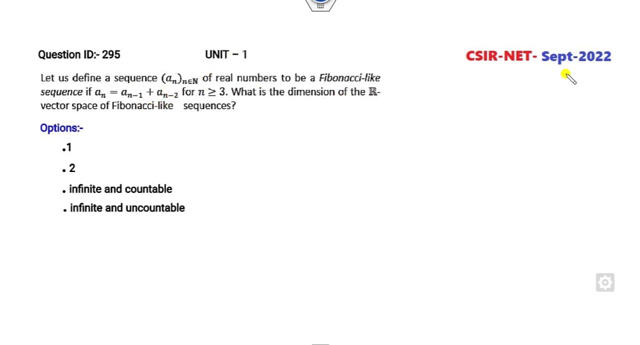 1, but you can see what is that determinant of this matrix, which is 1, so this option is cancel out. right answer is my b. whenever there is a n cross n, you can take the example for your own convenience. again, you can see: this is a 2022. 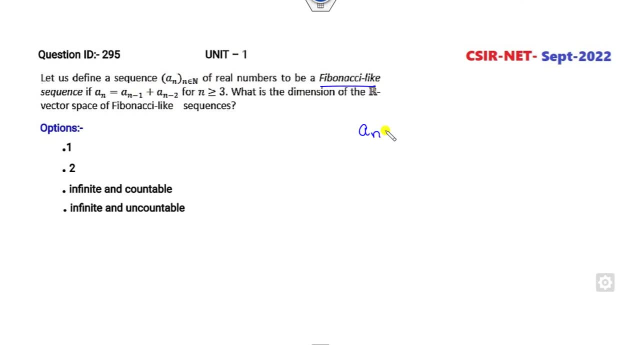 a sequence of the fibonacci series is defined like of this one: a n minus 1, a n minus 2, for all and greater than so, can i write this: one: a n. a n minus 1. a n minus 2 is 0. so how many variables are there? number of the variables are my 3. 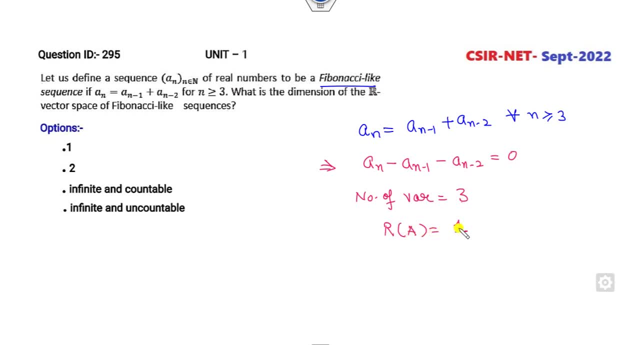 what is the rank of this matrix? clearly say it's a 1, so the number of free variable, or you can say the nullity. what is the nullity of this is 3 minus 1, is my 2, and your target is to find, because this: 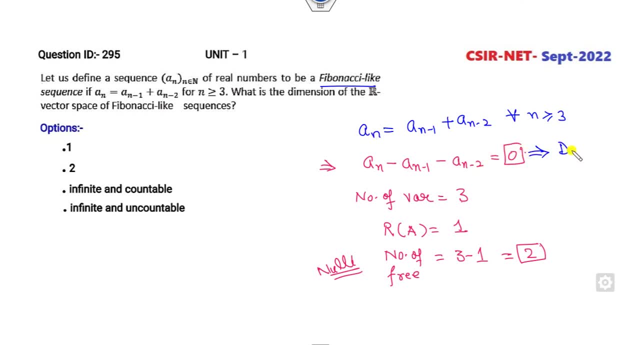 is right hand side is 0. so what is the meaning of that? i can return this as dimension of the ax is equal to 0. that is the rank of this matrix. so that means if i write this as a x is equal to 0 is nothing but my nullity. so what is the nullity? is my 2 is the right answer, okay. 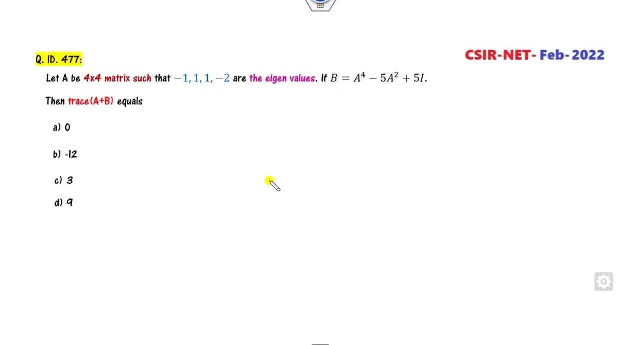 okay, what is the trace of the a plus b? we all know trace of a plus b is trace of a. trace of b. a are the eigenvalues. what are the trace of this? some of them it is minus 1. what is the trace of? we need to find that when a has the eigenvalue minus 1. so what are the eigenvalues of the b? 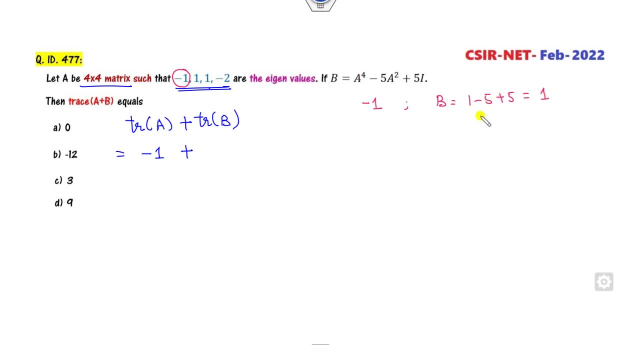 1 minus 5 plus 5, that is a 1 when it has a 1 eigenvalue. so b again has the 1 minus 5 plus 5, 1 when it is again 1. so again it has a 1. when it has a minus 2, then b will be 16, it is a 4, 20. 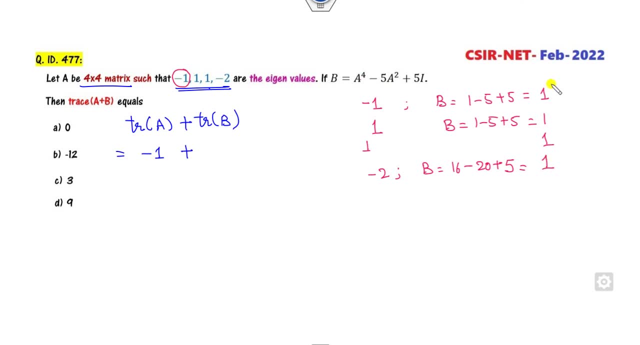 it is a 5, so it is a 21, it is a 1. so what is the trace of this? what is the trace of the b? these are the eigenvalues of the b, so trace is my 4. if you substitute them, answer is my 3 is the correct answer. 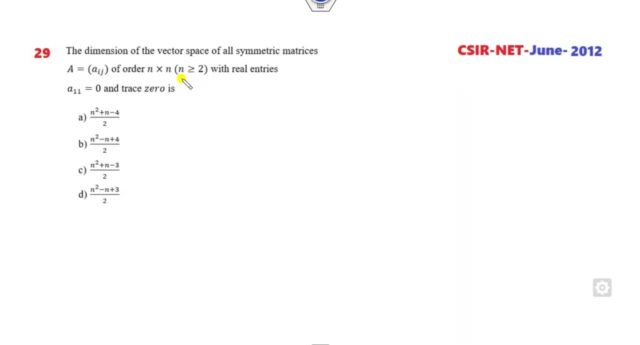 now again it is n cross n, so i can simply take a 2 cross 2 matrix. fine, so it has a 4 element, so a 1, 1, 0. so this is my 0. trace is also 0, so definitely this number will be my 0. 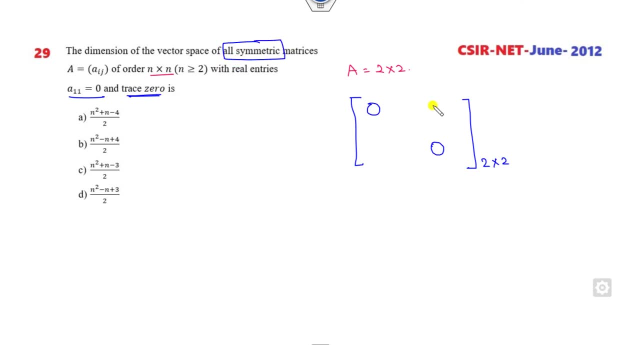 okay, So there is no need to them. It is a Smith-Wick matrix, So if I consider this is my a, then there is no need to find this. It is automatically be a minus a. So how many independent variables are there? 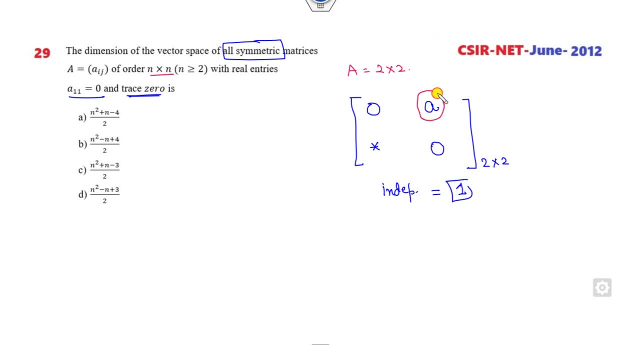 There is only one variable called as this element. So now I take n is 2.. I can substitute here, Check, whichever answer is 1.. So it is 4 plus 2 minus 4 over 2 is a 1.. 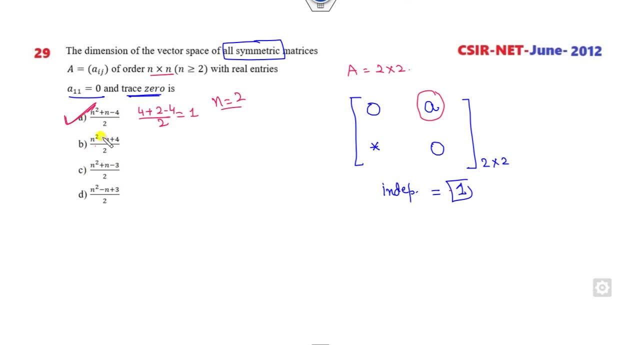 Correct answer Because there is only one correct option. that is over, But we can check others also. 4 minus 2 plus 4,, which is not equal to 1.. 4 plus 2 minus 3 over 2, is not equal to 1.. 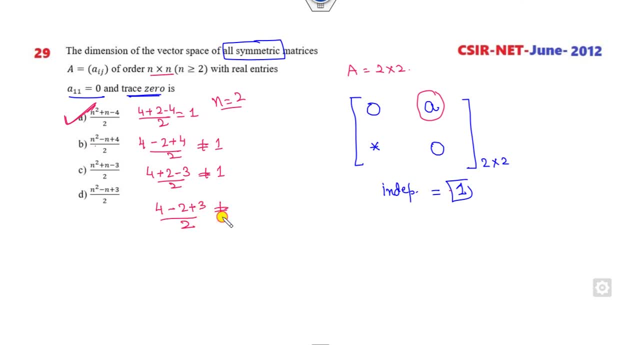 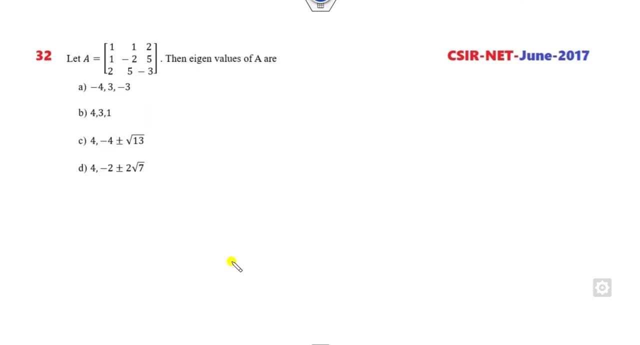 4 minus 2 plus 3 is again not equal to 1.. So the right answer is only my. a is the correct answer. Okay, which of the following is the eigenvalue? So we all know what is the properties of the eigenvalue. 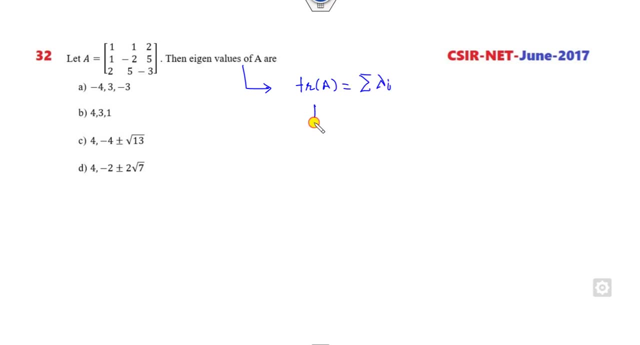 Trace of the. a is sum of the eigenvalue. Determinate of a is product of the eigenvalue. What is the trace? You can see the trace will be minus 4.. Now you can see the sum is minus 4.. Fine, the sum is not minus 4.. 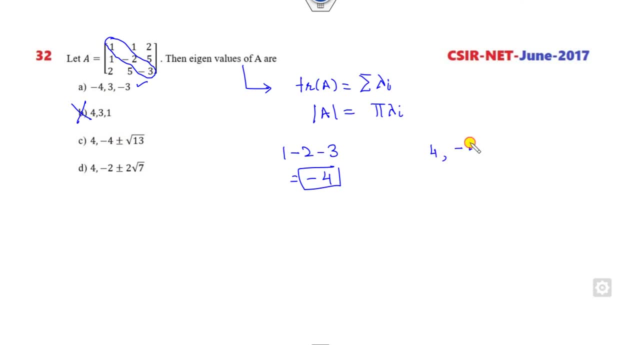 Sum is not a minus 4, because the eigenvalues are this and of this. So if you add them again, it is a minus 4 and it will be 4 minus 2 plus root, 7 minus 2.. So if you add them, it will be 0. 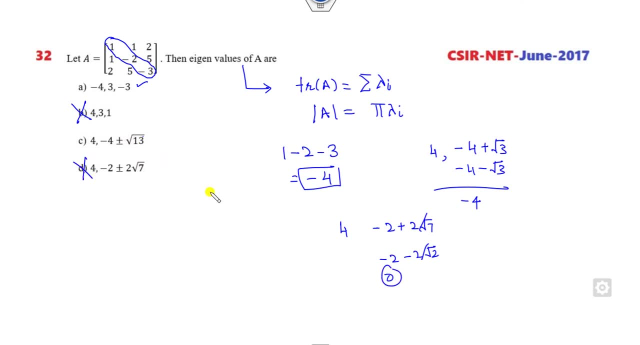 So now, out of these two options, 1 is the correct one. Now how you can check that The trace will be minus 4.. So both are the correct. Now you can find the determinate. So what is the determinate of the first one? 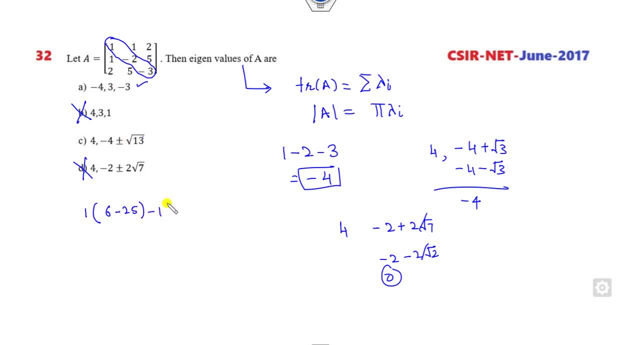 We can find it is a 6 minus 25 minus 1.. It is my minus 3. If I just clear this. So minus 1 will be minus 3 minus 10. And plus of 2, it will be 5 plus 4.. 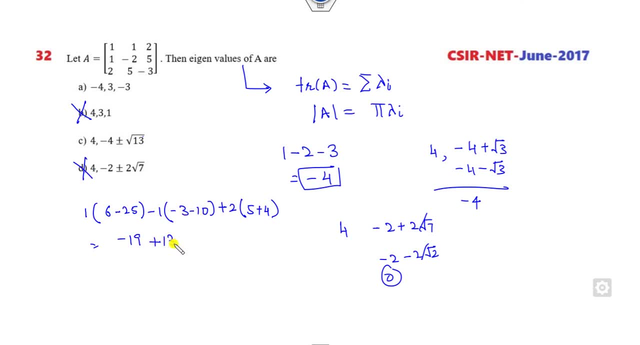 So what is that? It is a minus 19.. It is a 13.. Plus of 13 is a 10 plus of 20.. So it is a minus 7.. Sorry, minus 6 plus 20.. That is my plus 14.. 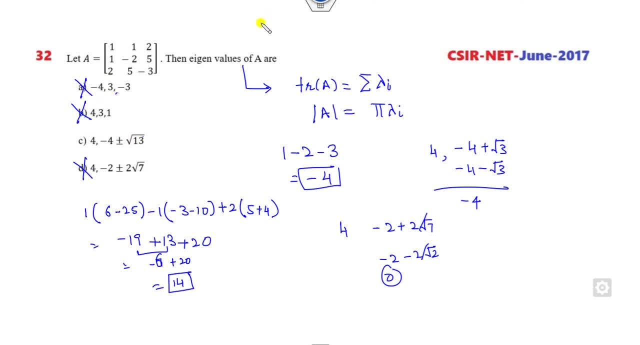 So is: the sum is 14? No, Can this be? the sum is 14?. So this? So what is that? It is a square minus b square. So what is that? It is a 3.. It is a 12.. 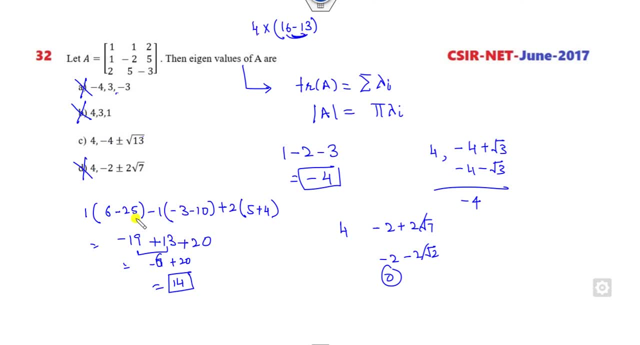 So again, it will not be there So you can check about this calculation again. It is a 6 minus 25 minus 3 minus 10. 5 plus 4. So it is a 9. 9 to the 18.. 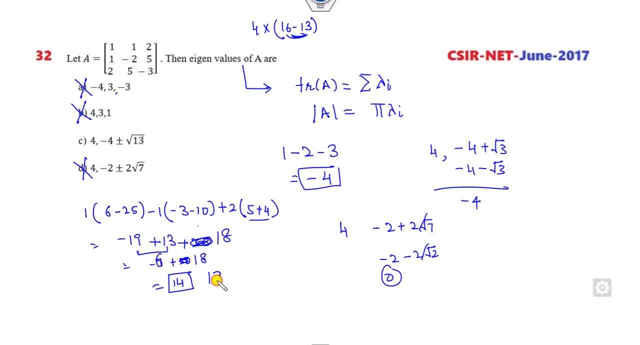 So what is that? It is a 6 and 18.. It is a 13.. It is my 12.. So what is that? It is 3.. 4 into 3 is my 12.. Is this the right answer? 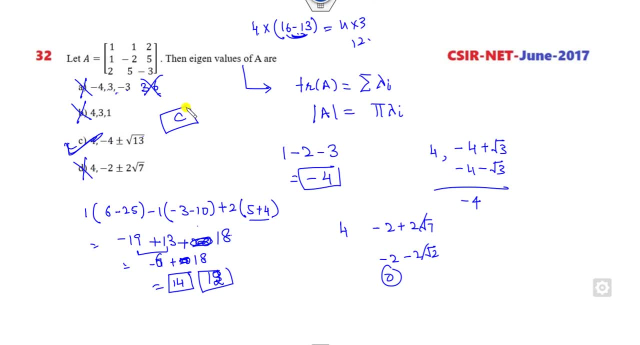 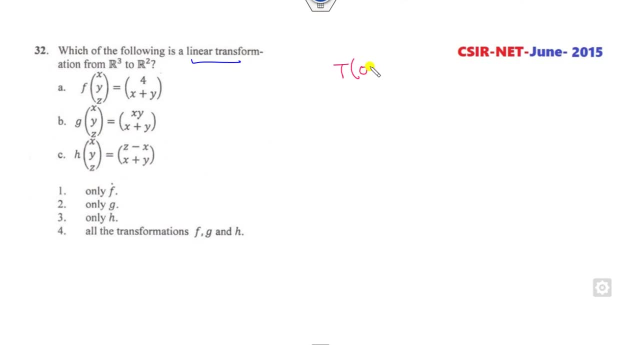 It is a 36. But it is not the right answer. So right answer is my C is the correct answer. So which of the following is my linear? So a very simple. Clearly see that x, y. 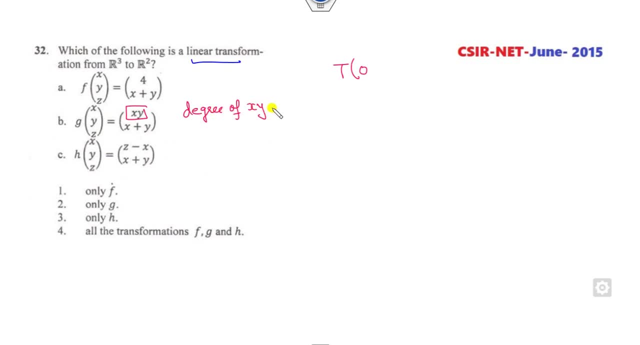 The degree of this? What is the degree of the x? y Is 2.. So it is a non-linear. So this option is cancelled out. What is the linear is: If t of 0 is non-zero, then we call as t is my non-linear. 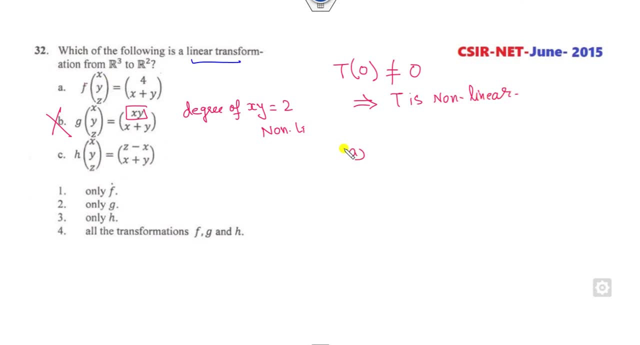 Fine. So what is the meaning of that? It clearly says the first option. What is f 0, 0, 0?? It is a 4, 0.. Which is not equal to 0, 0. So this is a non-linear. 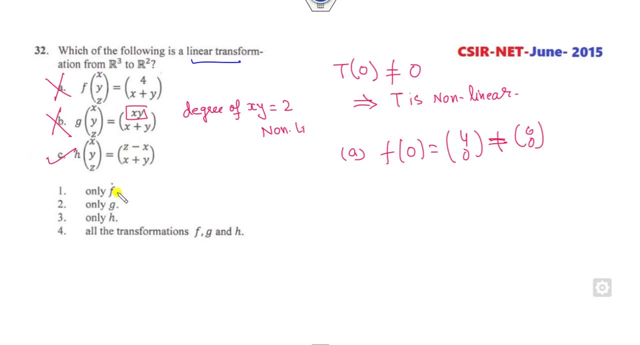 So it means this is the only correct option, Because if you substitute here: So only h is the right answer, f is cancelled, g is cancelled, All are cancelled, So right answer is only my. C is the right answer. 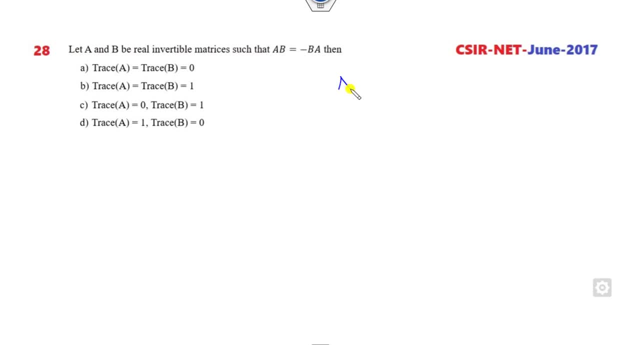 Now, a is a real invertible matrix, such that a b is equal to minus of b a. Then which of the following are here? So it is a invertible. Invertible means a inverse exist. Fine, Now which of the following is the correct option? 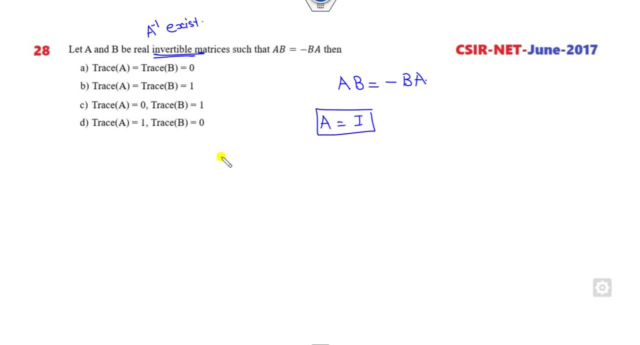 Very simple example You can simply take: a is i, which is invertible. If I substitute here b is my minus b. What is the meaning of that? Now, your target is to find that trace Trace of b is trace of minus b, which is minus trace of this. 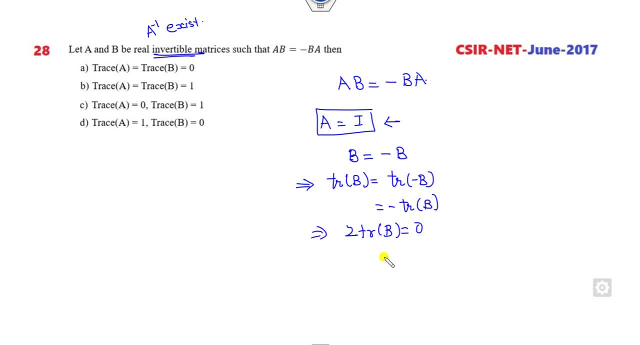 So what is that? 2 times trace of b is minus trace of this. So what is that? 2 times trace of b is minus trace of this. So what is that? So it is trace of b is my 0.. 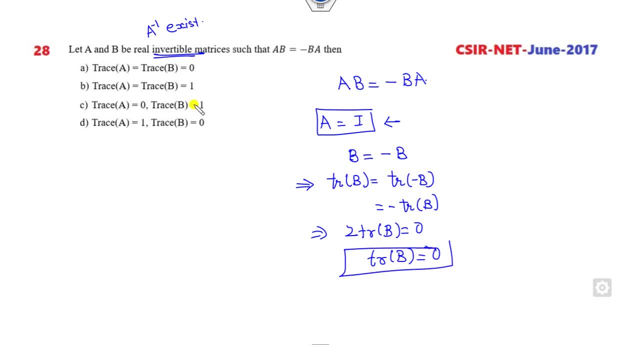 So it means trace of b is my 0. So trace of a. this b and c are cancelled. Now, similarly, if I consider b is i, because a and b, both are invertible, then you will get: a is equal to minus a. 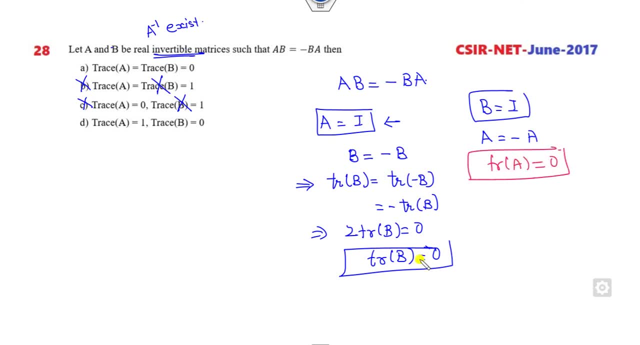 So it means trace of a is my 0. So both the trace are my 0. It is the simple, right concept, Because you can think any of the example, But the simplest one is you can think about invertible. i is always invertible. 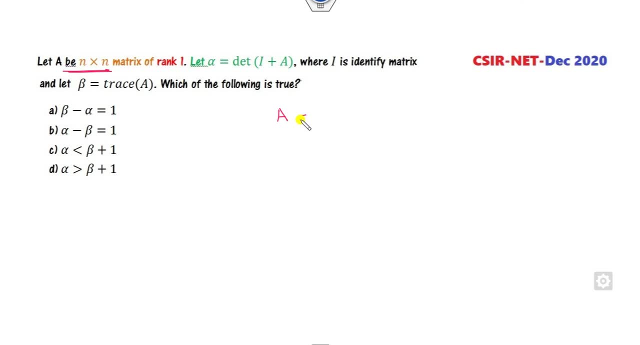 Okay Again, a is n cross n. You can simply take. a is my 2 cross 2.. Rank is my 1.. So if I take rank is 1, it means the 1 row will be 0. So if I simply take here, 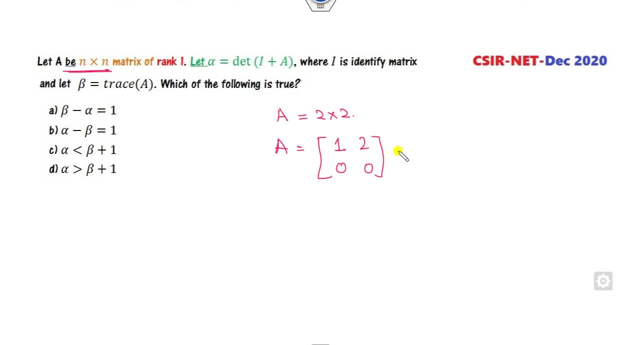 You may think about like of this also, It is my say 2.. Again, rank of this is my 1.. It satisfies this. Now, what are the eigenvalues of this? a Eigenvalue of this is my 1.. So it is my 0.. 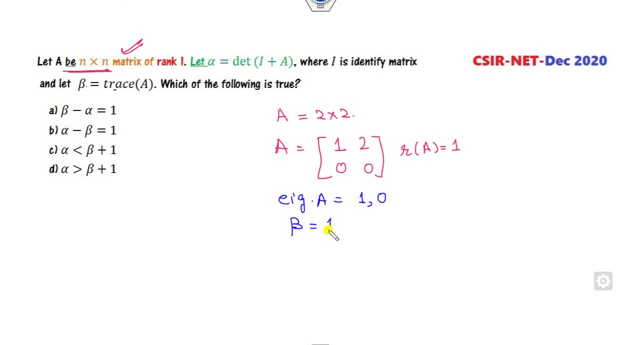 What is the beta? Trace will be sum, So it is my here Beta will be 1.. What is that eigenvalue of the i plus a? So you can add them 2 comma 1.. These are the eigenvalue of the i plus a. 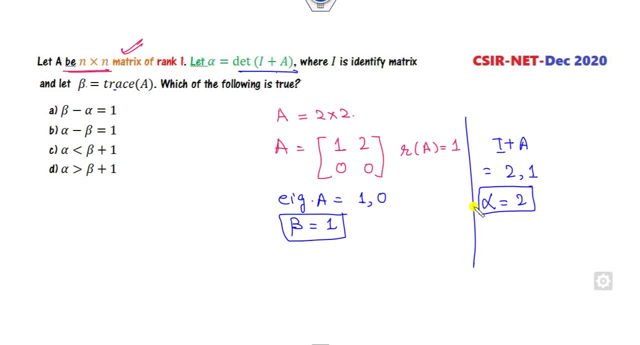 What is the alpha Determinate is my 2.. Once you know alpha and beta, check about this. 1 minus 2 is 1. Not satisfied. 2 minus 1 is satisfied. But this is a counter example. We cannot say it is a correct. 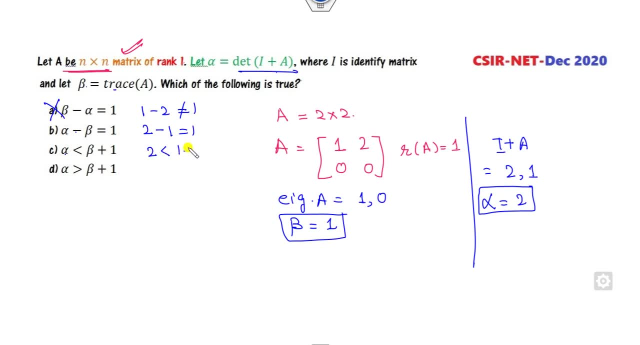 We cannot say it is a correct statement. Alpha 2 is less than 1 plus 1 is equality. It cannot be less than It is a cancel out. Alpha is greater than 1 plus 1.. Again, it is not satisfied. 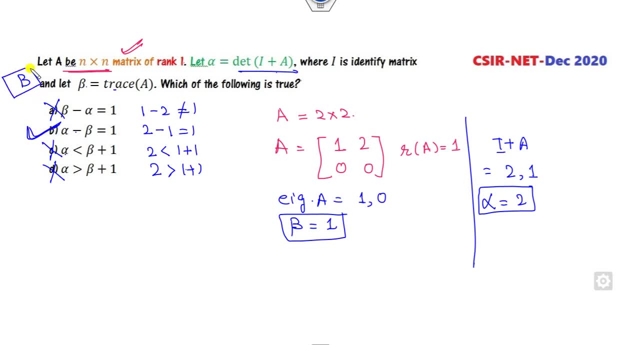 The only left option is b is the right answer. You can think that It is a very simple If you think about any of the matrix which satisfies such kind of the properties. Okay, what is the rank of this matrix? So it is a 5 cross 5.. 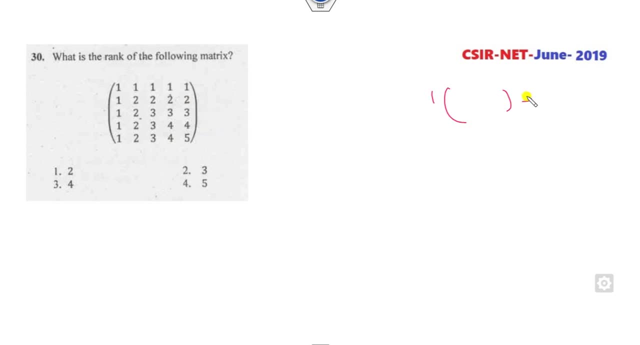 It is not an easy task for you. You can expand them, So what is the simplest manner? That is very simple If you look about these 2 last 2 rows. If I substitute r5 minus, So last value will be 0.. 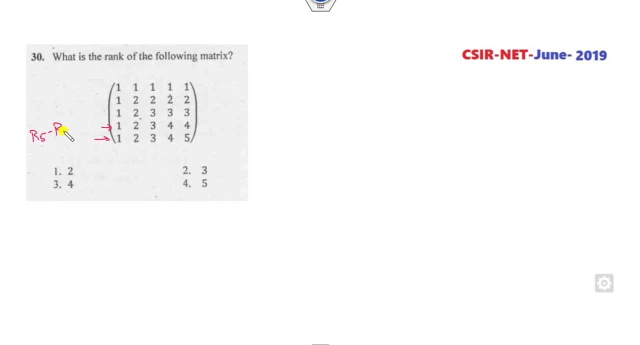 0, 0, 0, 1.. Fine, Similarly, if I take, If I subtract this from here, It will be 0, 0, 0, 1, 1.. Similarly, if I take like this way: 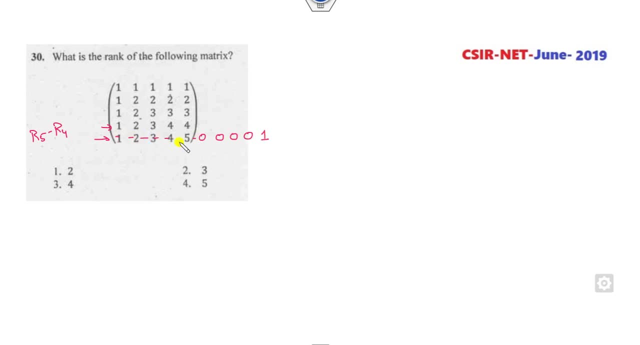 0, 0, 1, 0, 0.. Sorry, 0, 0, 1, 1.. 1, 0, 0, 1, 1.. Similarly, if I take like this way: 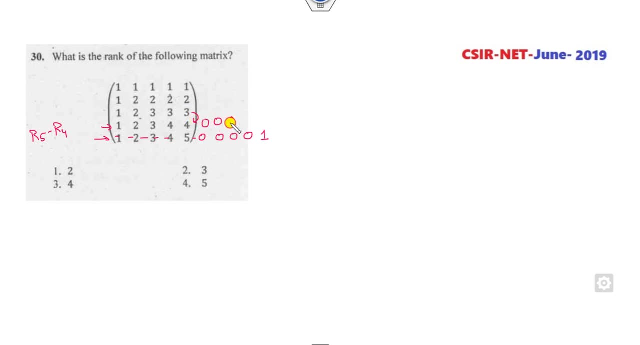 0, 0, 1, 0, 0.. Sorry. 0, 0, 1, 1.. 1, 0, 0, 1, 1. 1, 0, 0, 1, 1.. 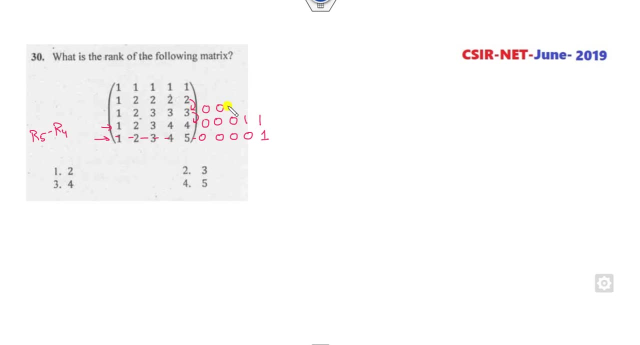 1, 0, 0, 1, 1.. Similarly, if I take like this way: 0, 0, 1, 0, 0.. Sorry, 0, 0, 1, 1.. 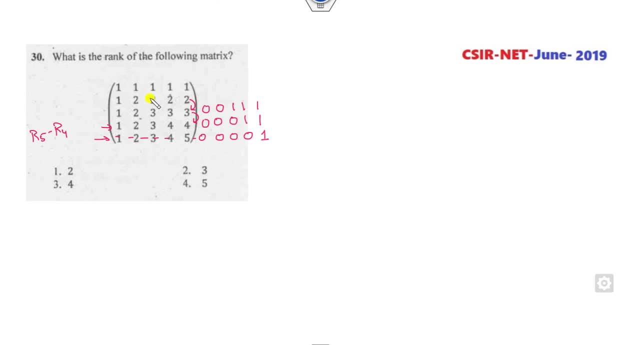 1, 1.. Same for here: 0, 1,, 1,, 1,, 1.. And the first value will be here. So what is that? This is the triangular matrix, And what are the Eigen values of this? 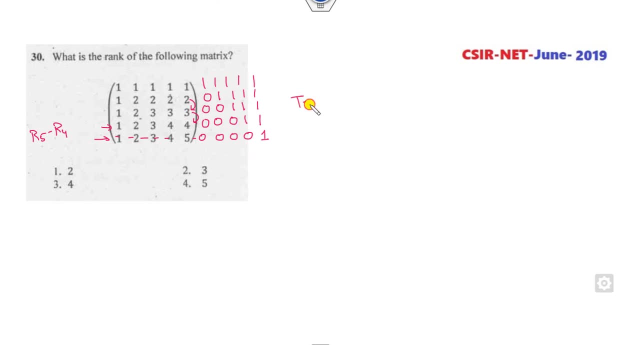 5 Eigen values, So product of them is my determinant is my 1.. Or otherwise, you can simply see It is a lower triangular, So that determinant will be here. So these are my 2 eigen values, So this is my 1.. 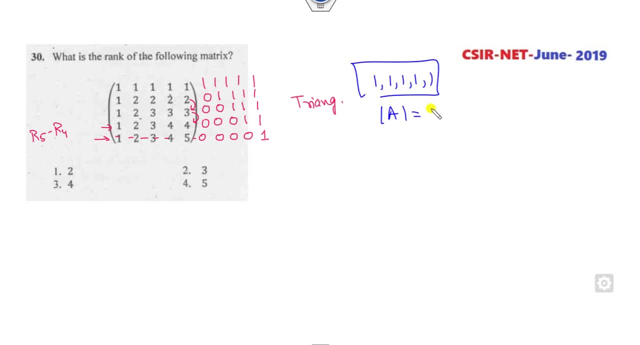 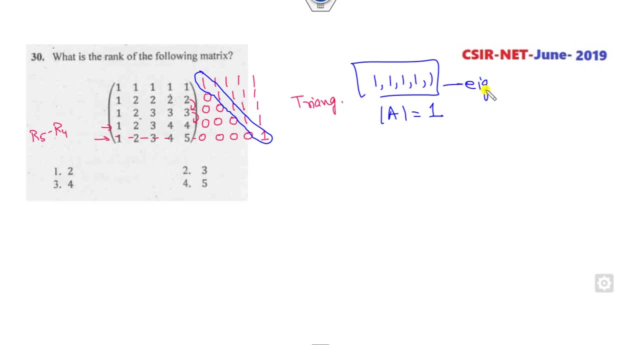 So these are my Eigen values Here, as you can see, is a lower triangular, So that determinant will be here. So these are my Eigen values, or you can simply say: So determinant is a non-0.. So it means the rank of them will be a 5 is the right ones. 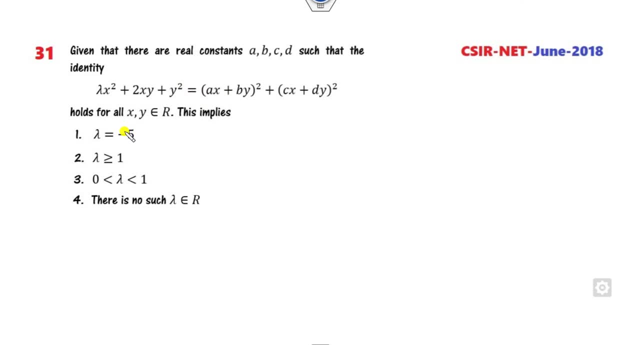 Consider here: A, B, C, D are the real constants. such, this condition holds for all pair of the x and y. then what is the value of the lambda? That is the very simple. you equate the coefficient on the both side. it will be a square plus b square. fine, now clearly. 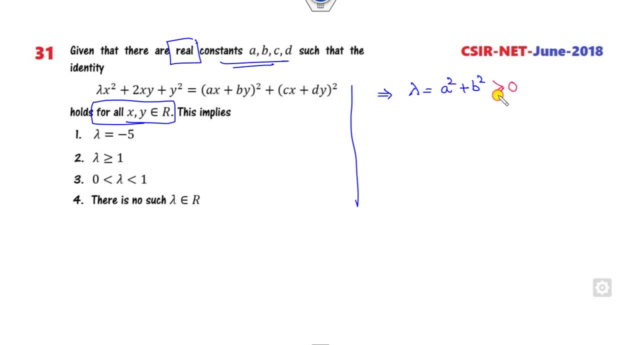 see, is a square plus b square is always be greater than 0 or equal to 0. fine, so first option is cancel out. a and b are my real numbers. so there is no such lambda exists. there is a cancel option. now it can be 0, it cannot be. now how you can check about the second and third. look at that. 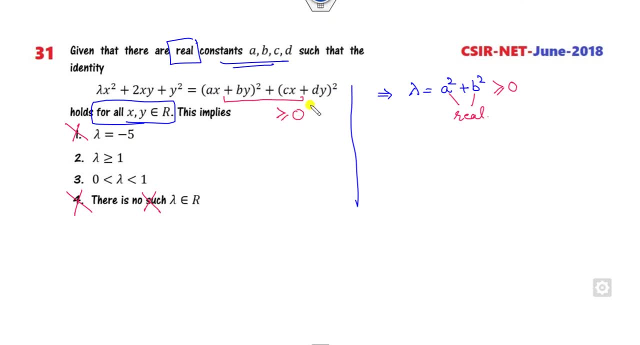 this option is greater than equal to 0. fine. another thing is: it is for all. so what is the meaning of that? the left hand side, this pair, is also be greater than 0 for all. the pair of the x, comma, y, remember the word is all. if it is for all, what is the meaning of that? it is a greater. 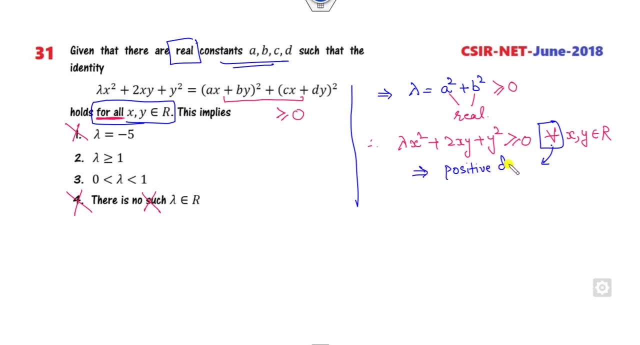 than 0. it means it is my positive definite. fine, because if it is there there exists some x, then it is not a positive definite. but he said, for all the x it means it is a positive definite. so once it is a positive definite we can write the matrix q as coefficient of the x square. 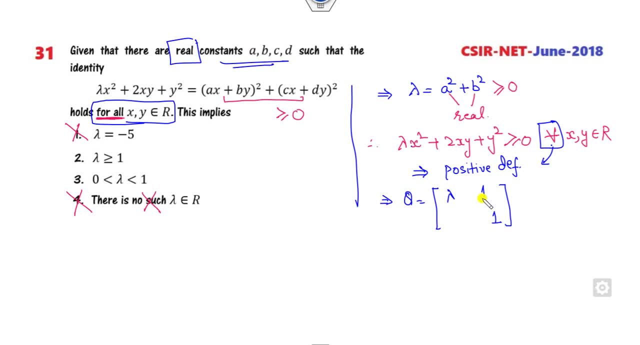 coefficient of the y square and it is a. it is always be the symmetric. so you can see the half of this and half of this. now, what is the property of the positive definite? the positive definite means the principal minors are always be greater than or equal to. 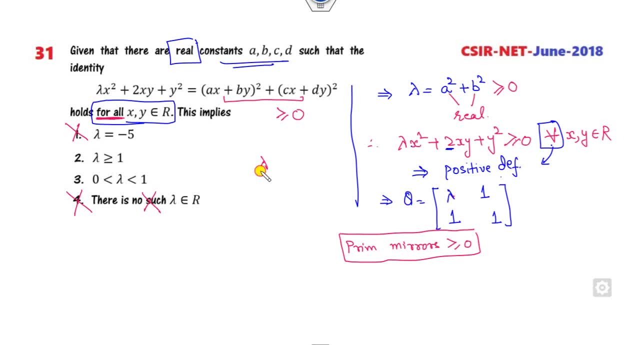 0. fine, because it is equality. so the first principal minor is lambda, which is greater than 0. second principal minor is the determinant of this. so lambda minus 1 is greater than equal to 0. so what is that? the first line say here, second line say here: so what is the? 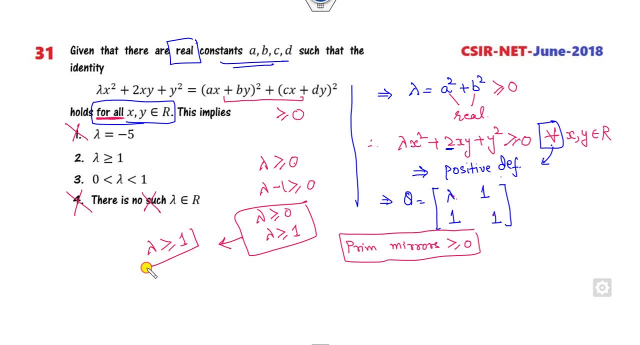 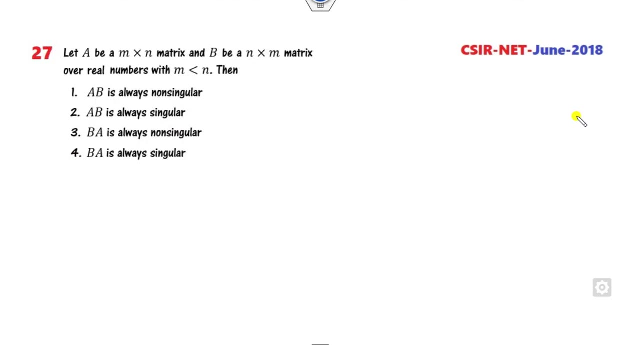 conclusion of these two cases. it means it is greater than equal to 1 is the right answer of this problem. so that is a simple, straightforward quadratic form here, remember the word is. so let us check the equation to see that boughtillon utilize to the stop at of the first key. 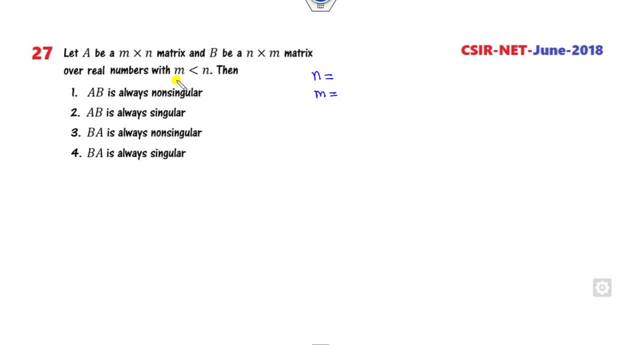 help. so that is the conclusion of this example. so we are straight forward. the whole tell us that is the shortcut. yeah, and then we have to65 the tense box. now come in and do the same thing here. this is the first grain of 0. prove: here it is ba non-singular and ba is a single. so what is that? this is my 1 cross 2. 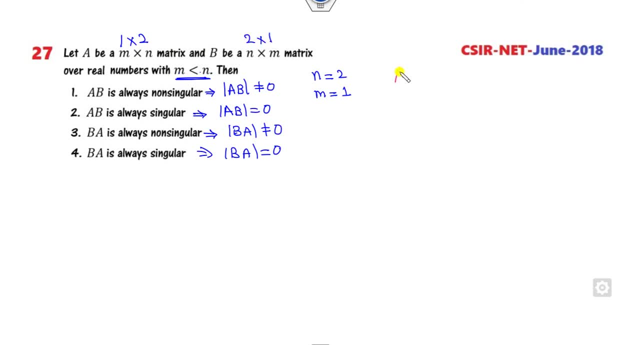 this is my 2 cross 1. so think about the. any example simplest way: 1 cross 2. fine, what is that? 2 cross 1, 1 comma 0. fine. now you can check about the ab. what is the ab? 1 0, 1, 0. so ab will be my. 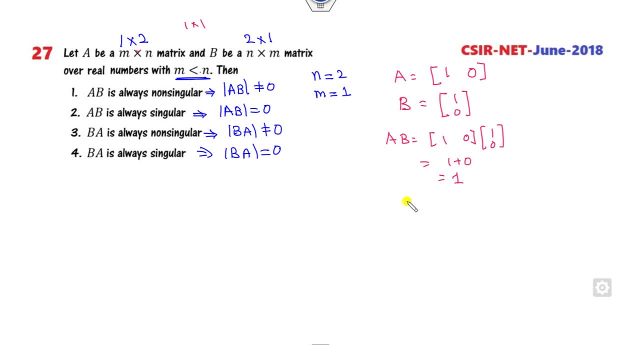 1 cross 1. if you multiply them, 1 plus 0 is 1, so what is that determinant of them is my non-zero, so he said it's a 0. this option cancelled. we can check also for the ba. what is my ba is 1: 0. 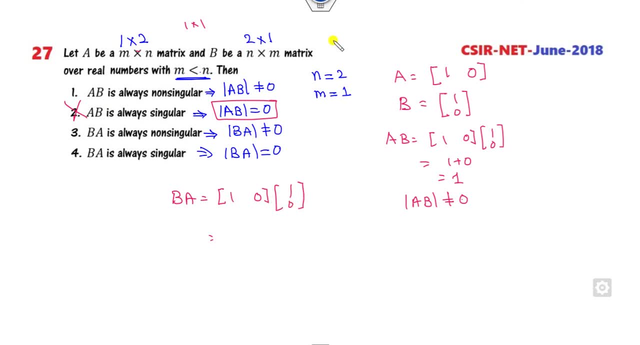 and 1, 0, so it's a 2 cross 2. so what is that? 1 first pair, 1 second pair, it's it's a, b firstly. sorry, it's a, b firstly. you have to write a, b, so b will be my 1, 0, a will be my 1 comma 0. so what is that? 1, 0, 0, 0. so what is that? determinant of the. 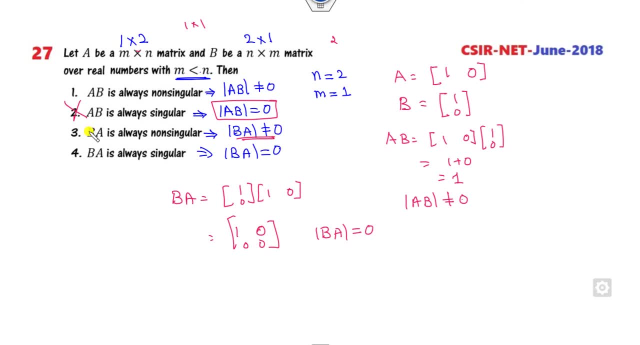 ba is a 0, but he said it's a non-zero, so this option also cancelled out. now how you can check about the ab, and here we can take the another example. i can copy this for here. so what do i can? i can take another value, say b, as reverse, say. 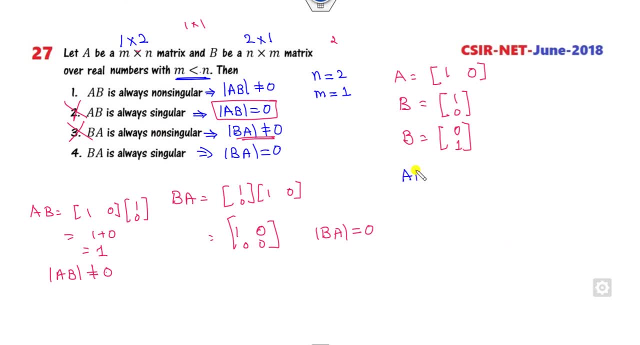 0, 1. fine, so then i can check about the ab: 1: 0 and 0: 1. so what is that? it's a 0 plus 0, it's a 0. so ab is a non-zero, is a cancelled out is the only right answer of this problem if you want to check. 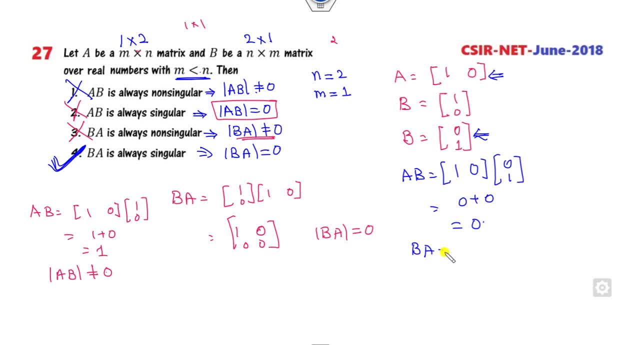 about this- is a, b. this is my a. if you want to check ba, it will be b, it will be a. so clearly say that: 0, 0, 1, 0. and what is the determinant of this? a, b is a, 0. so this property here satisfied, this property here satisfied, while the rest of the 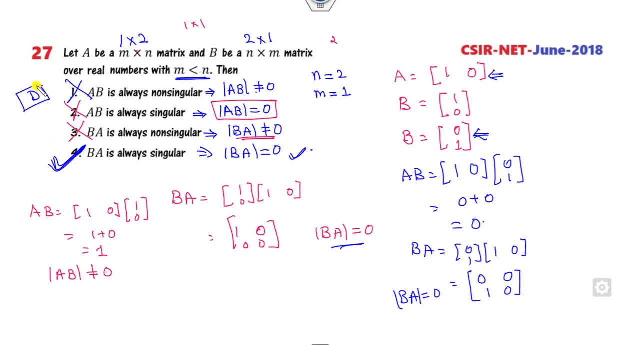 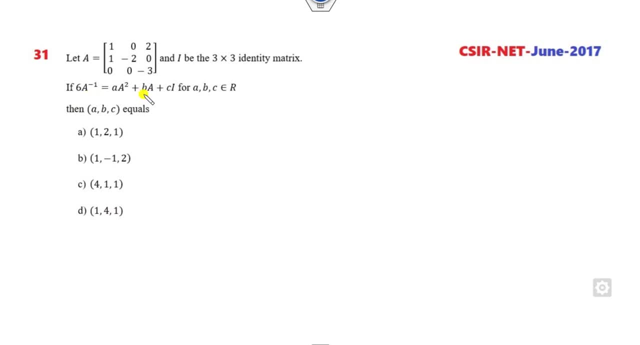 property cancel out. so the right answer is my d is the correct answer. okay, look for this one. a is my here, then okay, what is that? whenever you think about this equation, what is given? what is come in your mind? yes, that's a kelly hamilton theorem, so i can simply write this equation: 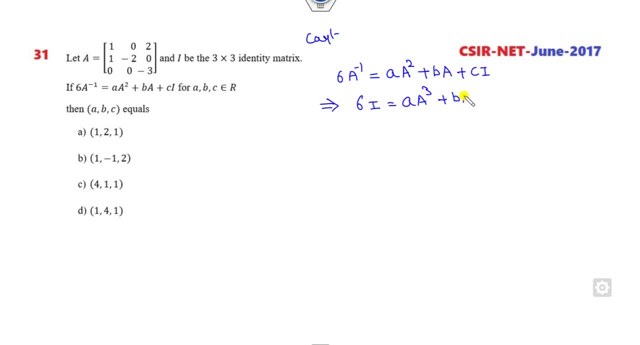 as 6. i is a cube plus b, a square plus 6 a. so if i say lambda is the eigenvalue of this, so this equation will give you plus b here, plus c minus 6, is equal to 0. fine, this is the meaning of this. 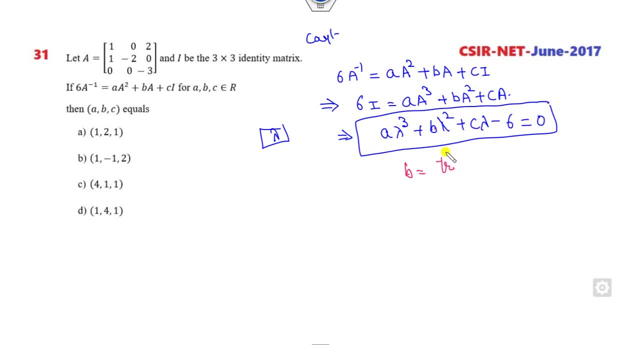 now, what is a, b, b is nothing but my trace. sorry, b is nothing but my sum of the root of this equation, root of equation number one. and we all knows what is the root of this eigenvalue sum of the root is here. what is given to you? that is nothing but my trace of the matrix. 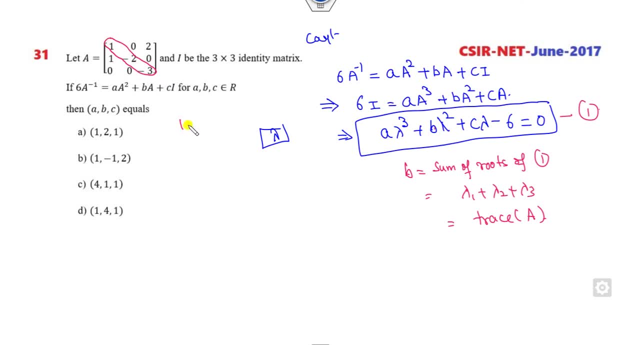 so what is the trace of this you can see? so it is 1 minus 2 minus 3. it is my minus 4, so sum of the root will be my minus b over a. fine, so what is the answer is minus b over a is my. 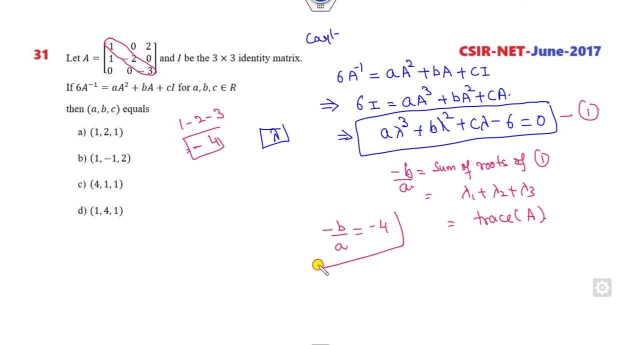 is my b over a or minus of 4, or you can see b is equal to 4a. so what is that? b is equal to 4a. not satisfied. b is equal to 4a. not satisfied. b is equal to 4a. not satisfied. b is equal to 4a. satisfied is the. 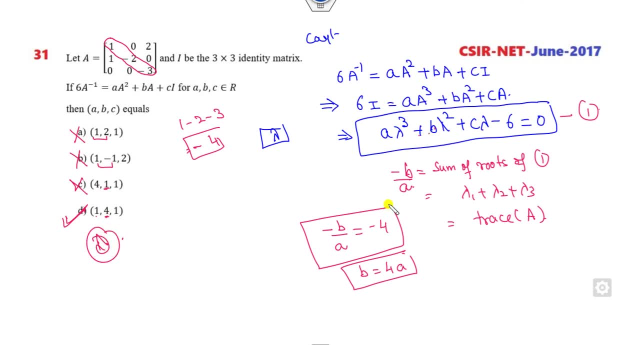 right answer of this problem. these are sum of the root minus b over a sum of the root is nothing but the trace trace is the sum of the diagonal length trace, so minus of the 4. so you can see b is equal to 4a. only this option, because a is 1, b is equal to 4, is satisfied. 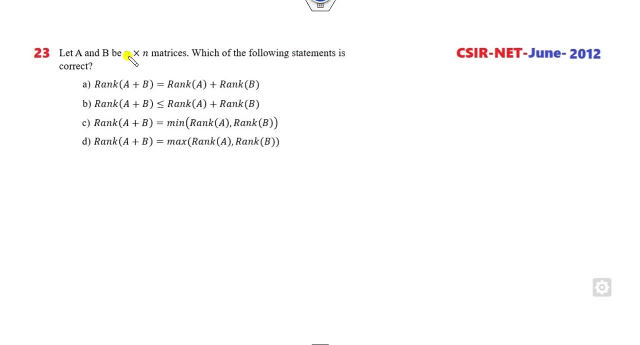 okay, again, this n cross n. you can think any of the a. so if i consider a is my 2 cross 2, b is also my 2 cross 2, fine, so think about any of there. i can simply take: a is my 1, 0, 0, 0. 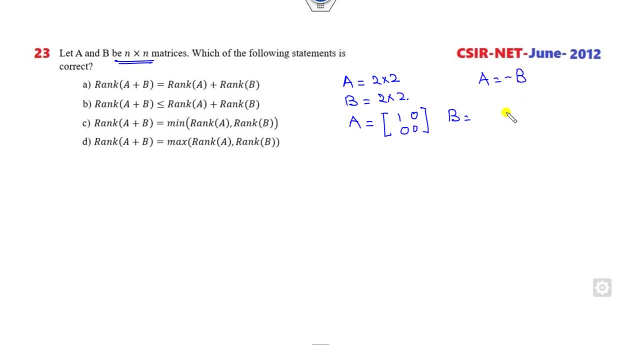 and b will be my. i can simply take: a is equal to minus b, so it is my here. so what is the rank of the a 1 rank of the b 1? what is the rank of the a plus b? so what is that? what is the happen of the a plus b? a plus b will be my. 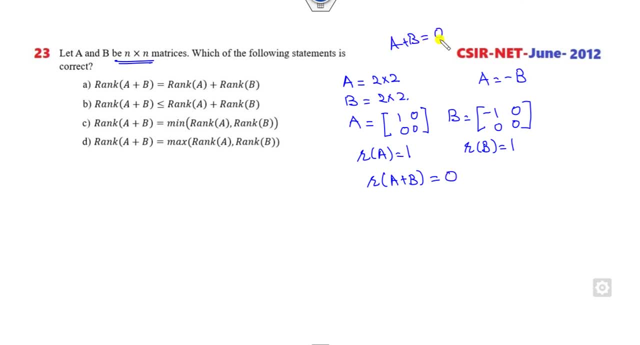 0 matrix, so the rank of this will be my 0. now check about that. this is a 0, a 1, 1 not satisfied. 0 less than 1 plus 1 satisfied. but this is a one counter example. third option: 0 is minimum of 1 comma. 1 zero is equal to 1 not satisfied. cancel again is a 1. 1 maximum is again. 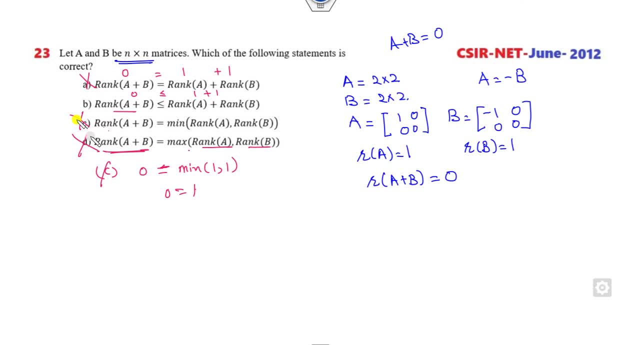 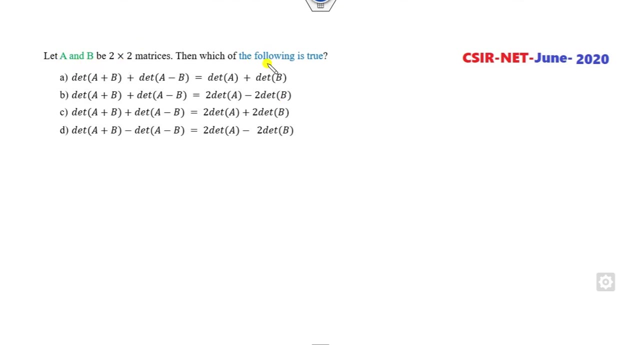 1, but left hand side is a 0, so not satisfied. the only right answer is my b is the correct answer. so you can see there is a very, very simple r there, once you think about this shortcut quick. so here a and b are the 2 cross 2, and here that is again very simple, because we need a minus b. 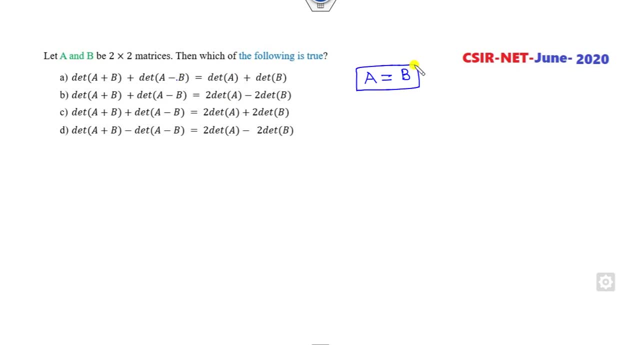 a plus b. firstly, we can think about: a is equal to b. is that 2 cross 2? i can simply take here, because it's a, 2 cross 2, either you can take i, i can simply take a is equal to, b is equal to i. 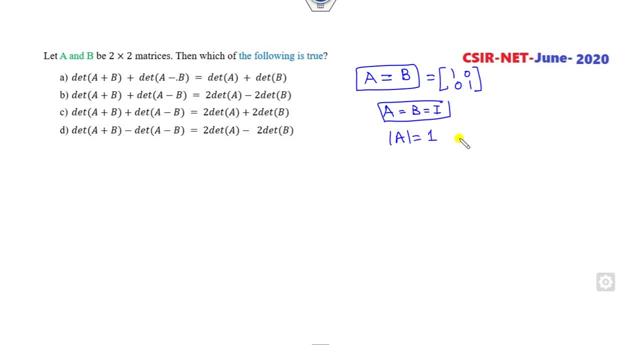 fine, so what is the determinant of a: 1. determinant of b: 1. so what is the first option? what is the determinant of 2a? so it is my 2 cross 2, so it is my 2 raised to power. 2. determinant of a, remember. 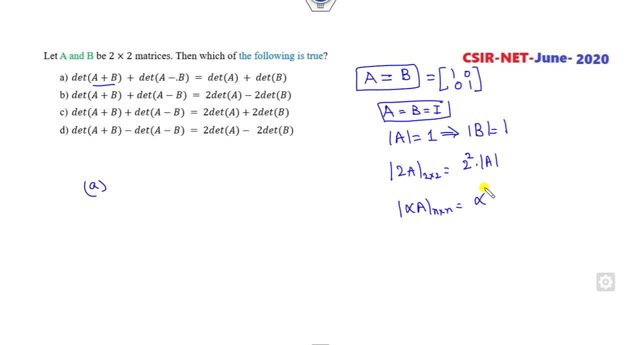 alpha of a, n cross. n is my alpha raised to power n determinant of a. so it is my 4, left hand side, 4 plus 0. this is 1 plus 1, not satisfied. this is my 4. this is 0, 2 minus 2, not satisfied 4. 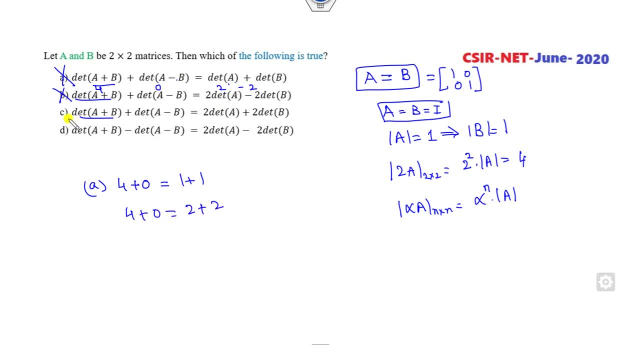 plus 0, 4, 2 plus 2 satisfied. but this is a one counter example. we have to discard this option as well. 4 minus 0, 2 minus 2, cancel out. so the right answer is only my. c is the right because here: 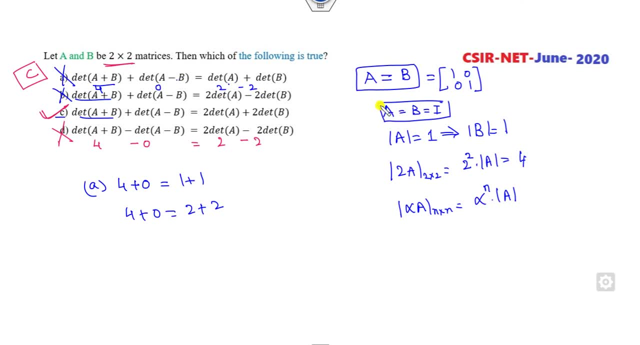 they are only talking about the 2 cross 2. you can think about any of the 2 cross 2 you may think about here as well, but that will take you a lot of the calculation. so i can simply take a and b as a. i. 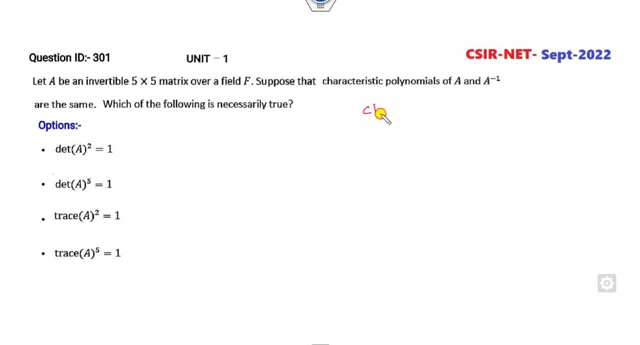 x. so now, what is the definition of the second criterion, fur yang k say. so what is number 8, k, k, k, k, ok, k, a is my 5 cross 5, such that characteristics polynomial of the a, characteristics polynomial of the a inverse are same. so what is the meaning of that? it means the eigenvalue of this matrix a and the 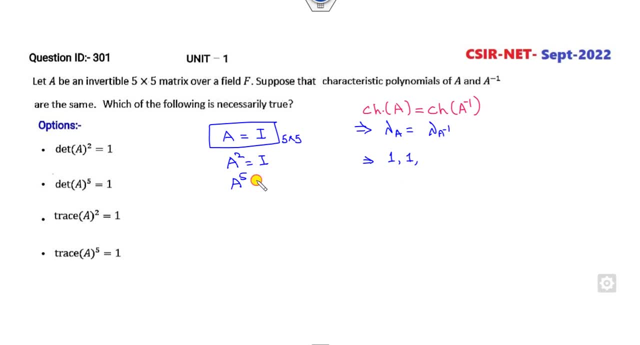 a square is also i. and what is the a5? it is also i. then what is the twice of the a square? so if it is a 5 cross 5, so this is my i, so twice of them will be my 5. but he said twice of the a square. 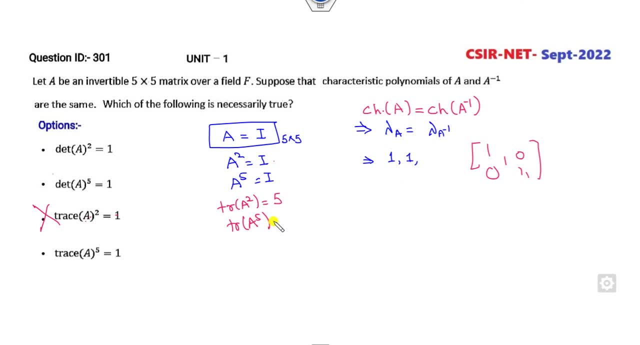 is 1 is a cancel out. twice of the a5 is again 5, so this option is also cancelled. what is the determinant of the a square? so it's only the diagonal entry 1, it's a 1. he said also 1, but we can't say it's a correct option because it's a counter example. determinant of the a5. 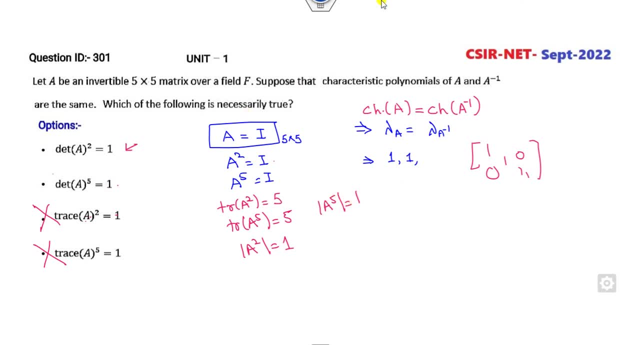 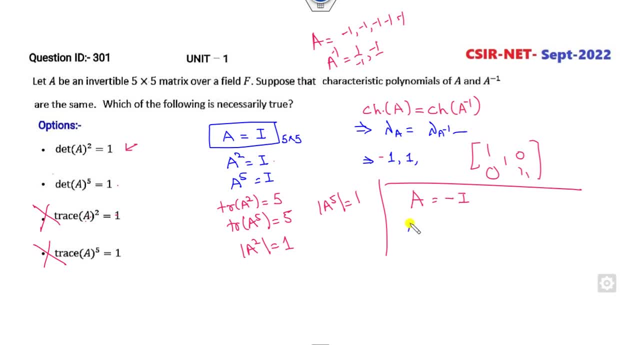 1 over minus 1. both are same, so they are the same. what is the a square is a plus i. what is the a raised to power, 5 minus of the i? what is the determinant of the a square 1? what is the determinant of the a5 minus 1? but he said determinant is plus 1. so based on this, 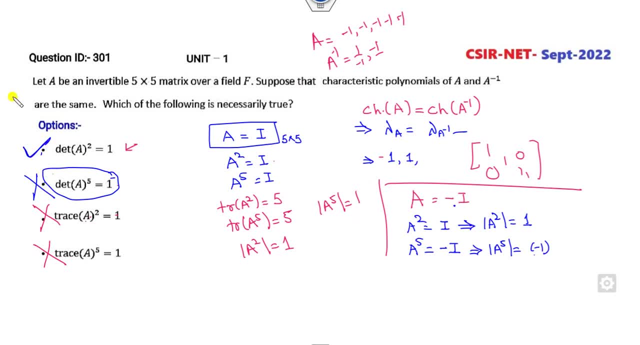 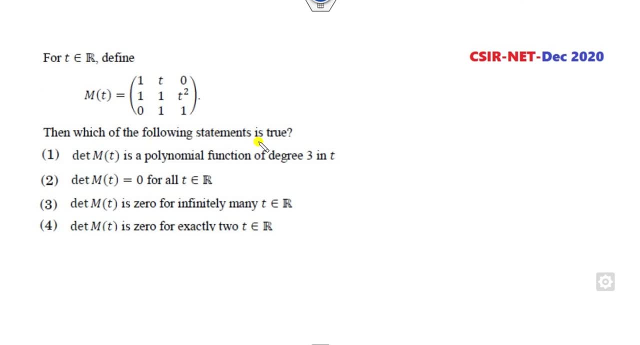 counter example. this is a cancel out, so only one option left. so that is my correct option, okay. next one is: which of the following statement is my true determinant? all they have the determinant. look at this option. this is 0 for all. the t belongs to the r. if i simply take t is my 0 for the easiest calculation. 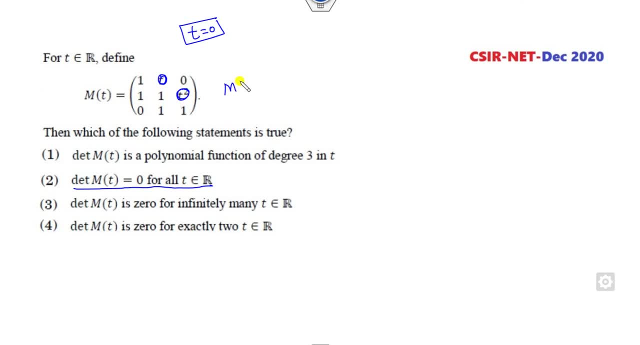 this value will be 0. this value will be 0. what is the determinant of this? it's a triangular matrix. it's a 1 which is non-zero. so this option is cancel out. fine, now look at that. determinant is a 0 for infinitely many, exactly 2, polynomial of degree 3. so what? i can expand them. what is that? 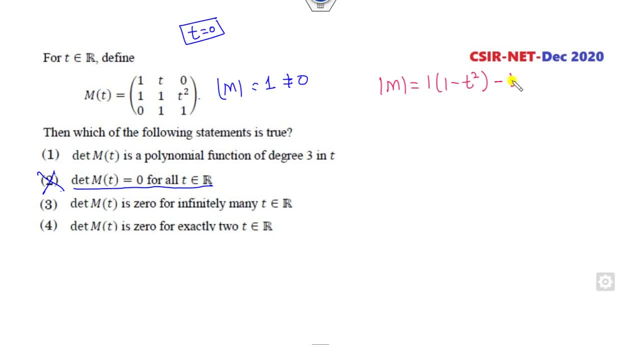 1 minus of t, square minus of t. 1 minus 0, so 1 minus t, square minus of t. so what is the degree of this polynomial? degrees my 2, but he said degree 3, cancel out. this is 0 for infinitely many t, that's. 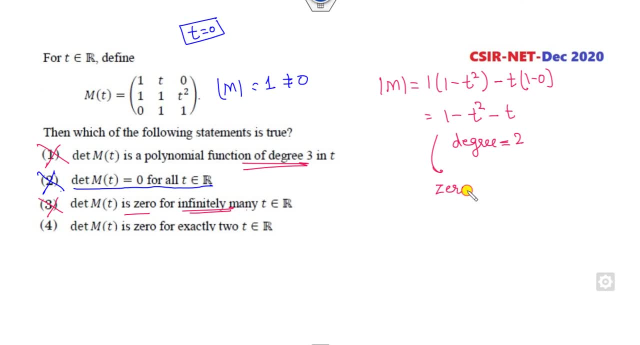 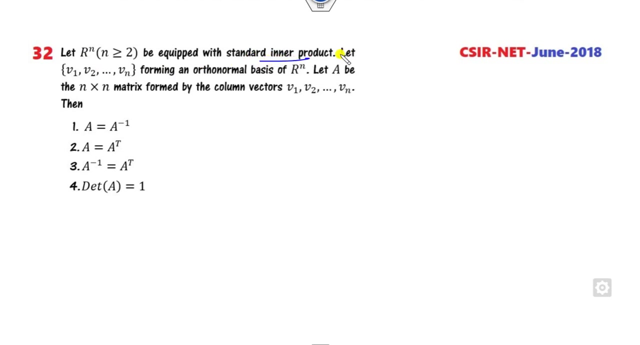 a wrong statement because this is 0 for exactly because it's a quadratic, so we can see exactly of the two roots of this t. so exactly, two values, the correct option. all the three are cancelled out. right option is the fourth option is the correct. okay, look at this one. r of n is my standard inner product. v1, v2 are my. 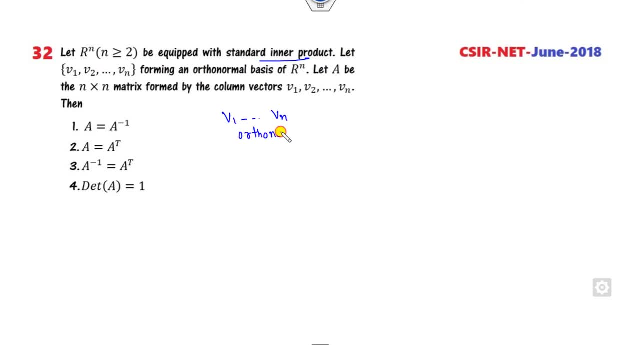 orthonormal is my orthonormal fine a. again it's a n cross n. so firstly i can take as a 2 cross 2. so it means my v1 and v2 are my orthonormal fine. then the matrix a is formed by v1 and v2. okay, what is orthonormal is that is v1 dot. v2 will be 0. 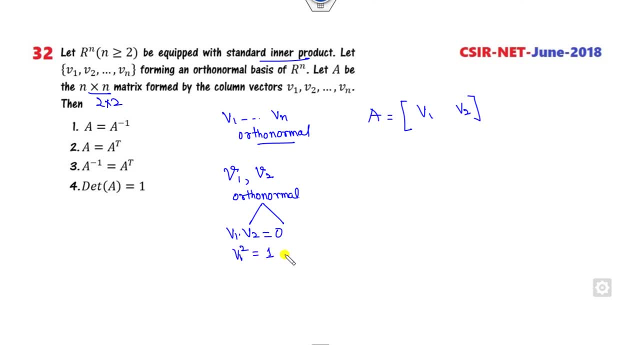 and v1 square will be 1. fine, like of this matrix if i simply say 1 0, 0 minus 1, so clearly say that if v11 is my 1 square of them is 1, square of 1 is 1 dot product will be 0. now, if you consider the 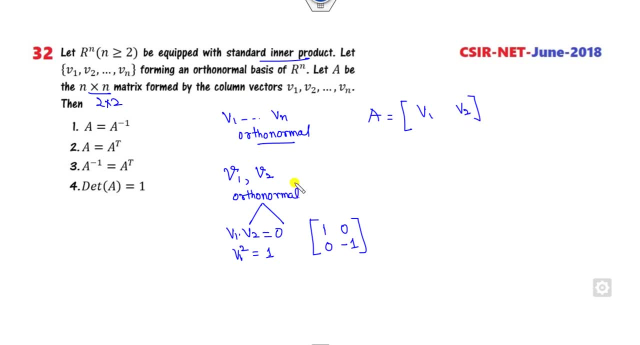 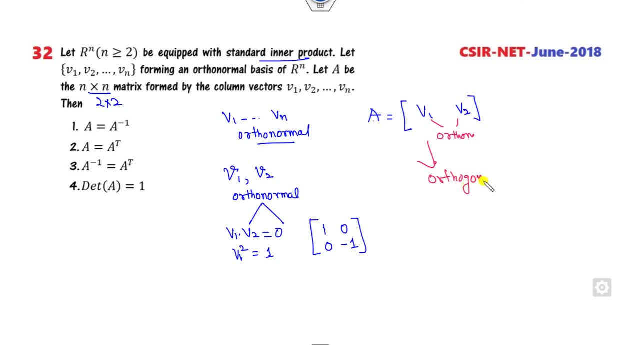 what is the matrix corresponding to them? this is my orthogonal matrix. you can easily construct by using the graham smith process. so once a is my orthogonal matrix, what is the meaning of that? a into a transpose is my i. that's a simple property. so a into a transpose is the i is a. 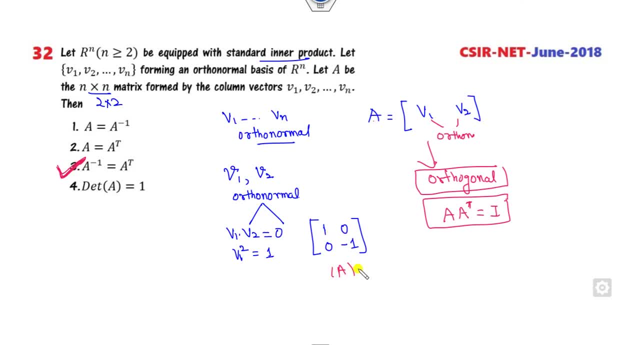 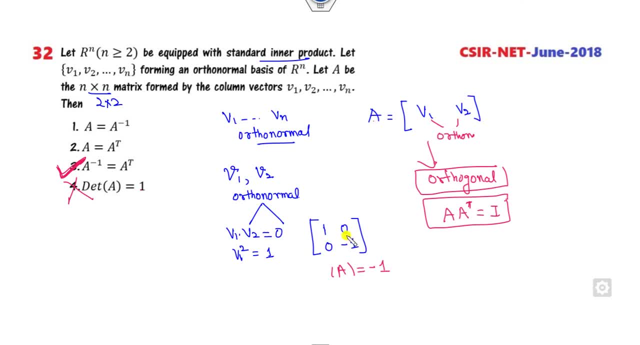 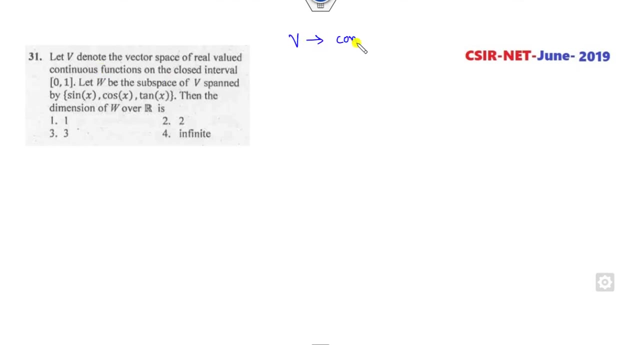 orthogonal property not satisfied. a and a inverse are same. in this case is also same, but it is not satisfied the orthogonal property. so the right answer is only my. c is the correct answer. okay, v is the vector space of the continuous function over the clause into a, 0 comma 1. 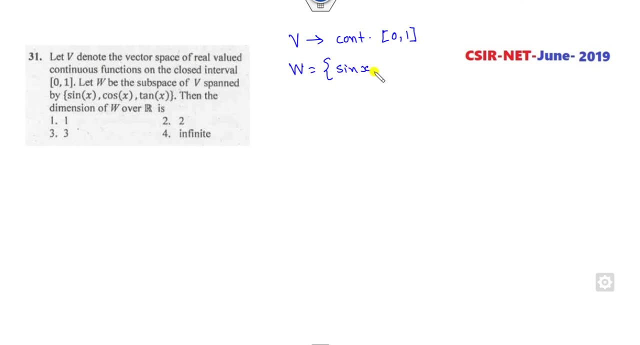 w is my subspace of the sine x, cos x and the tan x. fine, then your target is to find the dimension. what is the meaning of the dimension? you have to find the number of the linearly independent vectors. how you find the number of the linear independent vectors in case of the function? we will check about the. 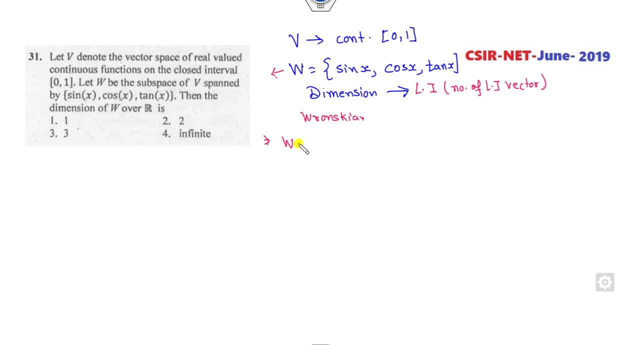 ronskian. fine, so what is the ronskian if you have the three different function, like f1, f2, f3, so we can take the first derivative, you can take the second derivative. fine, this is my 3 cross 3, if it. 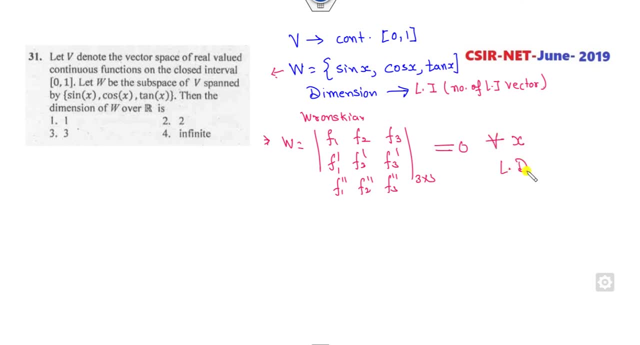 is 0 for all x, then we call as the ld. if it is a non-zero for all x, we call as the li. fine, so once we know the li, then we call as the li dimensions. so since, firstly, we can take the derivative sine x, cos x, tan x. so what is the derivative? is sin x, cos x, tan x, sin x, cos x, tan x. so what is the derivative? 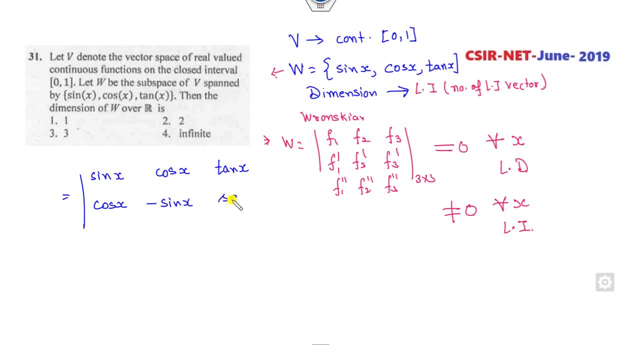 cos x minus sin x, tan. secant square x minus sin x minus cos x 2. secant x into secant x, tan x, so secant square tan x. so now we all know, in order to check for the linear independent, if wronskian 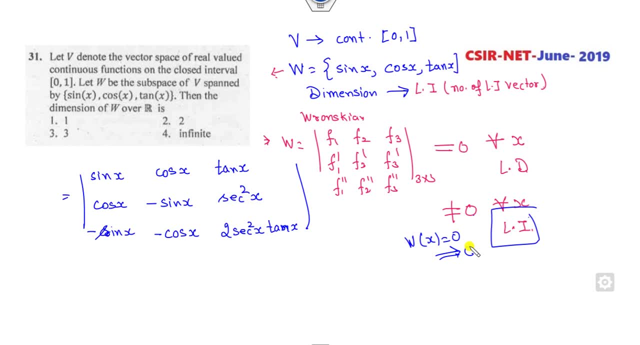 is 0, then it will be 0 for all the domain. it will be 0 for all the domain, otherwise it will not be it. so if you take any of the pair, so you can choose any of the value of the x, if we prove that that value- the wronskian- is non-zero, it means it is non-zero for the clause interval of this. 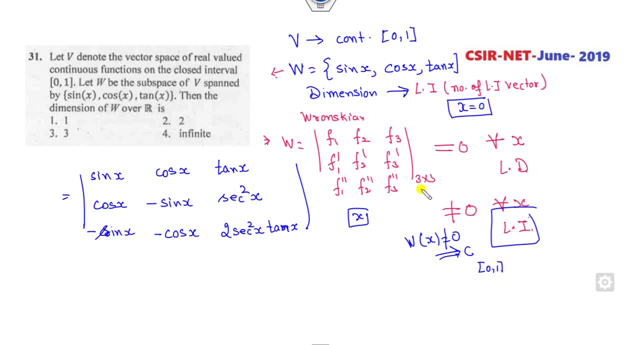 the easiest way we can to to cast x is equal to 0, but you can see when x is 0, the function 0, 1, 0. so it is not be there. so you can choose any of the value, the easiest way you can choose, as a. 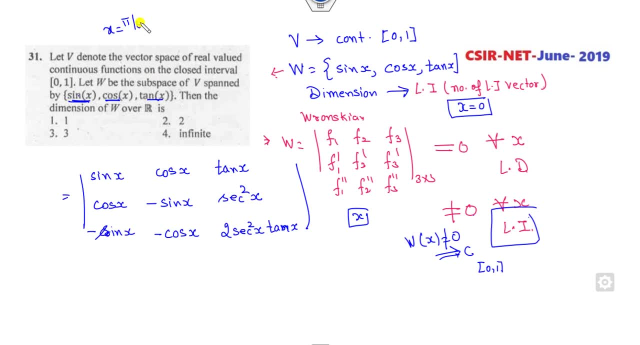 pi by 6, so, but it will give you as a root of this easier way you can choose as a pi by 6, so, but it will give you as a root of this easier way you can take as a pi by 4, so tan pi by 4 is 1 and here. so what is that? this is 1 by root, 2. 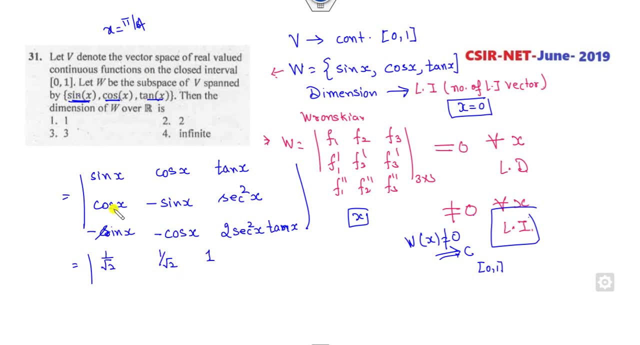 it is 1 by root 2. it is 1. cos is 1 by root 2. this is minus 1 by root 2. secant square is 2. sin is minus 1 by root 2. it is minus 1 by root 2. it is a tan: 45 is 1, secant square is my 2, so 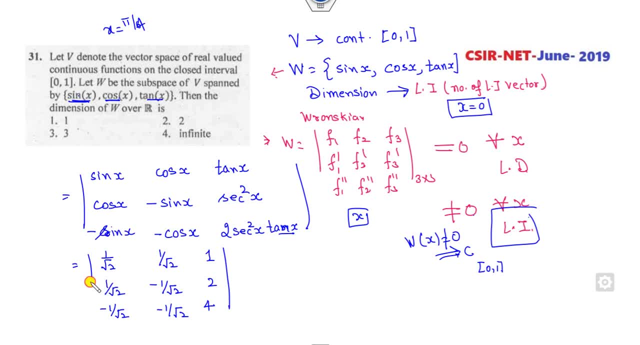 2 into 2 is my 4. now how you can solve the determinant? you can simply add them. this give you a two times. this give you a six times. you can subtract them. this will give you a zero. this will give you two times. this will give you one. then you can make them. you can subtract this pair. this will: 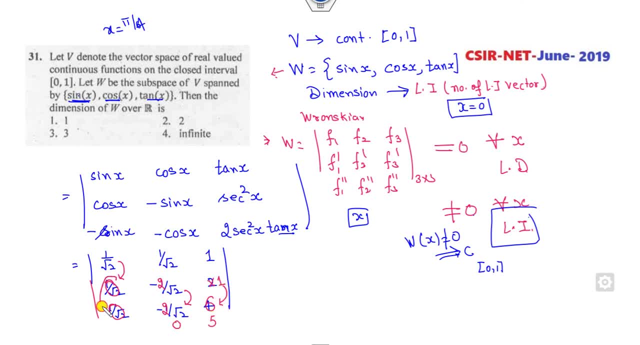 give a zero, this will give you a 5, so these three values will be zero. so what is the product of them? 1 by root 2 minus 2 by root 2, and of 5, which is my non-zero. so it means these three vectors are my. 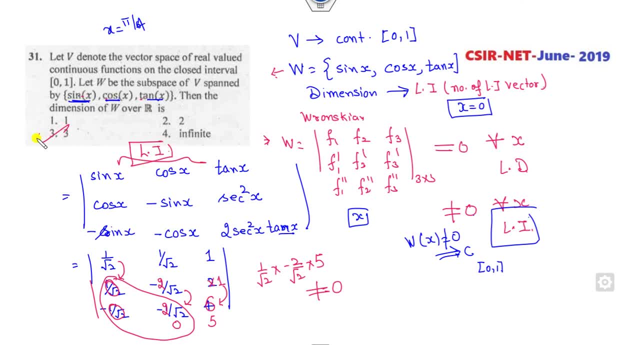 li. So what is the dimension of this? There are the 3 vectors, So dimension is my 3 is the right answer. So that is a very simple. You can check about the li. If li is not be there, then 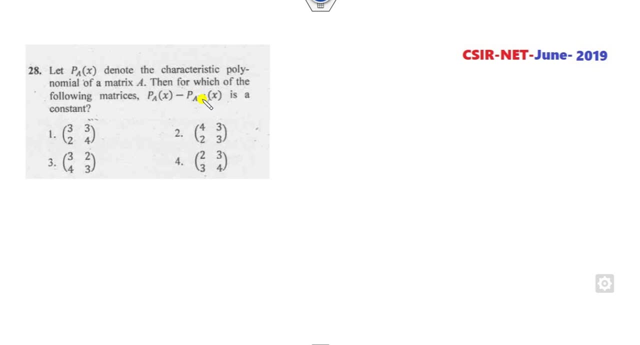 dimension will be less than of the 3.. Okay, look at this. another concept: P of a is the characteristics polynomial of a. Then P of a inverse is the characteristics polynomial of the a inverse. which of the following is a constant? What is the characteristics polynomial? 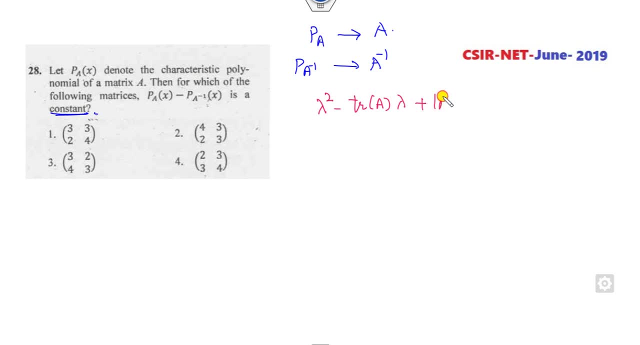 This is my characteristics polynomial of the matrix a. Fine. What is the characteristics polynomial of the? a inverse? This is the characteristics polynomial of the? a inverse. Fine, Now what the statement said. if you take the difference, it will be constant. When it will? 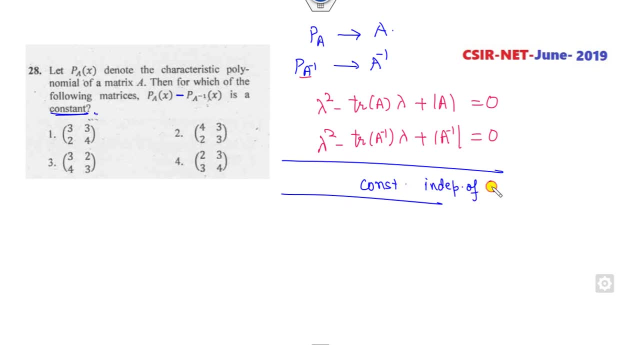 be constant When it is independent of the variable lambda. So when it will be here? So only When both the values, when both the values are same, then only if you subtract them, it will be cancelled out and then it will be left as here, as a constant. So what is the meaning of that? 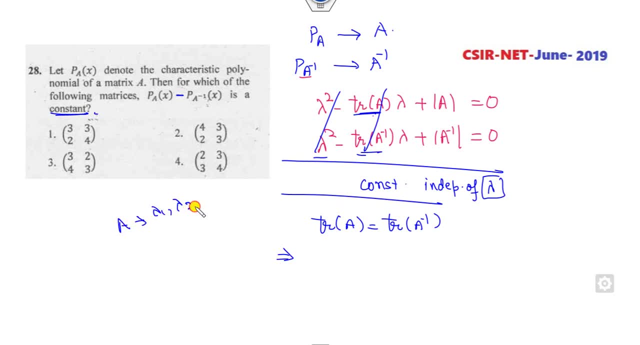 What is that? If I consider a has the eigenvalue lambda 1 and lambda 2, what is the? a inverse eigenvalue, 1 over this, 1 over this. So what is the trace of this? This is What is the trace of. 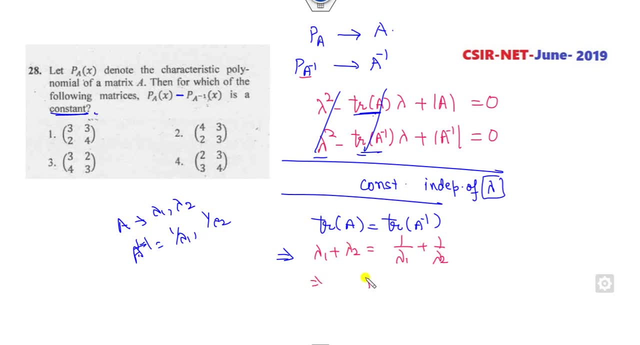 this Here. So if you take the LCM, what is the meaning of that? This will be 1.. So what is the meaning of that? Or you can say what is that? If a has the eigenvalue, this product of them is 1.. That means determinant will be 1.. So check about the 4. 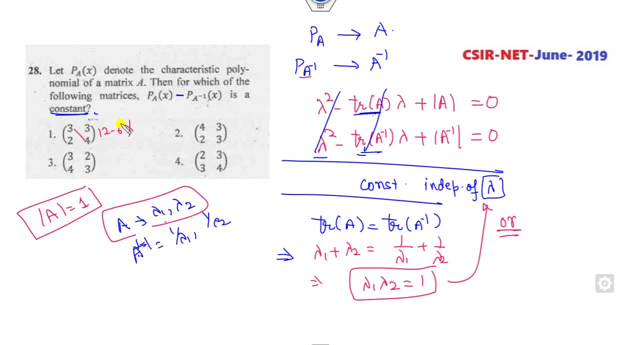 option whose determinant will be 1.. So 12 minus 6, not 1.. 9 minus 8, 1.. Correct option: 12 minus 6, not 1.. 8 minus 9 is a minus 1, but we need a plus 1.. So the right answer is only the third option. 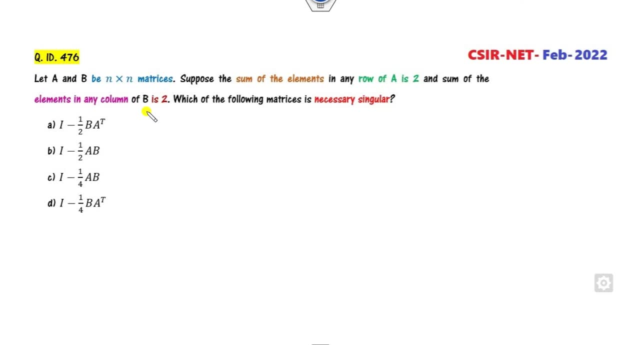 is the correct answer. Okay, Look about this. another question. So again, it is given to you as a is n cross n, So I can simply take 2 cross 2.. Fine, a is my 2 cross 2, such that the sum of the each element of the row 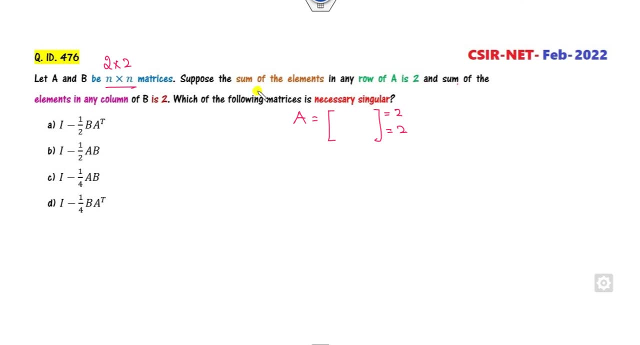 is my 2.. This is my 2 and sum of the. if I take as a b sum of the each column values, sum of the each column is my 2.. So firstly check whether this property is satisfied for the i: 1,, 0,, 0,, 1.. No, Sum is not. 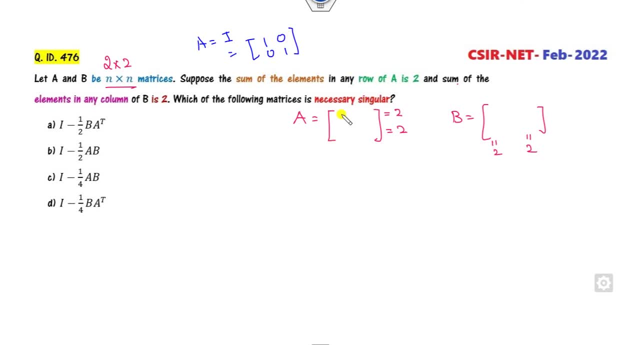 be a 2.. So what you can do, I can simply take, is a 0,, 2, sum is 2, 1, 1 satisfied, Okay, And we need a transpose also. So if I take same as, So ultimately what I can think is here: Fine, Now. 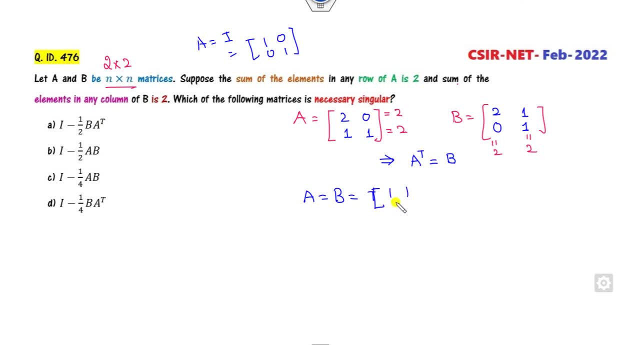 one simplest way is: you can simply take as 1, 1, 1, 1.. Column sum, row sum are same. Now what is the eigenvalue of this? What is the eigenvalue of this matrix? So clearly say that rank is 0. So 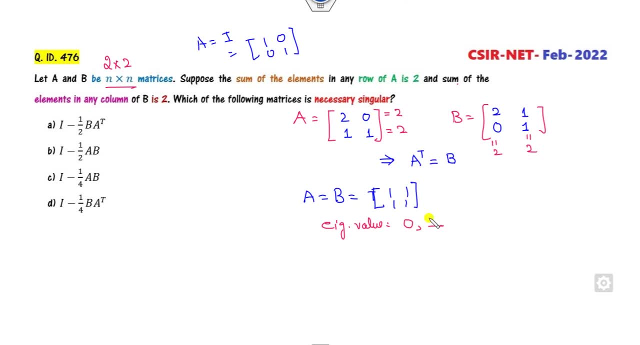 one eigenvalue is 0. The sum of the eigenvalue is my 2. So other value is my 2.. Fine, So a has the eigenvalue 0, a has eigenvalue 2.. What is that transpose? We all know that transpose has the. 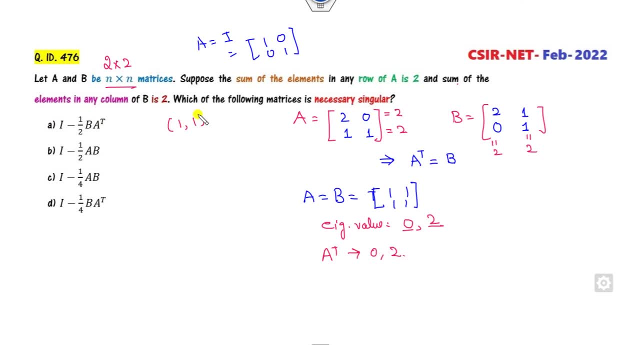 same eigenvalue. Fine, What is the eigenvalue of d Is 1, 1.. What is the eigenvalue of d? a is equal to b, So this is what is the b of a. transpose is b square. So eigenvalue of this is my b. What is the eigenvalue of the b? square 0, 4.. So now, 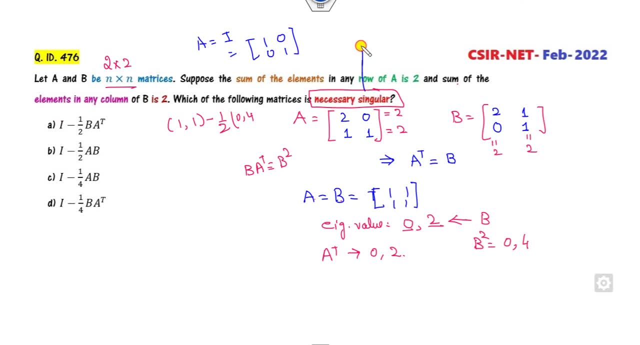 your target is to prove which one of them is a necessary singular Singular means. determinant of this answer will be 0, or at least one of the eigenvalue is my 0.. Fine, So these are the pair. So clearly say that if you take 1 minus 0 and 1 minus 2, none of the eigenvalue is 0. So first option: 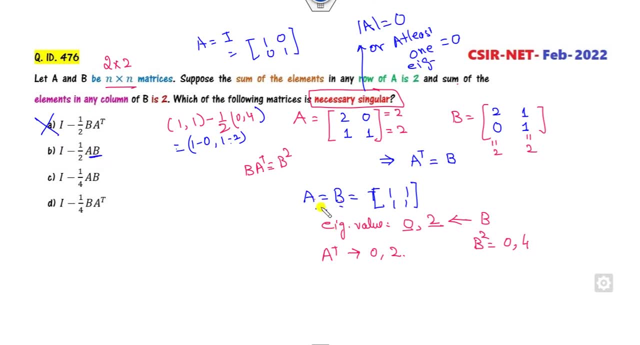 is cancelled. Same for here. What is the ab? ab is nothing but the b square, So none of the eigenvalue is 0.. Look at this one: 1, 1.. What is the eigenvalue of the ab? ab is nothing but my b. 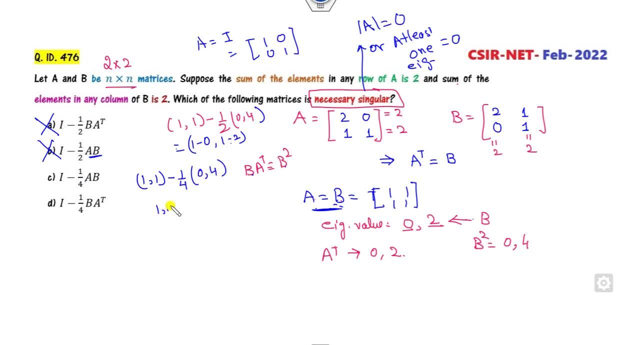 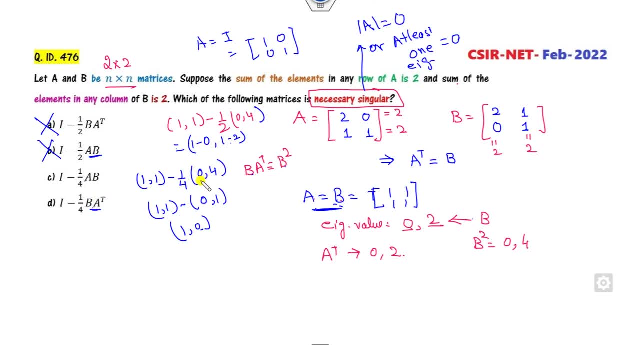 counter example: We can check over the b a transpose. This is again a b square. So out of these two options, we will check about that. So this first example. that is enough to discard for the first two options. Now how we can check for the other options. So I can look about this. 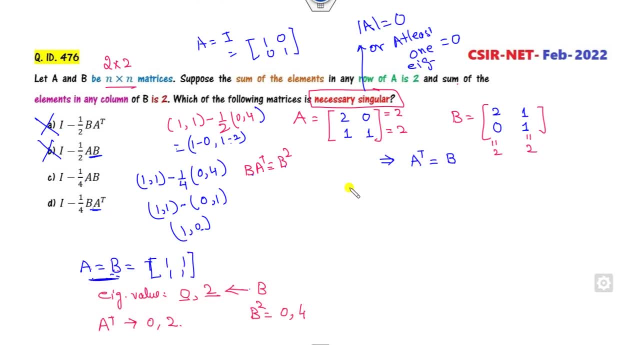 example. So a transpose is nothing but b. So what is that? This pair is my 1 minus half b square. What is the eigenvalue of the b? Eigenvalue of the b is my 2, 1.. What is the eigenvalue of the? 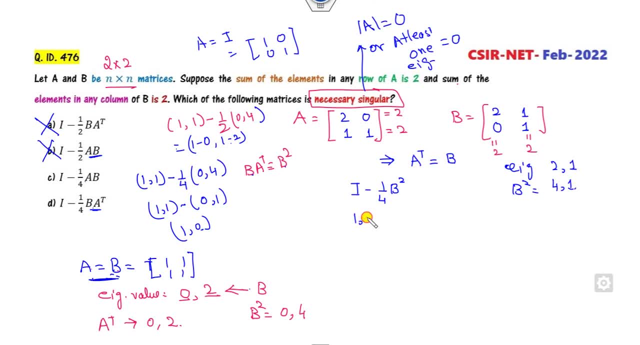 b square 4, 1.. So if I substitute here, these are the eigenvalue of the 1, 1.. Eigenvalue of this is 4, 1.. So it is 1 minus 1, 1 minus 1 by 4. It is still 0.. So we cannot discard them. 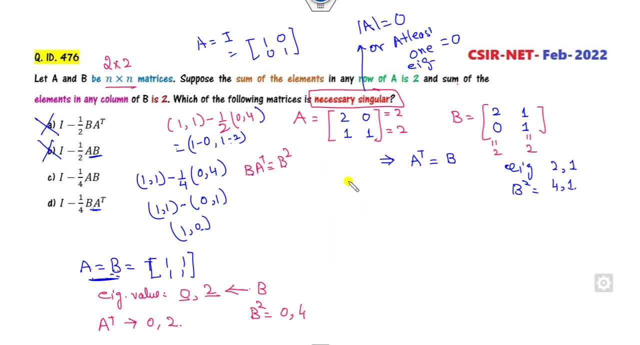 So we will check about the a b. If I a and this, what is the a b? So it is my 4, it is my 2, it is my 2 and it is my 2.. How you can find the eigenvalue? 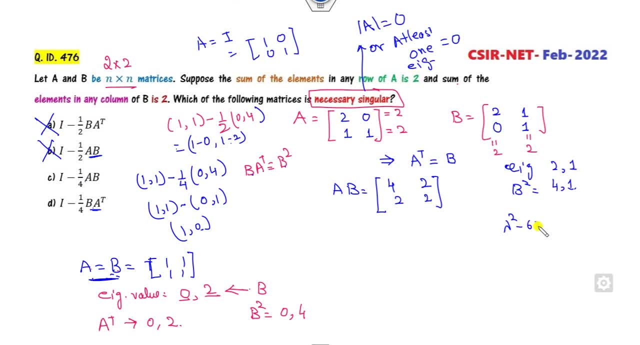 You can find this here. This is 6, 8 minus 4.. So this is the plus minus of here. So otherwise I can check about the determinant of this matrix. What is that? i minus 4 a, b. So 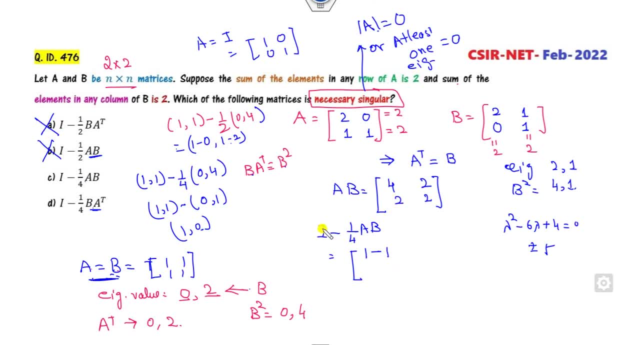 1 minus 1.. This is second component- is 0.. So 0 minus half, 1 by 4 of a b. 0 minus 1 by 4 of a b half. This is 1 minus. 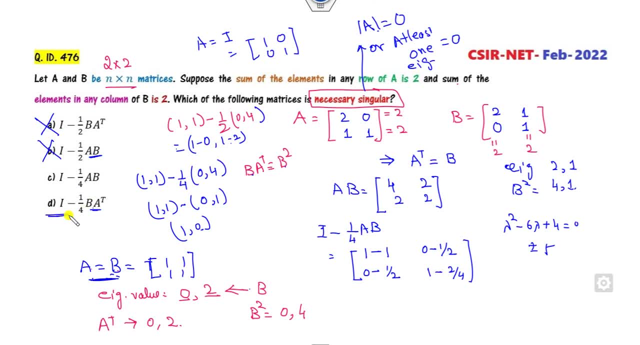 2 by 4.. So this is my matrix of this. What is the determinant of this? This is a 0.. So this will be 0.. This is a non-zero, So it is 1 by 4, which is a non-zero. So for the singular, 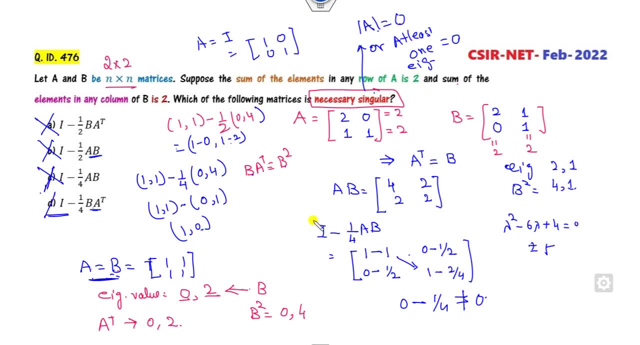 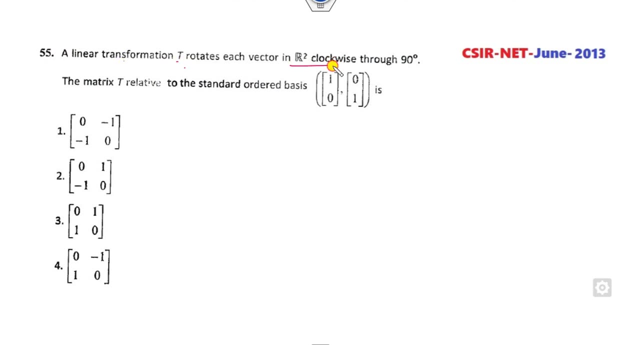 this matrix must be 0. So this option is. this option is cancelled. I have taken a b, So the only rest option is d is the right answer. Okay, look at the linear transformation. Rotate clockwise through the 90 degree, then off this. That is very simple. What is the 1, 0? You? 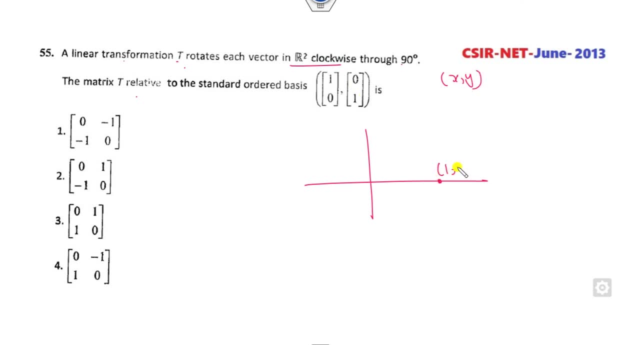 can think about the x- y pair. This is my 1, 0 pair. 0, 1 is my here. Now you have to rotate through the clockwise. This is my clockwise: 90 degree. This point, if I call this, is my a. 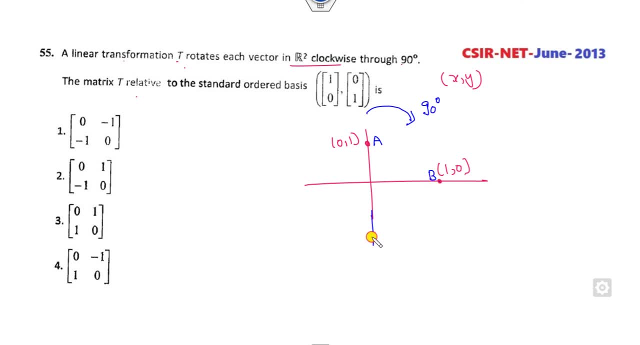 this is my b, So this point b will be my here. This is b dash and a will be my here. I call as a a dash. So what is the coordinate of the a dash? This point on this axis? it will be 1, 0.. What is the coordinate of the b On this y axis? x component is 0,. 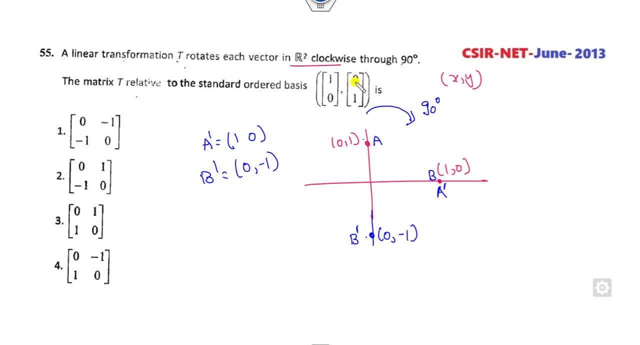 y axis is minus 1.. Fine, So what is the answer? So this map: 1, 0 will map to the 0, minus 1.. 0, 1 will map to the 1, 0 is the right answer. You can see. only this option is there. 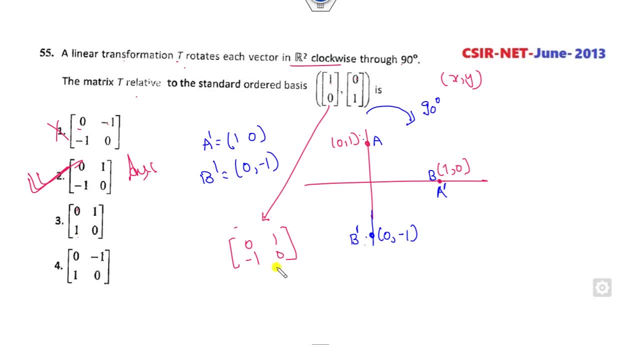 0, minus 1.. It is a minus 1.. Cancel out: 0, 1, but we need a 0, minus 1.. 0, 1, but we need a minus 1 is the wrong answer. Remember whenever you are talking about the linear transformation. 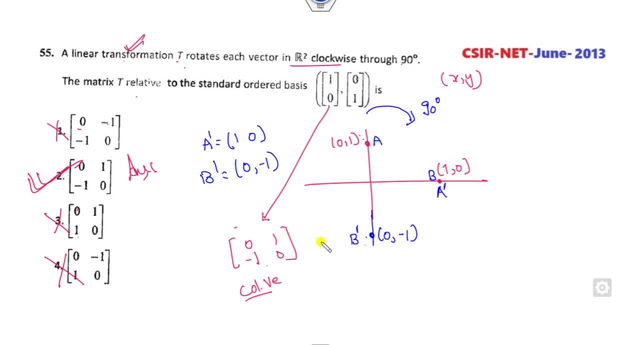 vectors are always written in the column vector. If you return this vector as a row matrix, then you can see this option is correct. but that is wrong. Always return the matrix in the column wise. So the right answer is: my b is the correct option. 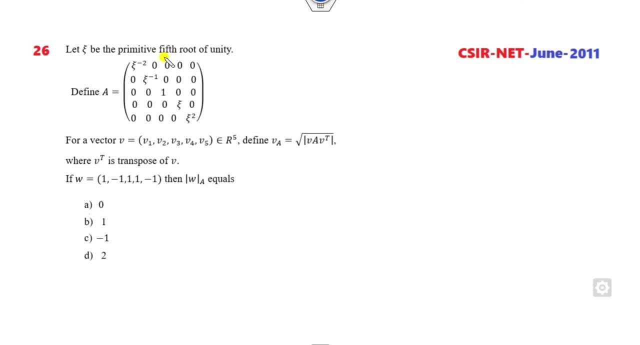 Okay, What is that? This is the primitive root of the unity. Omega raised to power. 5 is my 1.. Fine, Okay, V is my here. This is some certain matrix V of here is this V. a v transpose: Fine, So clearly say: 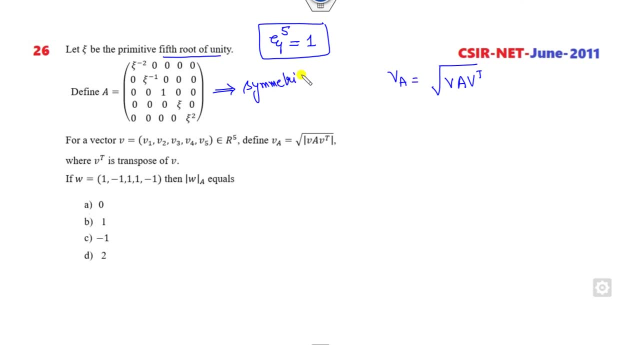 this is my symmetric matrix. Fine, Then, for the particular pair of the w. what is the value of this, of here? So what is that? This is nothing but my here. Fine, Now, what is the shortcut matrix Otherwise? 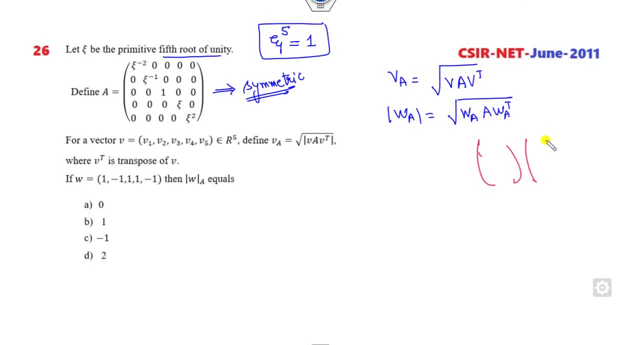 what you can do. You can write as a matrix a. You can write that transpose as 1, minus 1, 1, 1, and then you can multiply them. but there is no need How you can multiply them, Think about. 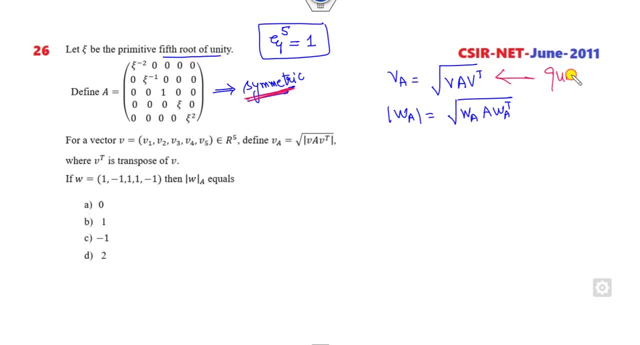 that This is matrix. What is that? This is my quadratic nature. Once this is matrix, it is a quadratic, So it is always be the quadratic form. So how you can multiply them is a quadratic form. When you multiply them, what will be the nature? The nature will be. this is my 1, 1.. So you can. 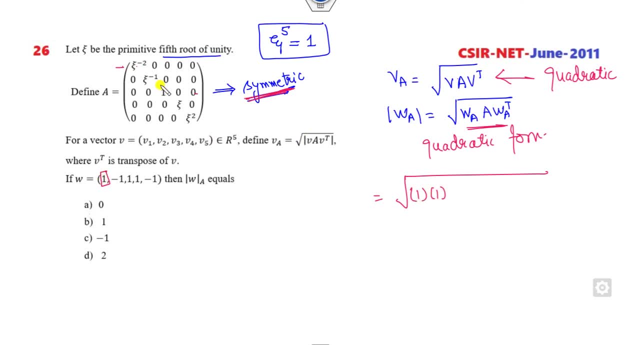 pair. first pair, 1 into 1.. That is, 1 into 1 of x i square Fine. Second is a 0.. So rest of the all are 0.. This is my a 2, 2.. So second element and again the second element. So this is my. 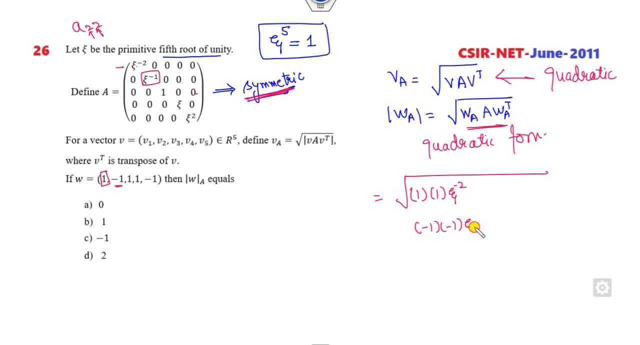 minus 1,, minus 1 of x. i minus Like here if I say this number is my 1 or say 4.. So what is that? If you multiply them, it will be a 1, 4.. The first pair: 1.. Fourth pair will be 1.. That is the. 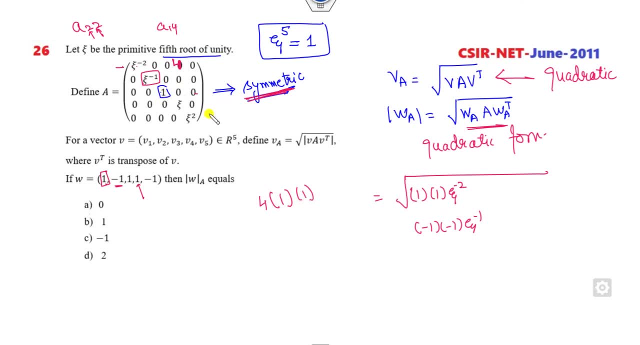 meaning of this. Similarly, the third pair is a 3, 3.. So 1.. Third pair is my square of this: 1, a 3, 3.. Fourth pair is x- i. Fourth pair, a 4, 4.. 1, 1.. Fifth pair is minus 1, minus 1 of x i. 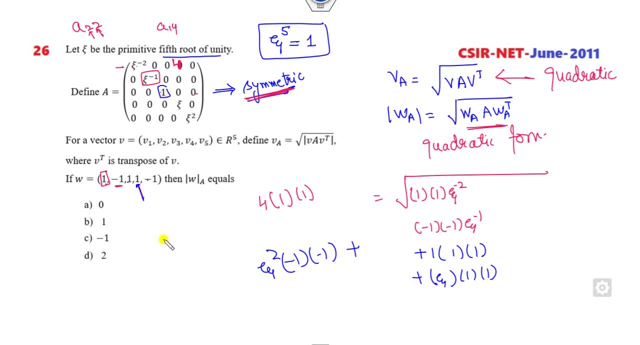 square. So what is the answer of this? This is my, so what is the answer? is: x i raise to power 2, x i raised to power minus 1, 1, x, i, x, i square. So what is the meaning of that? If you simplify, 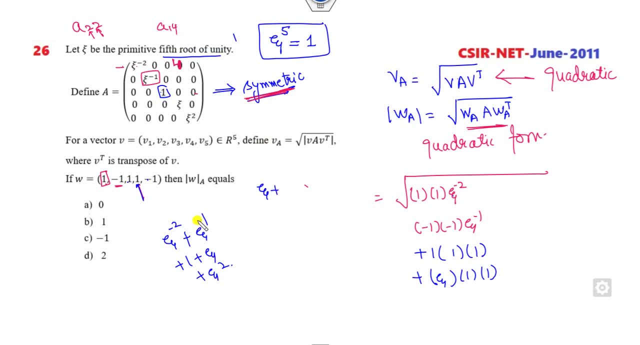 them. if you take the LCM, it will give you: or x i raised to power, 5 is 1.. So what is that? It is x i cube, x i square. 1 x i, x, i square. What is that? The sum of the primitive fifth root of the. 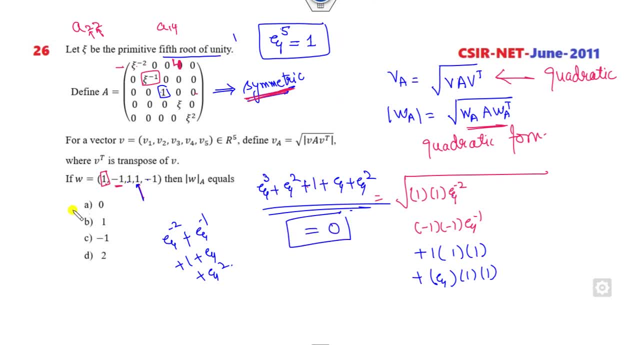 unity is always be the 0. So what is the right answer of this 0? square root of 0 is my 0. is the right answer of this: Sum of the primitive root is 0, product is my 1.. This is again the. 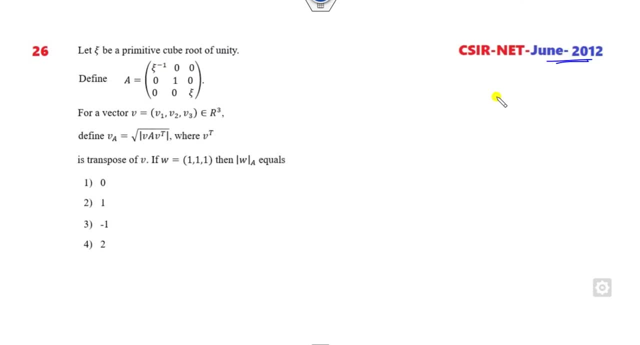 same: This is in the year 2012 and this is the year 2011.. Again, it is a primitive cube, root of the unity. So it is my 1.. Again, this is Smithwick and this is my quantity. Fine, So what is the? 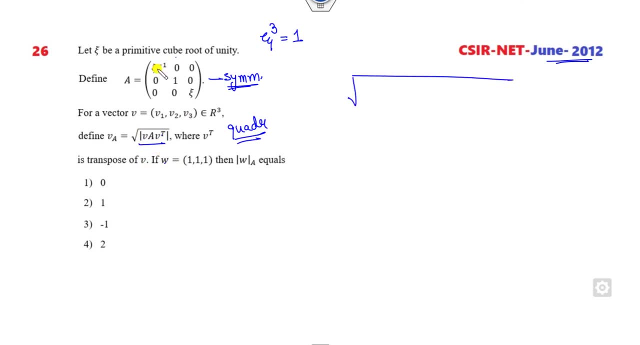 answer of the w of this. It is my root of the a 1, 1.. So first element is repeated two times. It is my quantity. So what is the answer of the w of this? It is my root of a 1, 1.. So first, 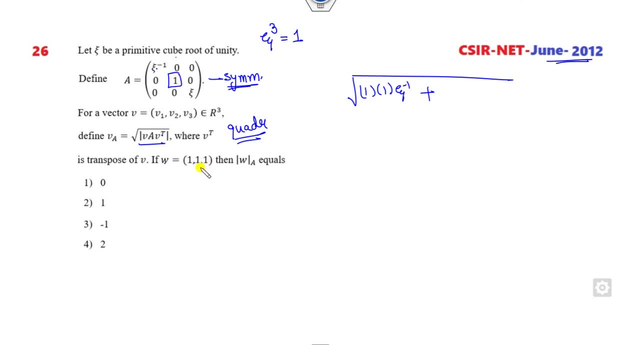 element is repeated two times. This is my a- 2, 2.. So second element repeated two times of 1 plus a 3, 3, two times of this. So what is that? This is x i raised to power minus 1,. 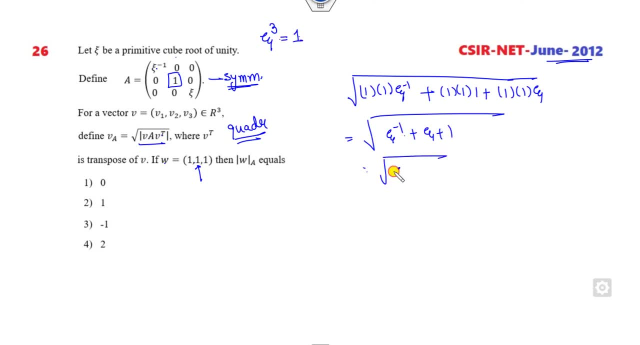 x i 1.. x i cube is 1.. So x i minus 1 is x i square. So what is that? This is sum of the cube, root of the unity, That is my 0.. So again, answer is 0 is the. 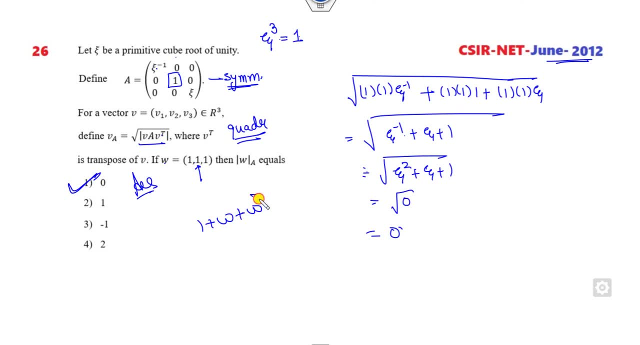 right answer, Because we all know, if omega is a cube root of unity, this value will be 0.. Omega cube is my 1.. Or you can simply see: I can write this number as of this manner also. Fine, So. 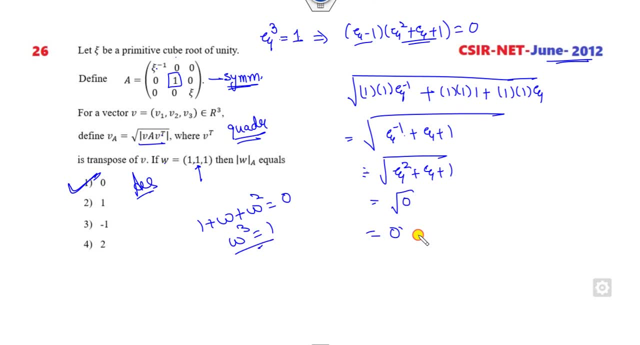 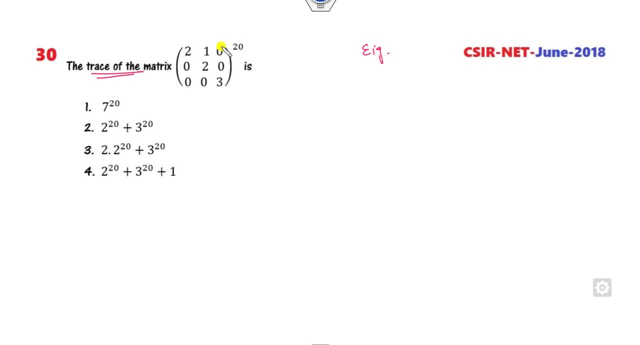 1 is a cube root of unity. This must be 0. So it is the right answer of this problem. Okay, Now you have to find the trace, So we will look about the eigenvalue. So firstly, we will check about the eigenvalue of this. What is the eigenvalue of this? 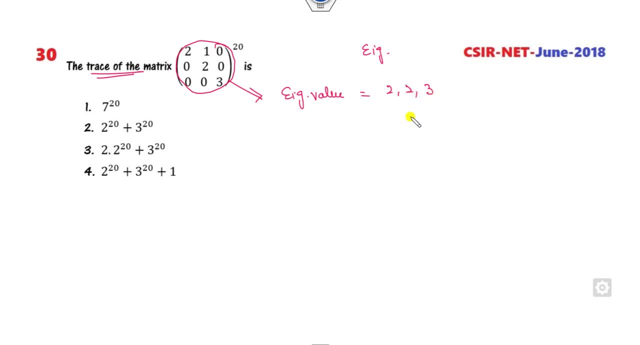 This matrix Eigenvalues are 2,, 2 and 3.. Then what is the eigenvalue of this matrix? 2 raised to power 20,, 2 raised to power 20,, 3 raised to power 20.. Why, If a has the eigenvalue? 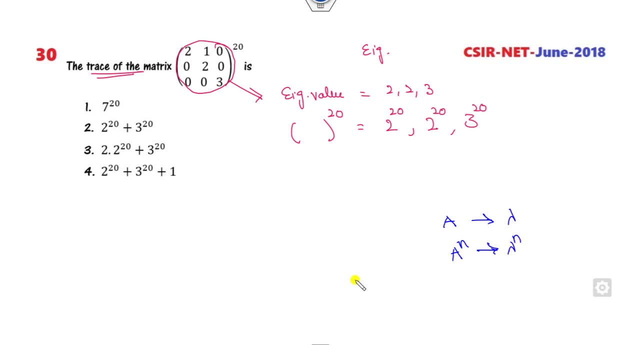 lambda a raised to power n has the eigenvalues here. Then what is the trace of this matrix? You can simply add them. So this is the right answer. So you can write as: 2 into 2 raised to power 20 plus 3 into 2 raised to power 20 is the right answer. So this option. 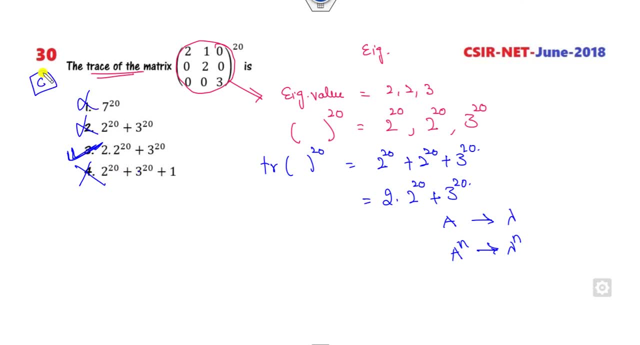 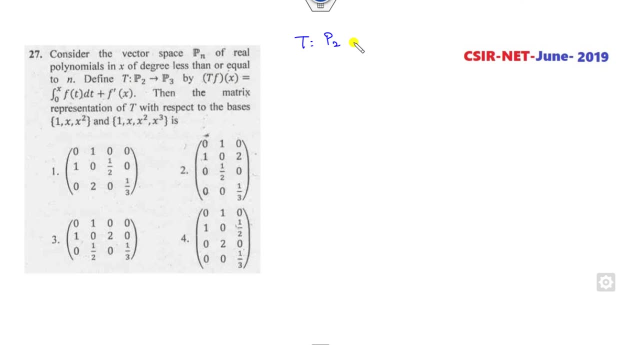 cancel This, cancel Only the C is the right answer of the problem. Okay, T is the mapping from P2 to P3 defined by integration: 0, F, dt plus F. dash, Fine, Then the matrix associated with this matrix is P3.. So this is 4 cross 3.. This is 4 cross 3.. Sorry, 3 cross 4,, 3 cross 4,. 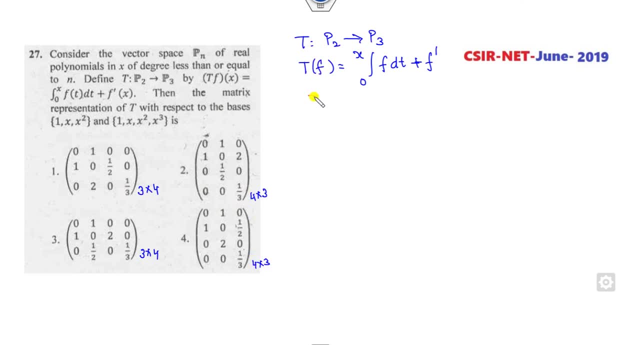 4 cross 3,, 4 cross 3.. Then what will be the matrix size? That is very simple. What is the size is, If I call this is a dimension n, this has the dimension m. Then the matrix. 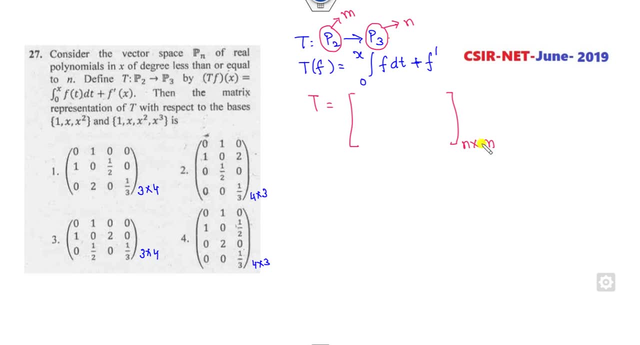 is always be the range multiplied by core domain here. So what is the dimension of the P3?? P3 is a polynomial of degree less than 0.. 4, equal to n. So what is the dimension of this? Less than or equal to 3.. So the dimension? 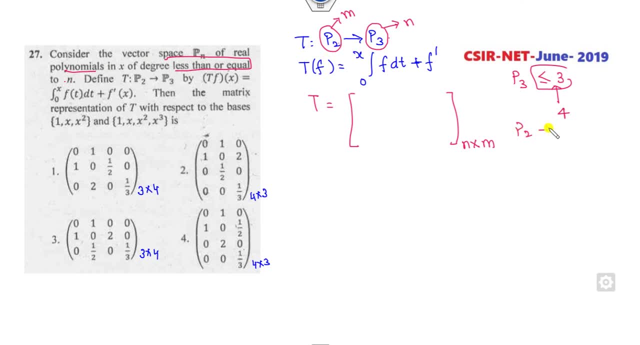 of this will be my 4. Dimension of the P2 will be my 3. So this matrix will be my 4 cross 3.. So first option, third option, cancel. Fine, Now look over there, We can take any. 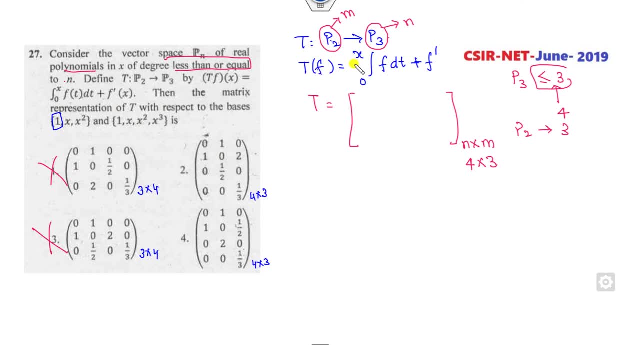 of the basis from the P2.. That is a 1.. If I substitute here what is the integration of the 1 dx? What is the derivative is 0. So it is x. So if I consider the basis of, 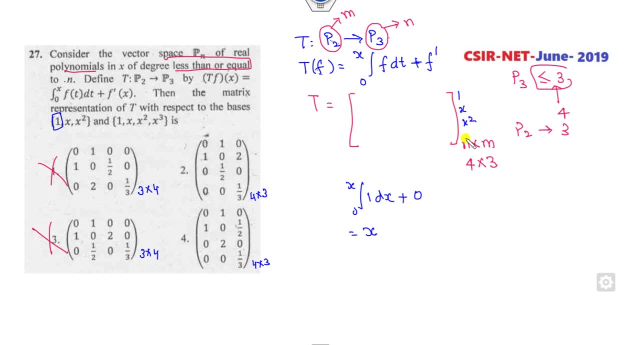 the 4, what is the derivative is 0.. So it is x. So if I consider the basis of the 4 cross So 1 x x, square, x, cube, This is my x. So that is a second. So second value. 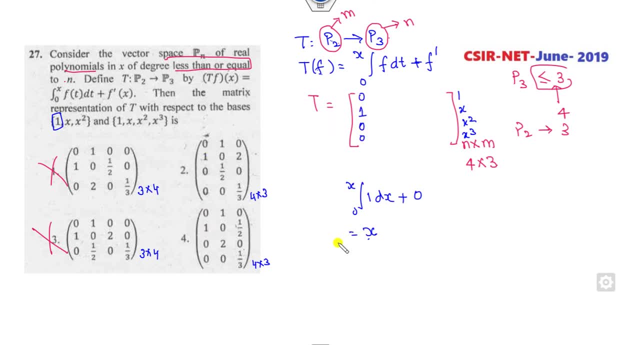 will be 1.. Rest all are my 0.. So first column satisfied. If I take the second basis as a x, then it is x of dx plus f dash There is a 1.. So integration is x square by 2 minus. 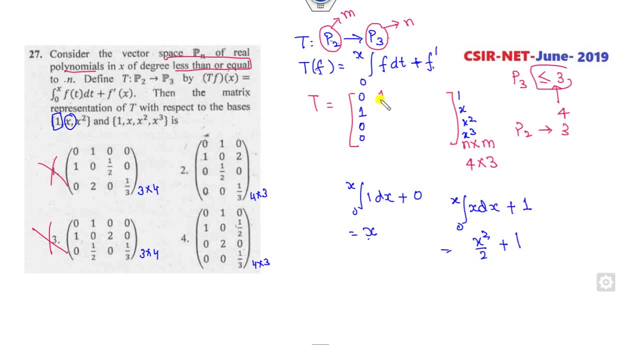 0 plus 1.. So you can see, 1 is a constant, So 1 is a constant x square. So this is my half. This is 0.. This is 0.. So this pair is satisfied. So this pair is satisfied. 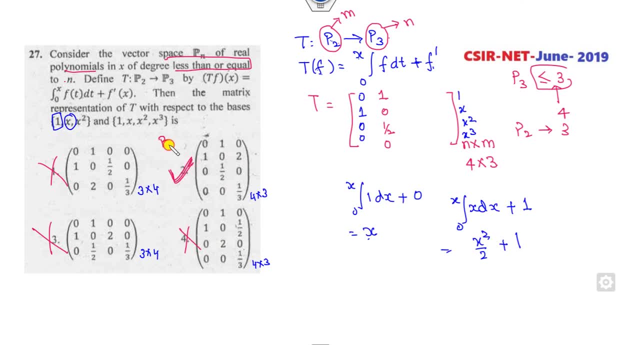 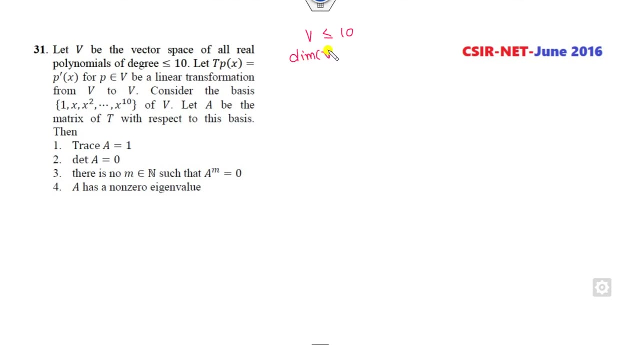 This is not satisfied. Right answer is my b is the correct option. Remember always your target is to discard the options. Okay, v is the vector space of the polynomial less than equal to 10.. So what is the dimension of the v? 11. Because whenever it is a polynomial, 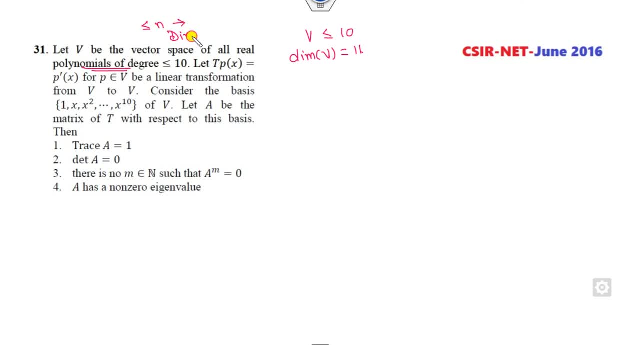 of degree less than equal to n, then their dimension will be n plus 1.. Define the mapping as t of px. This is my derivative. Then you have to define a mapping from v to v. So what is the dimension? What is the size of this matrix? Dimension of v is 11.. So it is 11, cross 11.. Let a is: 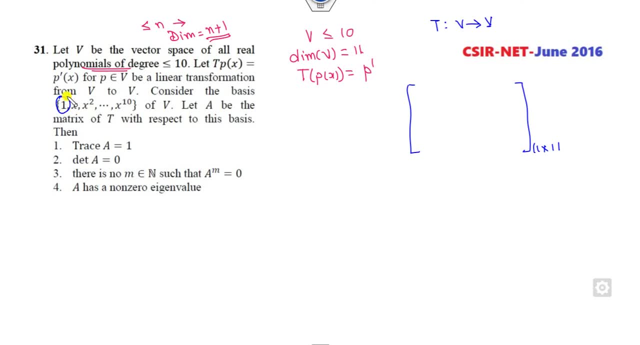 the matrix associated. Okay, fine. So firstly, if I take 1,, what is the derivative is: If I write here as 1 x, x square, the last value will be. last value will be my x raised to power 10.. 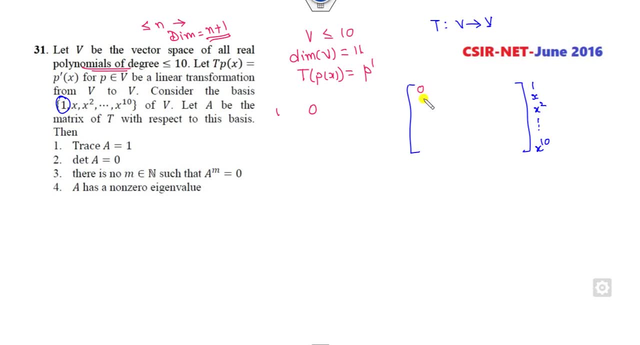 So the derivative will be 0. so 0 is a constant. The rest values are my 0.. If I take as a x, the derivative will be 1. that is a constant value, So it is a 1.. The rest, all values. 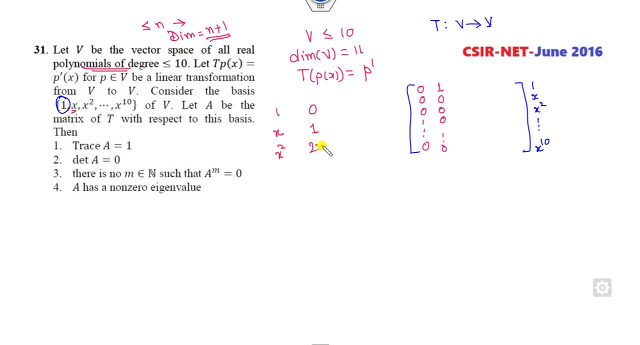 are my 0.. If I take as x square, the derivative will be my 2 x, So 2 x is my here. The rest all values are my 0.. x cube: 3 x square, So x square is my 3.. The rest, all values are: 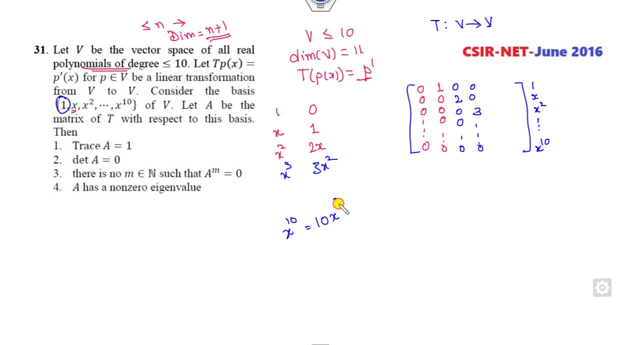 my 0.. Similarly, if I take x raised to power 10, it is my here. x raised to power 9 is my 10, rest all values are my 0.. So what is the meaning of that? You can see. 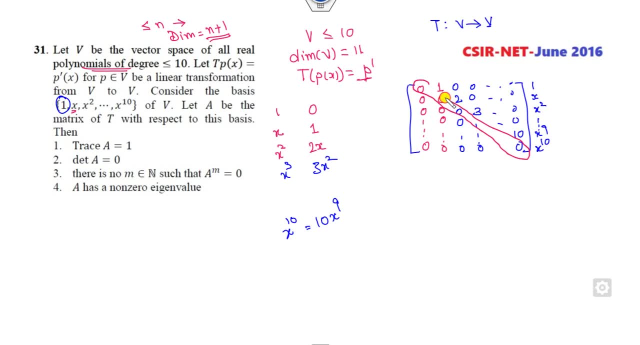 the diagonal values are my 0. So what is the meaning of that? Trace of this matrix is my 0,. the determinant of this matrix is my 0,. okay Now, trace is my 1, cancel determinant is my. 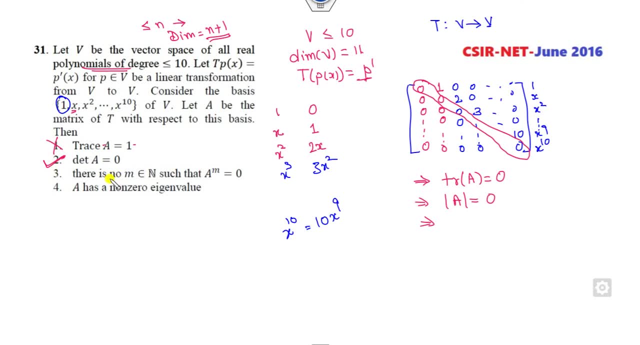 0, that is correct option. There is no m such that a raised to power m is 0. So what is the meaning of that? What is the eigenvalues of this matrix? 0, 0, 0. So 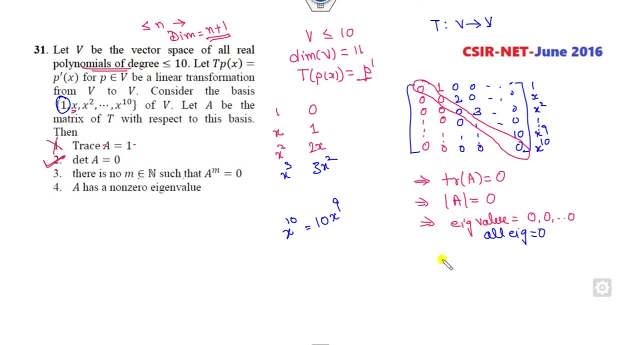 that means all the eigenvalues are my 0.. Once all the eigenvalues are 0,, what kind of the matrix? So this matrix is my nilpotent matrix. fine, So once there is a nilpotent matrix, it means there. 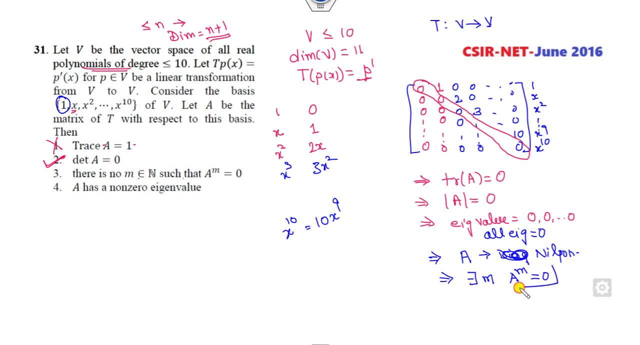 exists a matrix. So once there is a nilpotent matrix, it means there exists a matrix, So at least 1m, so that a raised to power m will be 0, but he said there is no, So this is cancel. 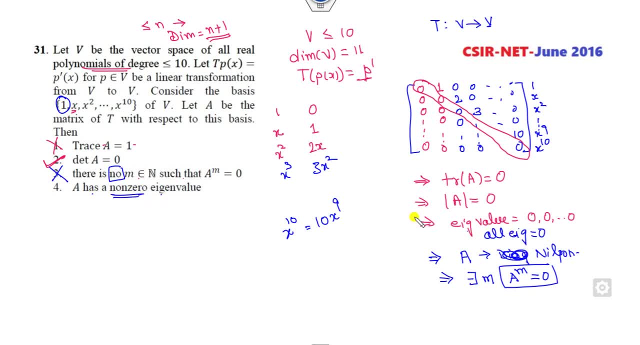 out: a has a non-zero eigenvalue, but all the eigenvalues are 0. So this option is also cancel out, okay. So here one another tips related to that: if a has all the 0 eigenvalue, what is the meaning of that? a is my nilpotent matrix. Once a is my nilpotent matrix, then it is. 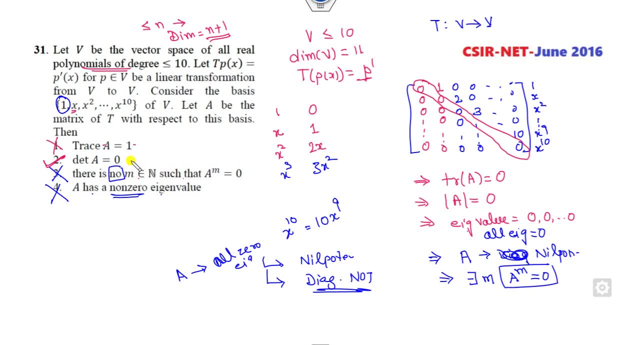 not a matrix. So what is the meaning of that? Once a is my nilpotent matrix, then it is not a diagonal matrix. So, but right now they are not talking about the diagonally blue matrix. But if in, if they are ask you like, a is diagonal matrix. So then again this option is cancel out. 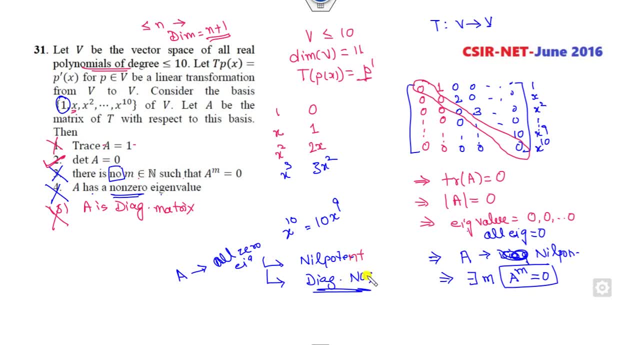 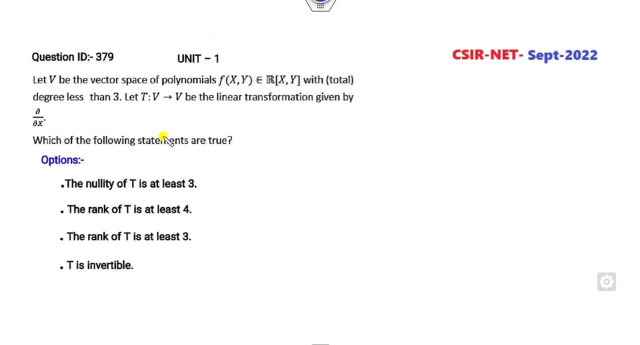 because whenever there is a nilpotent matrix, it can never be a diagonal matrix. So in this case, the right answer is my. b is the correct answer. Okay. v is the vector space of the polynomial F of a. So this is the vector space of the polynomial of a. So here once, a is my nilpotent tricks. 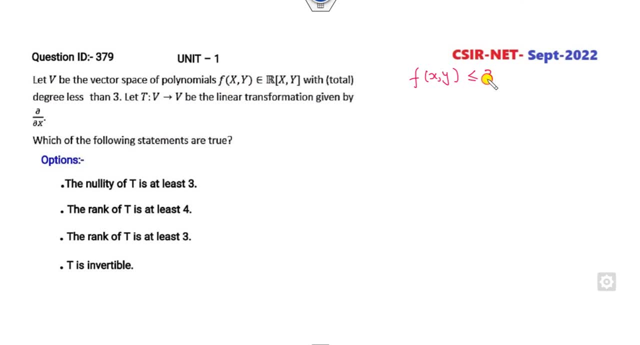 So let us have a look at a dice. So that is my matrix. Once a has a nilpotent matrix, then it is of x, comma y, with degree less than equal to 3. okay, now it's a polynomial of the two variable. 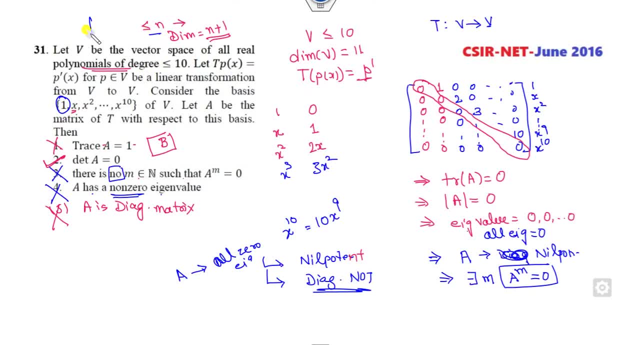 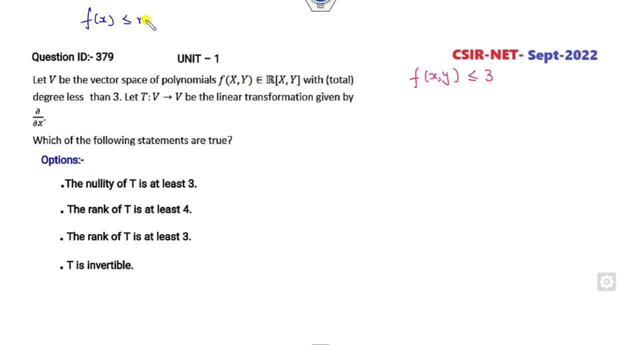 what i discuss in here is: whenever a polynomial of degree 1, then the dimension is n plus 1. like here: whenever is the polynomial of degree n, then their dimension is n plus 1. but whenever there is a polynomial of degree x plus y, that is a function of the several variable and whose 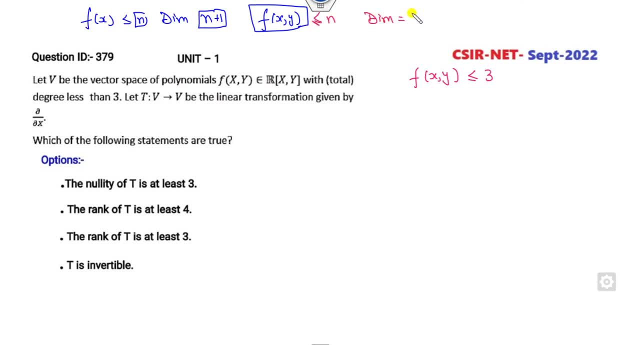 degree is less than equal to n, then their dimension will be always n plus 1, n plus 2 divided by 2. fine, so now in this case it is a strictly less than n, but it not satisfy the equality, so i can return this number as less than equal to 2. so what is the dimension of the f? 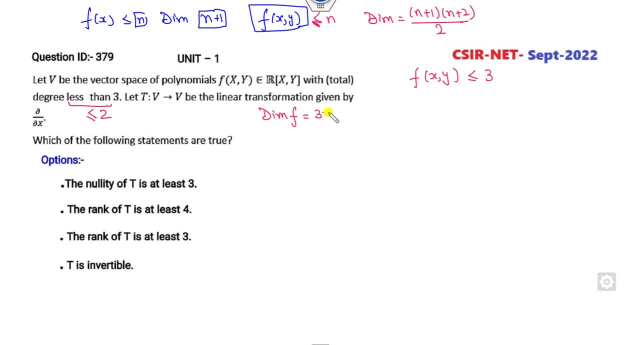 so n is my 2, so it is my 3. 4 over 2, that is my 6. so it means it. dimension 6 means it has 6 degrees less than equal to n. so it is less than equal to n. so it is less than equal to n. 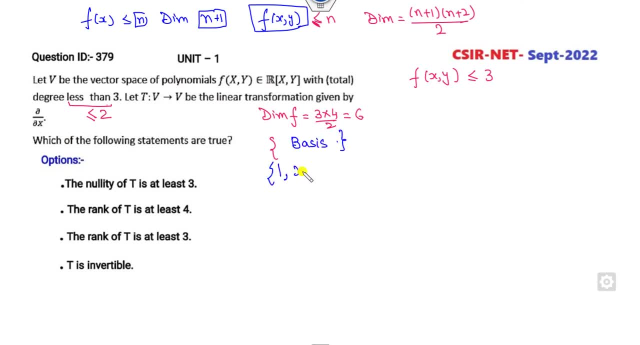 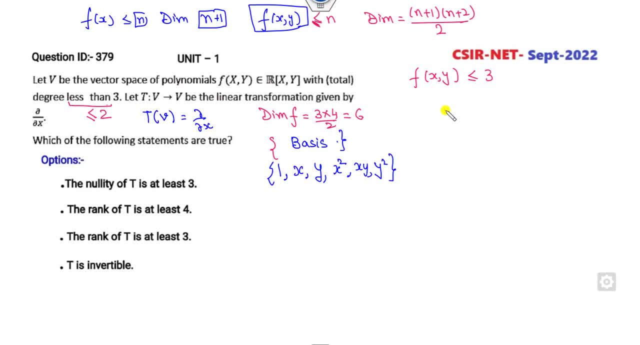 such that it is partial derivative. so now that's over. now it's a 6 cross 6, because dimension of this is my 6, dimension of this is 6, so it's a 6 cross 6. i written as: x, y, x square, x, y, y, square. so look at that. if i take the first, what is the partial derivative of one is: 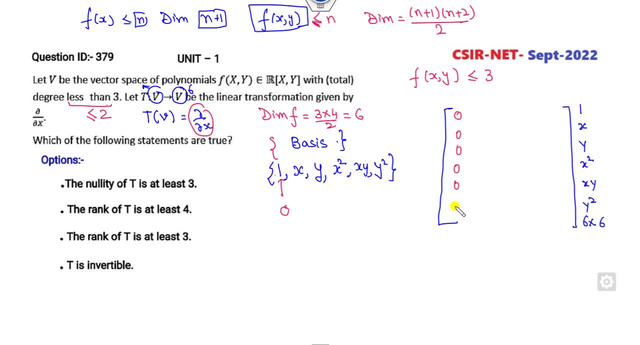 0, so 0 is the constant. rest, all values are my 0. if i take this partial derivative is my 1, so 1 is again constant. it's a 1. rest values are my 0. what is the partial derivative of y- 0? it's a constant. 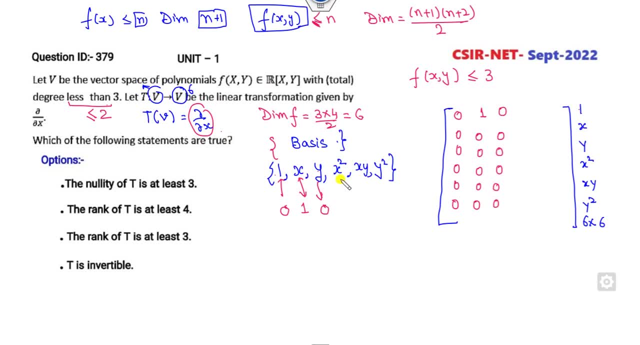 is 0. there is no coefficient of the x- x square here. what is the derivative is 2 x, that's the x. so this is my coefficient of the x. rest values are my 0. coefficient of the x partial derivative is y. so y is my here 1. rest values are my 0. what is the derivative is, with respect to x: 0. so y, 0 is. 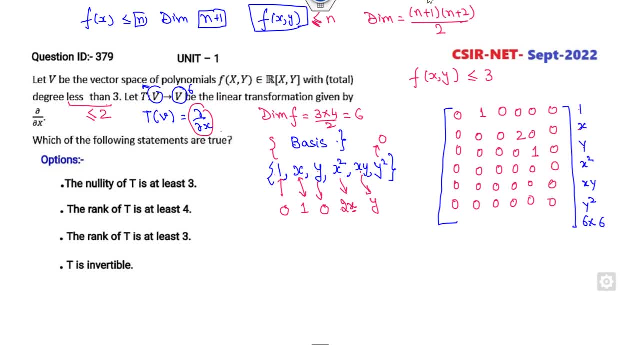 a constant here rest. all values are my 0. fine, now again you can see the diagonal length is: all are 0. so what is the meaning of that determinant of this matrix a, or i call this as a t? then the determinant of t is my 0. trace of this t is my 0. 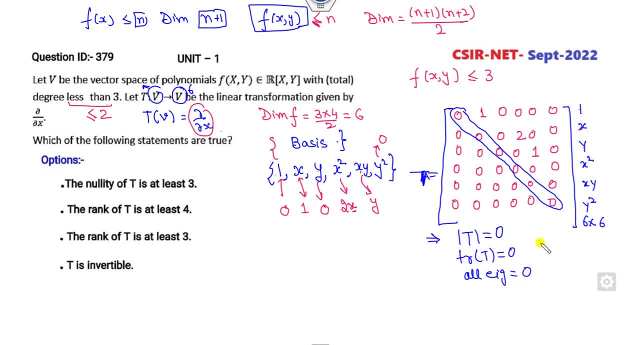 all eigenvalues are my 0. so again, it's a nilpotent matrix and so t is invertible. cancel out, because determinant of t is 0. rank: how many number of the non-zero rows? so you can see 1, 2 and 3. these are: 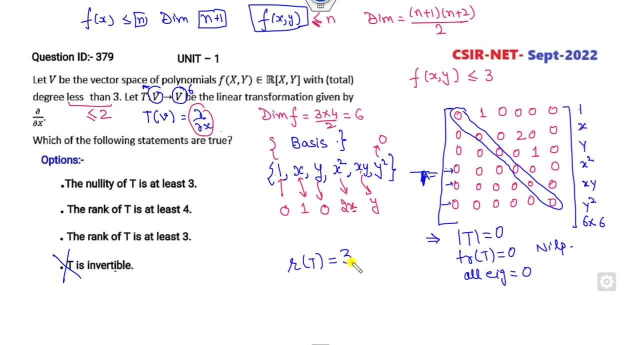 completely 0. so the rank of the t is my 3. so at least 4, cancel out at least 3. so that means greater than or equal to 3. so equality is satisfied. so this satisfied nullity. how you can find the nullity? by using the. 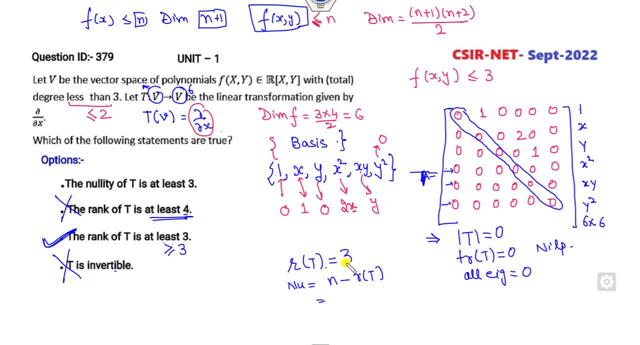 rank sort theorem n minus rank of t. so n is my 6, 6 minus 3, because this is my 3. so it is my here. so nullity will be 3. but he said nullity is verr three at least greater than equal to three. but now you can see, if i say it's a, at least it means. 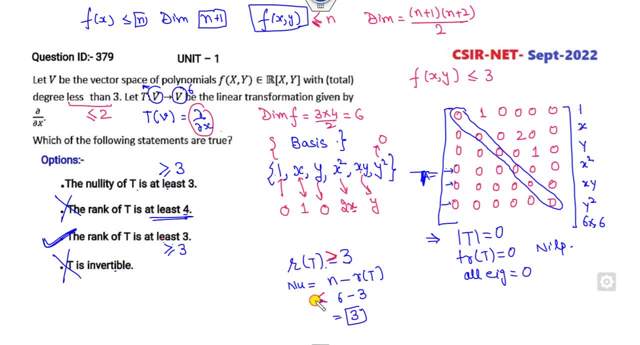 it's a greater than equal to three. if i substitute here, it is less than equal to three. so nullity will be at the most three. so this option is cancelled. this option is cancelled. this cancelled. the only right option left is: this is the right because rank plus nullity is my dimension. so 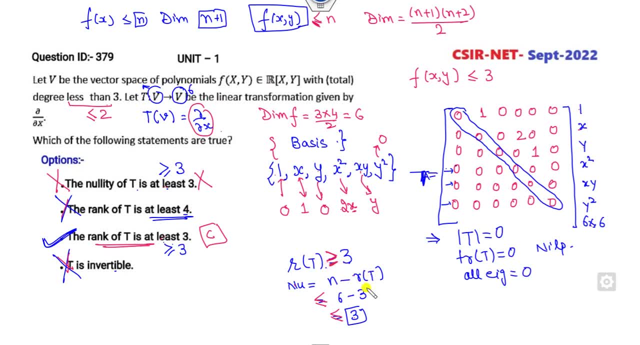 dimension is six, rank is: if rank is my at least, then this is the right, but at least is also satisfied. it is three also, equality, also satisfied, sorry. so this is also the right answer. this nullity is also be the right answer, because if i say rank is my four, then definitely say less than. 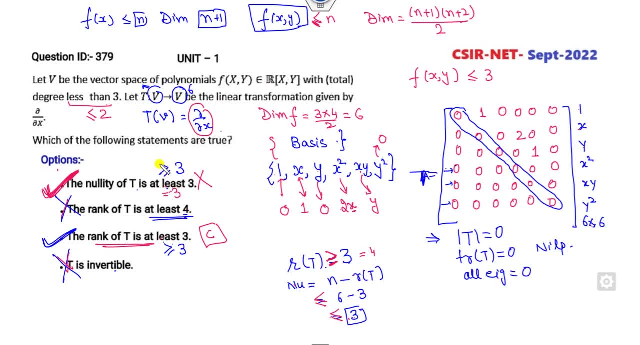 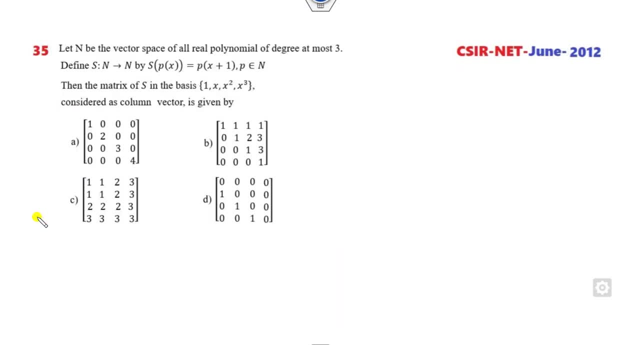 no, it's. nullity is less than at least three is a greater than sign, but we need a less than sign. so definitely, this is not right answer. right answer is c. that's correct. okay, s is a mapping from. okay again, this is a vector space. what is the dimension of the s? 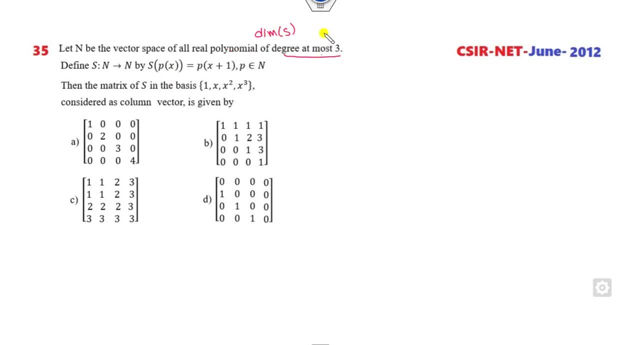 is all the polynomial of degree, at most three at most three. equality is there. so the dimension is my four, so is a s from dimension is four cross four, so matrix will be four cross four. how you define the matrix is my four, so matrix will be four cross four, so matrix will be four cross four. 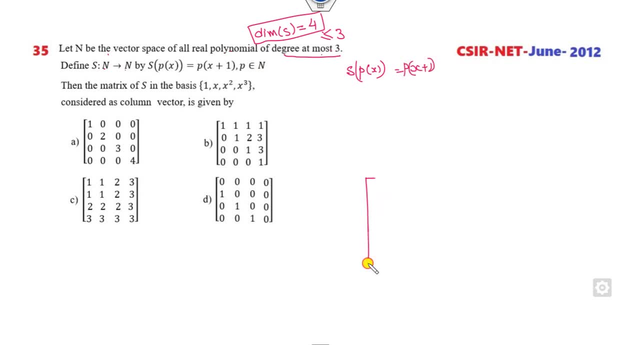 by x plus polynomial of the x plus one. okay, so it will be my four cross, four, degree of three: one x, x, square, x, cube. these are my here. firstly, i can take as a one. so if i take p of x is my one. what is the p of x plus one is again one. so it is one, zero, zero, zero. so this option cancelled first. 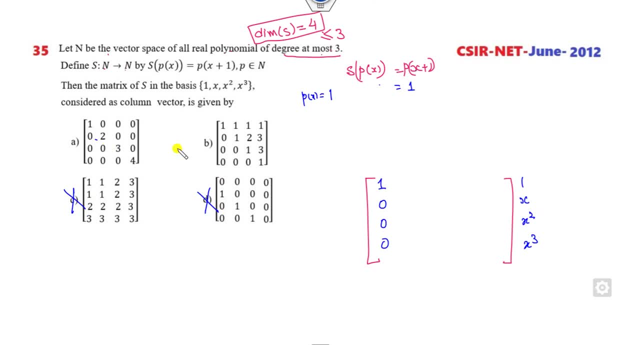 column is here. this option cancelled to two options left. so look at the second column. we will get the right answer in the next. next one: if i take, p of x is my x. what is the right hand side is, if p of x is x, it will be x plus one. so 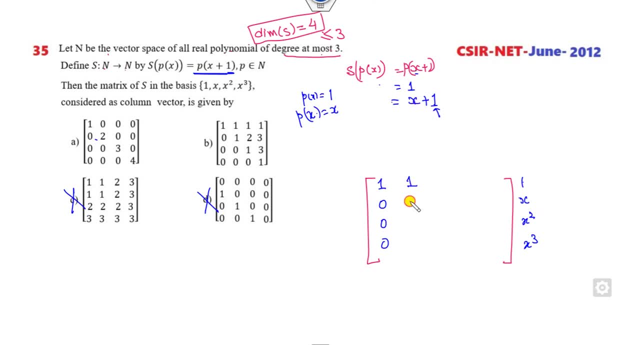 this is my constant. constant will be one. x will be one rest, all are zero, so one one zero. so this is zero, zero, zero. to cancel out all these three, option cancel right answer is my. here is the correct option if you want to check for the other, but there is no need. so if i take as x square, 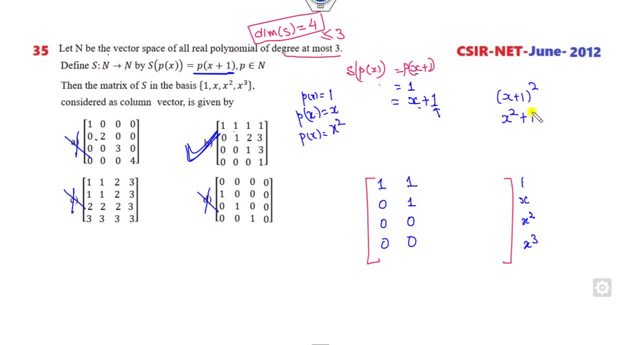 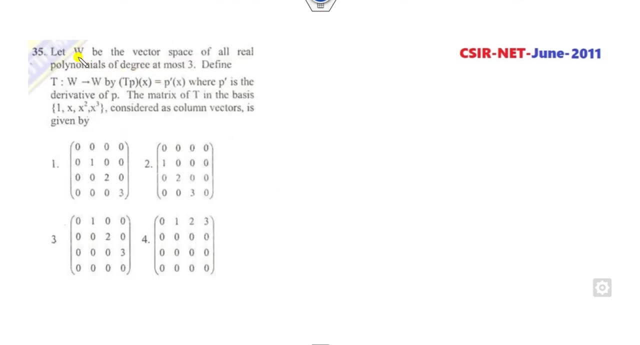 this number will be x plus one whole square, x square plus one plus two. x constant will be one. coefficient of the x will be two. coefficient of the x square is one here one, two one. similarly for the cube is the right also okay. w is the vector space of the. 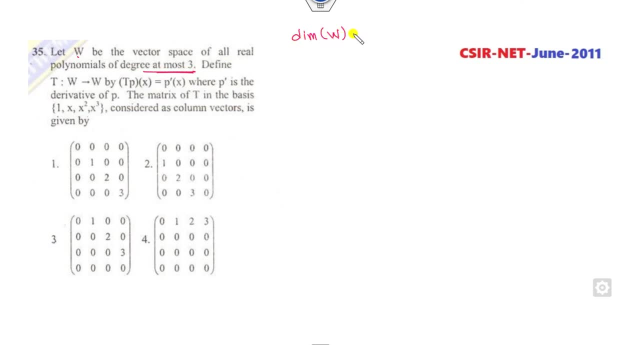 degree, at the most three. so again, dimension of w is my four at most, w is the mapping, t is the mapping from derivative p, dash is the derivative of p. so again, this is my 4 cross 4. what is that? it's 1, x, x, square, x, cube. so what is that? if i take p of x? 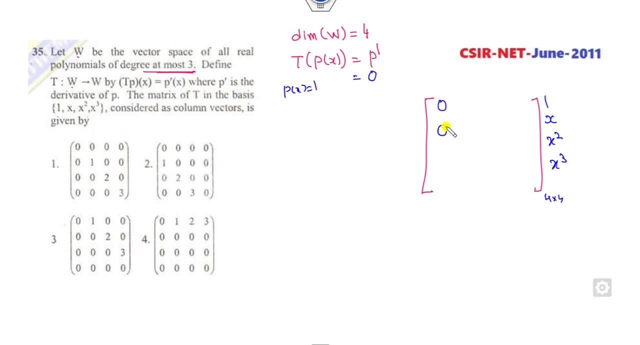 is my 1. derivative will be 0. so 0 is a constant. here all the values are 0. so this option cancel. this is a correct. this is correct. this may be correct if i take p of x is my 1, sorry, x, what is? the derivative is 1, it's a constant here. rest, all values are 0. remember written in the: 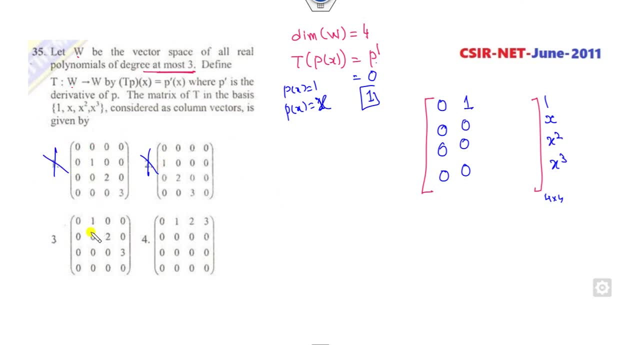 column wise. so this option is cancelled out. this option may be correct. this option may be correct if i take the third option: x square. what is the derivative is 2 x, that's the coefficient of the x. 2 rest. all are 0, 0, 2 0 0 0, 2 0 0, 2 0 0. so this cancel. only one option left is the right answer. 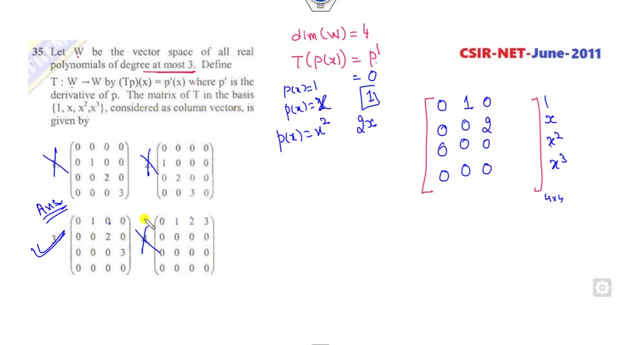 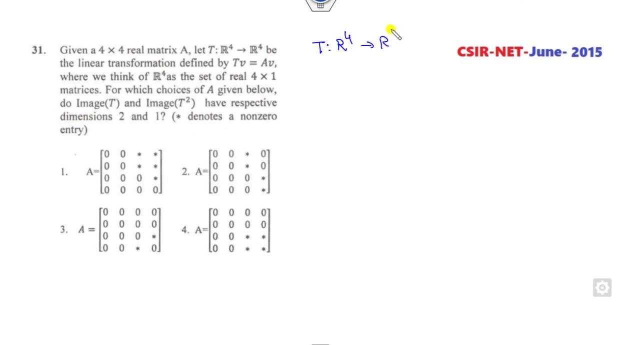 of this problem. you can see within the 10 second you can solve the problem. okay. t is the mapping from r4 to r4. defined by t of v is a v which are the for which choices of the a given by image of t and image of t square has the value 2 and 1? what is the meaning of the image? 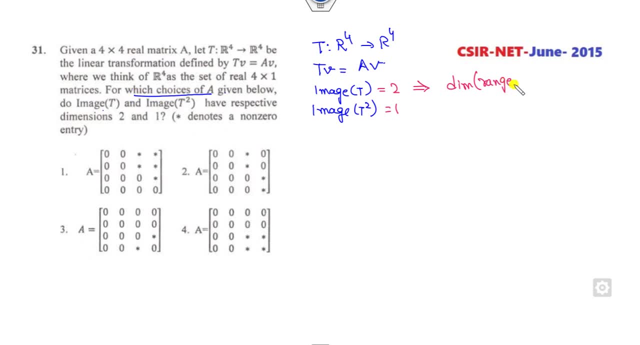 dimension of the range space. that is the meaning of this. what is the dimension of the range space? that is the rank. that is the meaning of the rank. so i can return this number as rank of t is my 2 and rank of t square is my 1, so we have to check this option. what is the star means? 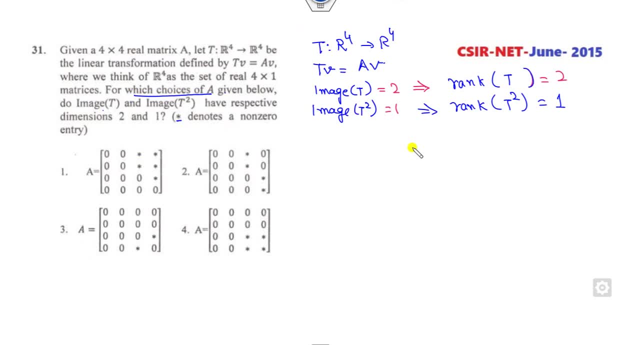 star represents the non-zero angles. fine, so firstly we will check which of the following has non-rank 2. what is the definition of the rank? rank of is number of the non-zeros- non-zero rows, or the number of the non-zero columns, or you can say the dimension of the row space. 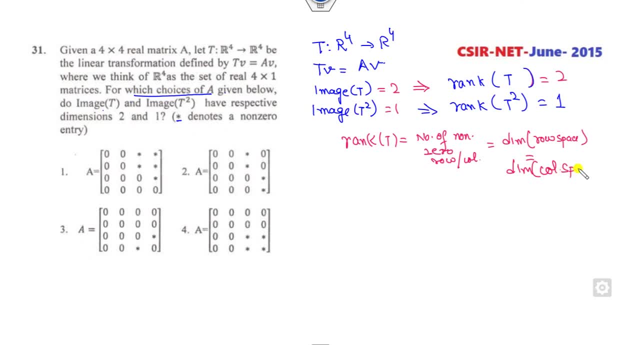 or you can say dimension of the column space. so look at the first column. there are two zero values, two non-zero, so the rank is my two. these are again. rank is my two. these are the two non-zero values. two zero values, so rank is my two. two non-zero values. rank is my two. the first property satisfied. 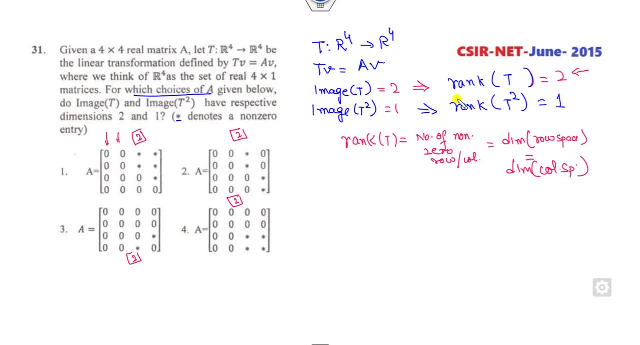 in each case. now the only target, we will check for the rank of the t scale. so how you can multiply them. so if i say this is my four matrix, this can be anything. this can be anything. this can be anything. fine, how you can find the a scale. so one way is you can write this matrix here, but how you can multiply? 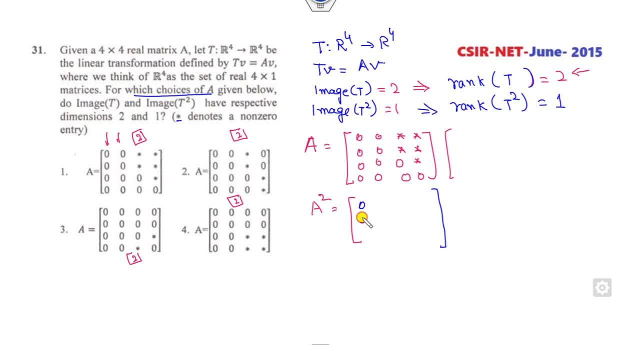 them. that's a simple shortcut fix. i will tell you: the two columns are zero, so you can write this value as a zero as such. now look at that. this is the first row. this is the first row. this element is my a one. three, first row, third column, so you can write the first. that's. the third and fourth are my non-zero value. 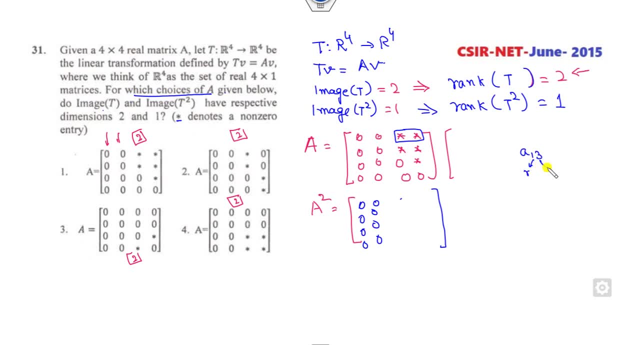 the elements. so i can take the first row, third column, first row, third column. if you multiply them, the value will be zero because the third non-zero elements are there. similarly, if you multiply this as a one, four, first row, fourth column, the first two value will be zero. 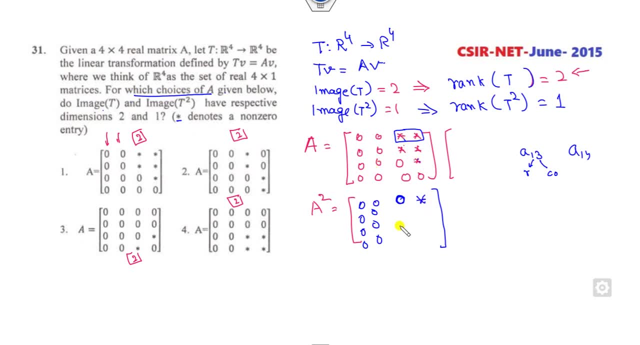 the third value will be non-zero. so it has one non-zero element. similarly, for the other pair, this is a: a two, three: this value: multiply by here, it's a zero. this value multiplied by here, there's a third element: non-zero. similarly for here, this only fourth position is a non-zero. so if you look, 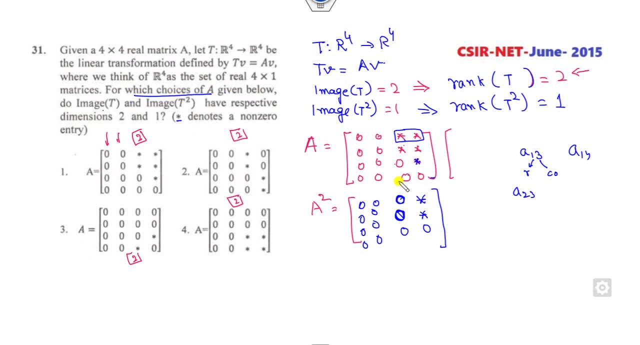 about that. this is zero, and this is a zero, and the last row is zero, so it's a zero. so what is the rank of this? clearly, see is you can how many three zero elements, so what is the rank of that? a square is one, and this is what we need. so this first option is the correct option. now look at the second. 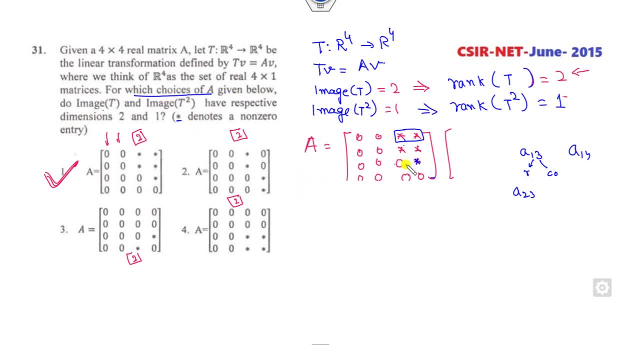 option. look at the second option. here is: this value is my non-zero, fine, so how you can multiply them. so again, how you can easily multiply them, because there is only one correct option. so first we can easily get, but we will see the rest of the option also here. so first column this value. so 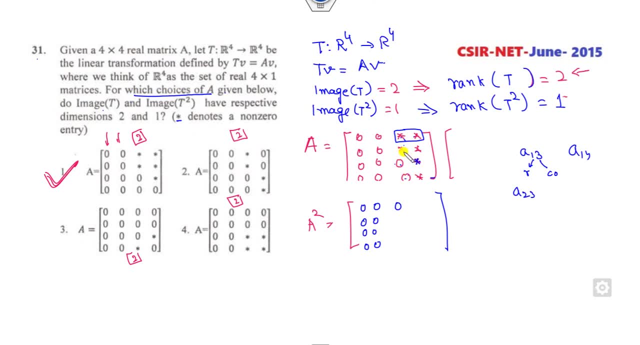 this is a third and fourth option. so third and fourth will be zero. this to the here, third and fourth- is a non-zero. second or third and fourth is a zero: this is a non-zero. third and fourth zero. this is non-zero. third and fourth, this is a last option. this is a. this value will be non-zero. 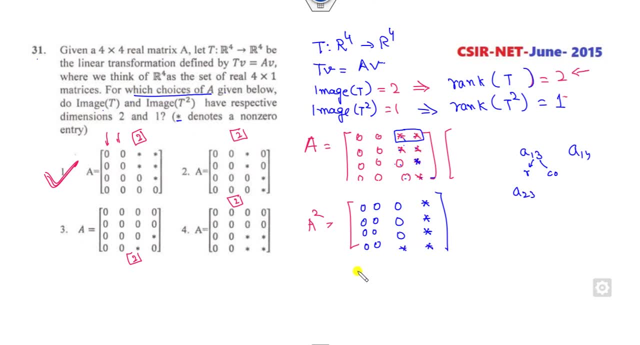 this value will be non-zero. so what is the rank of now? there are the two non-zero rows, are there? so what is the rank of this? there are two non-zero rows, so the rank will be a square two, but we need a one, so this option is cancelled. similarly, how you can multiply this matrix: first, two columns are zero. 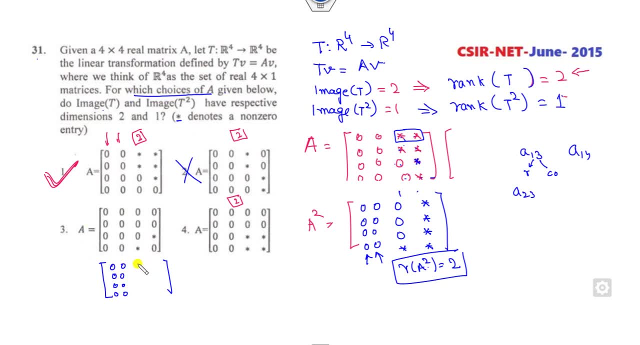 so you can write as directly zero. first. two row are also zero. you can write directly as here now the two values- this value is my a three, two, third row, so only the fourth value are there non-zero. third row, fourth column, third and fourth values are zero. so 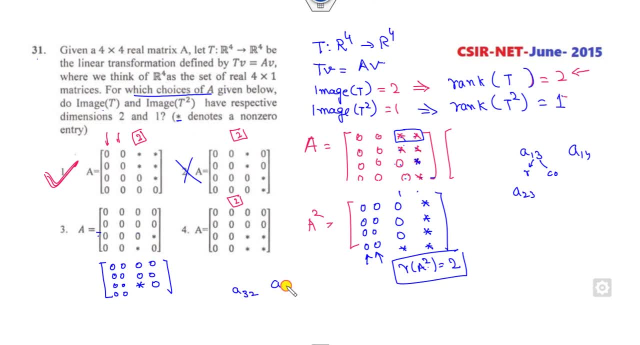 it's a zero. it's a a four comma three, fourth, fourth row, third column. so the last value is a non-zero. this value will be this into: this is a non-zero again. you can see that two values are the zeros. two rows are non-zero. rank of this is my two, but we need again one. this option is cancelled. 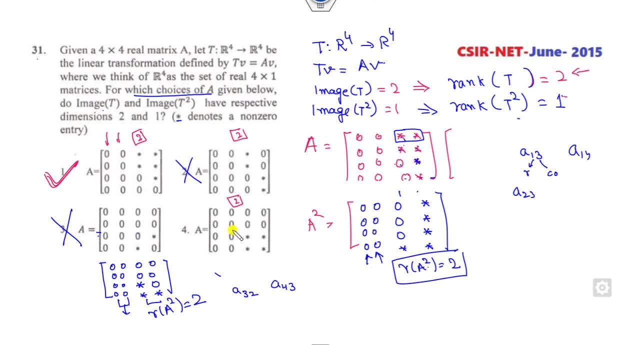 now you can see about this again. so first two values are zero again. so we can. i can write for you here how you can multiply them again. so first two columns are zero, first two rows are zero, so i need to only compute this value. so this value multiplied by this value. 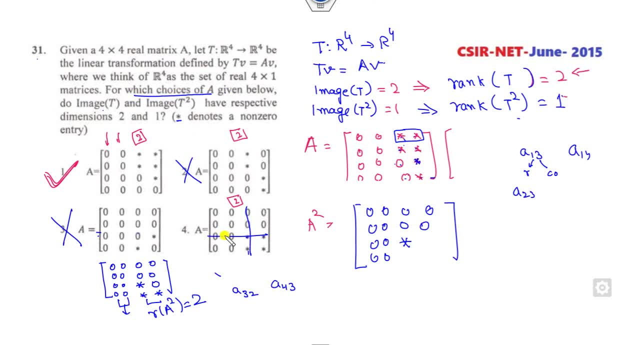 so third and fourth, third and fourth, it's a non-zero. third: this value, this value. so again, non-zero. this value, this value, non-zero, this value, non-zero. so now, what is that the rank? if you again, if you think about that, it's value is a one, one, it's a two, two, if i make them, it's a zero as well. 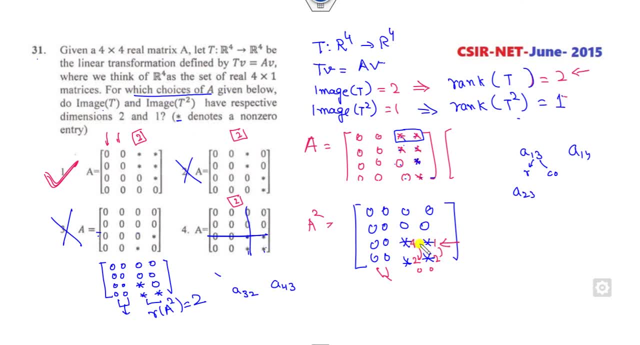 so there is a one non-zero row, but if the value will be four and seven and it's a two and eight, then again will be a rank of this will be my two. so in this case either the rank two or the one, but we always need a non-zero entries. so this option is also cancelled. right option is only a is my. 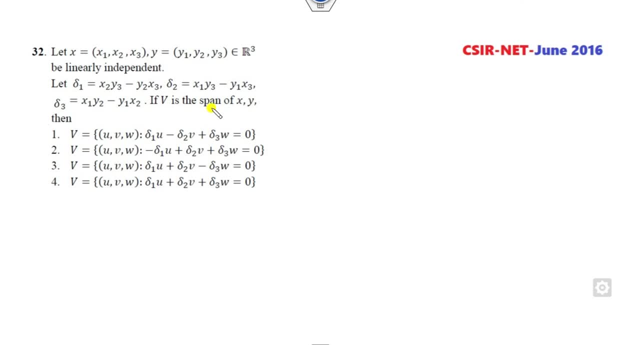 correct answer. okay, look at that. x and y are my li. it is given to you. there are some parameters of given to you. v is the span of x and y. you know what is the meaning of the span. span means basis. you can write in terms of the linear combinations lies. sorry, it's not a basis. 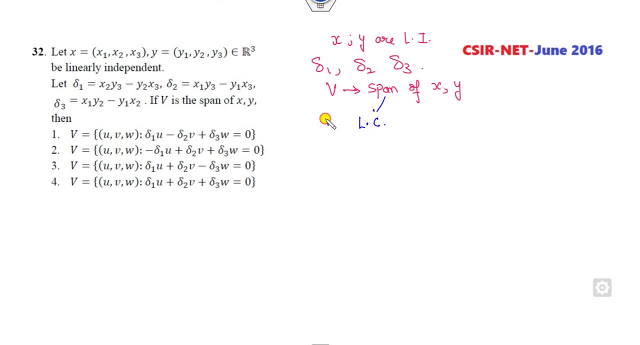 you can write in in terms of the linear combinations. so you can write in terms of the linear combinations- that is, the element of the v is right- as a linear combinations of x and y. what is that, tips? what is the concept for the span? if v is my, u, v, w, what is the definition of the span? that is the definition. 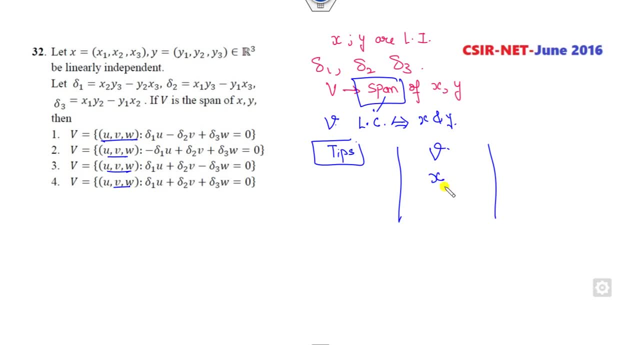 of the span v, x and y. this must be g. that's a simple shortcut text for you. what is the v? v is the element of the so u, v, w. what is the element of the x? x1, x2, x3, y1, y2, y3 is my 0, now we. 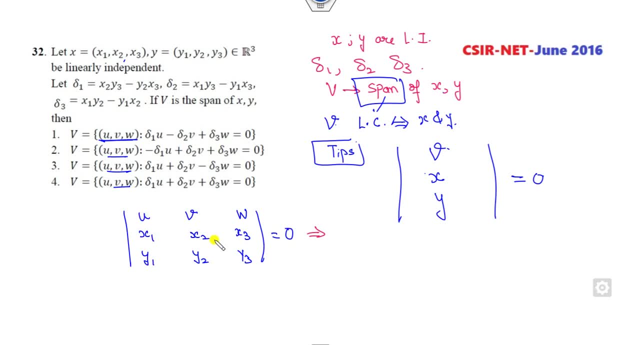 can expand them and check which one is our relation. so if you expand them, it will be x2, y3 minus y2, x3, x2, y3 minus y2, x3. is a delta one of u minus of v, x1, y3 minus y1, x3. is there any value? x1, y3, y1, x2, so minus delta 2, so you can see plus. 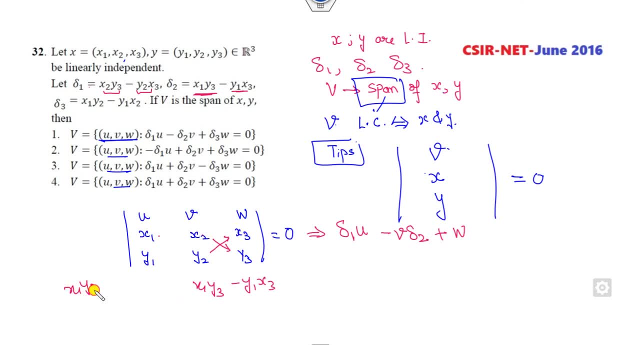 w, it's a x1 y2 minus x2 y1 is a delta 3 is the required answer. you can see the first option correct, minus delta 1. cancel out it's. it's a plus, but we need a v as a negative sign. v as a negative sign, but it's a plus. right answer is only my a. so this is the property of the span. 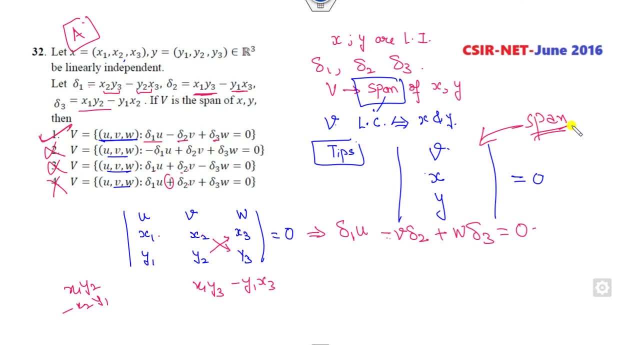 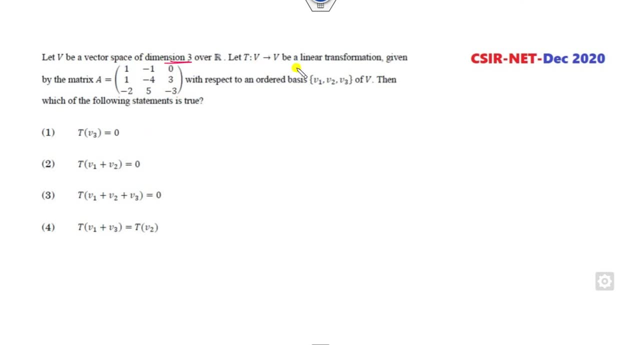 that's a simple tips for you. for the span case. okay, v is the vector of the dimension 3, then which of the following is there? that's a linear transformation. as i mentioned you, always, whenever this is a non-zero, it is called as the non-linear. fine, okay, it's an ordered basis. we 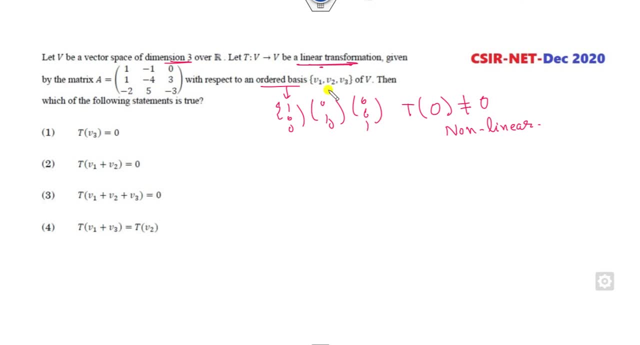 have 0 0 0, 1 0 and 0 0- 1, whenever there is an ordered basis, whatever the column vector. the first column is corresponding to v1. second is columns corresponding v2. third is my v3. fine, so now you can see this is a non-zero. fine, so t of v is non-zero v1, because we all know zero map will. 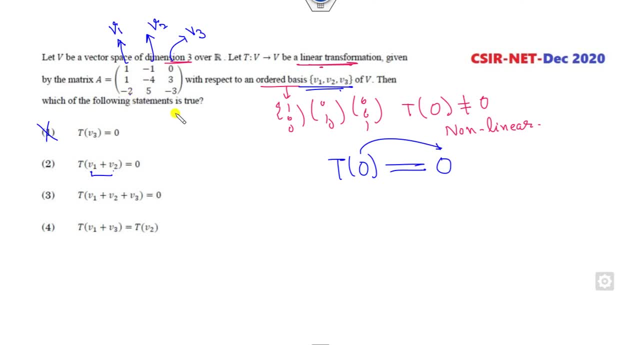 belong to the zero map. so v1 plus v2 is it a zero. zero minus three, three, which is a non-zero, some of them v1 plus v2 plus v3- zero. v1 plus v2 plus v3: zero. v1 plus v2 plus v3: zero. 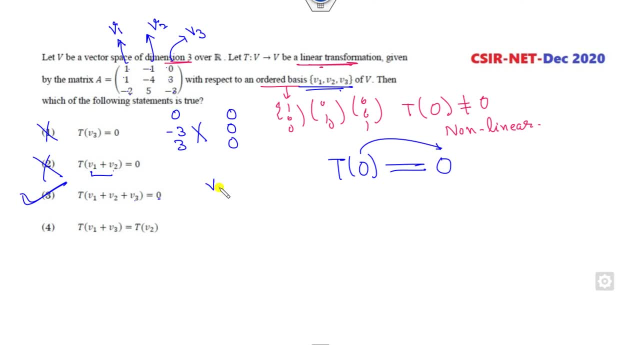 so zero maps to the zero is a satisfied v1 plus v3 is equal to v2. what is a v1 plus v2? it's a one. first one is not satisfied. some of them will be a minus one, but it is a plus one. similarly, it's a: 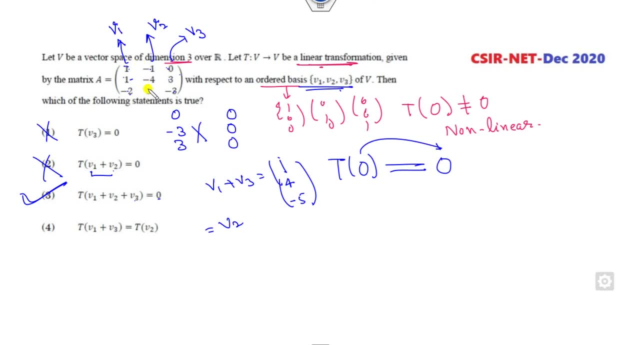 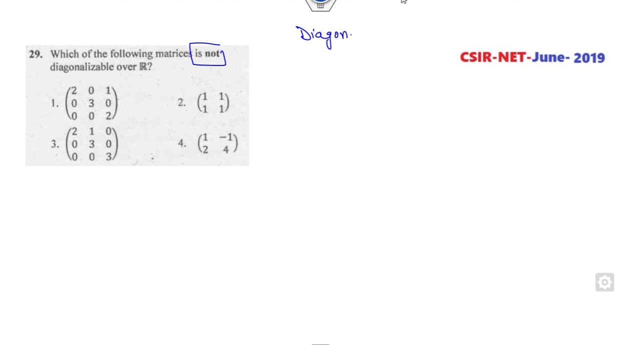 four. it's minus five, but here is a opposite of them. so it's a minus of v2, but it's a minus of v2 plus it's a cancel. right option is the third option is the correct answer. okay, which of the following is not diagonal? so, first of all, what is the tips for you when you can say it's a? 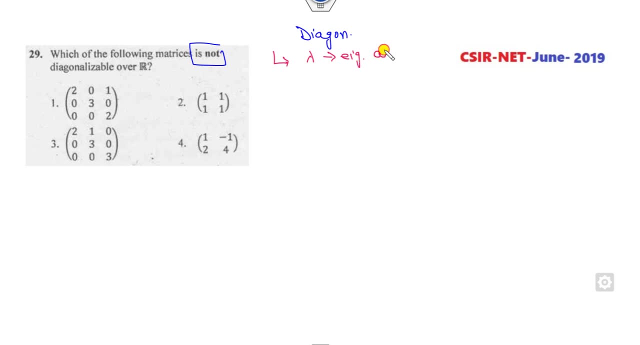 diagonal when you find the eigenvalues. if all the eigenvalues are distinct, then it's a diagonal. second is: if you find the algebraic multiplicity of the lambda, if it is same as that of the geometric multiplicity of lambda, how you can find the geometric multiplicity? this is my n minus rank of a minus lambda, i. third one is: 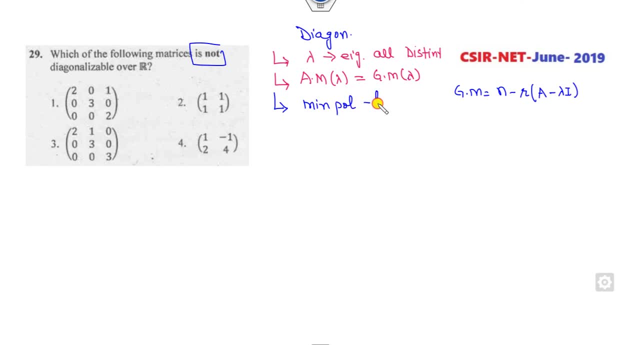 if you prove that the minimal polynomial is in the linear factor, then it's a diagonal. now we will check about this first case. what is the eigenvalue of the first option? 2, 2 and 3? this is a distinct, but this algebraic multiplicity of the 2 is my 2, 2 times. 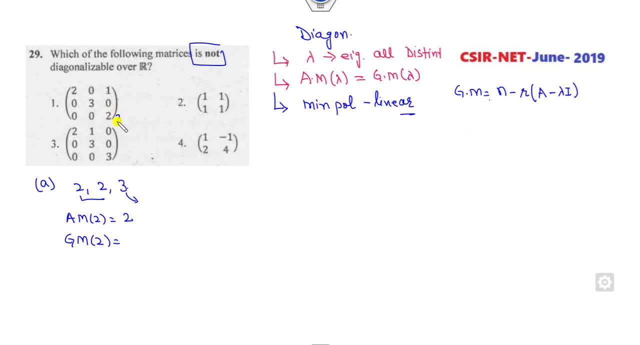 n minus 2 here how you can find this geometric multiplicity here? dimension is my 3, cross 3, so 3 minus rank of a minus lambda is my 2. so what is that? a minus 2, i 0, 0, 1010 0 0, 2. so what is the? 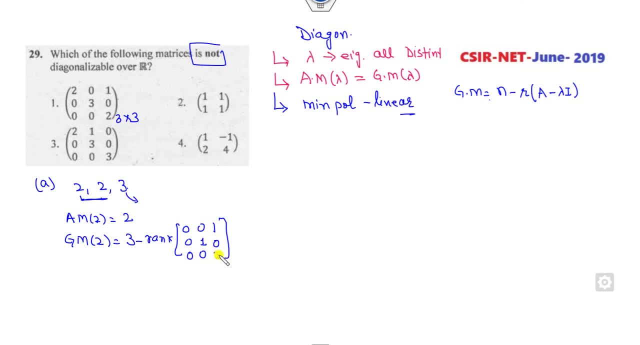 rank of this. you can see I can easily make this value as a zero. are two minus here, so this value will be 0 if I take this value as of this. so what is the rank of this? rank is my two. the rank is 2, 3 minus 2 is 1. so algebraic multiplicity and geometric multiplicity are not same. so it means 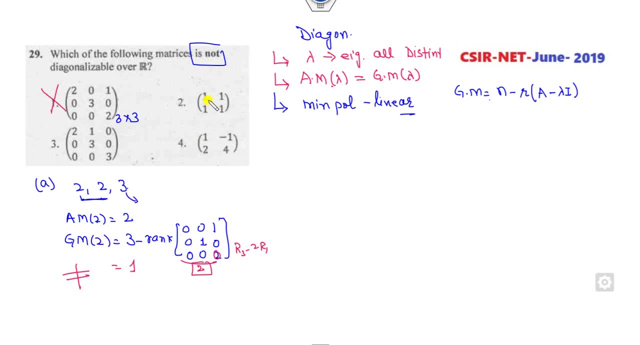 this is not diagonal. here you can, it is a not. so it is not a diagonal, so we need also not. so it means this is the right answer. look at there. you can easily find the eigenvalue. so one eigenvalue is 0, because determinant is a 0 trace is my 2, so second eigenvalue is 2, so you can see these are. 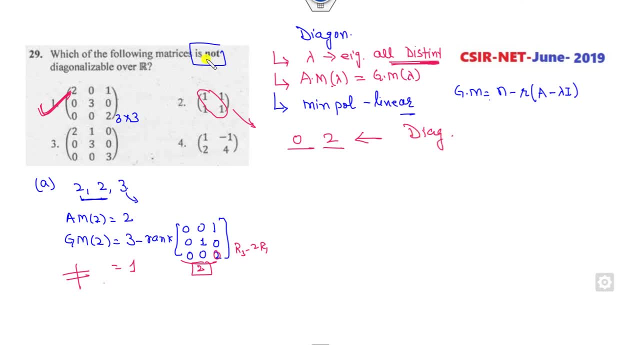 my distinct eigenvalue, so it is a diagonal matrix, but we need a not. what is that? so? lambda, square minus 5. lambda 4 plus 2, 6. so clearly say that 3 and 2 are my eigenvalue, which are the distinct eigenvalues, so it is a diagonal matrix, but we need a not, it's a cancel out. look at this third. 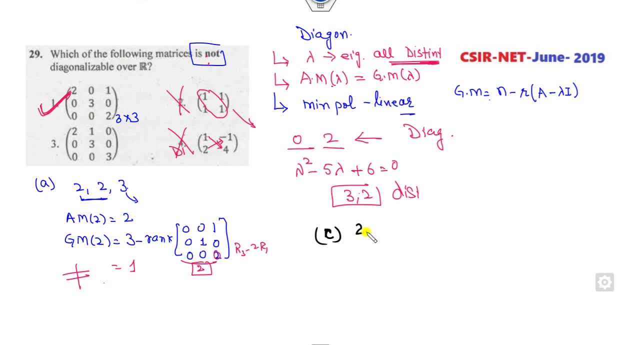 option. eigenvalues are my 2, 3 and 3. this is the distinct eigenvalues, so will check about. algebraic multiplicity of 3 is my 2. what is the geometric multiplicity of the 3? so 3 minus rank of a minus 3i? so what is the rank of a minus 3i minus 1? 1, 0. 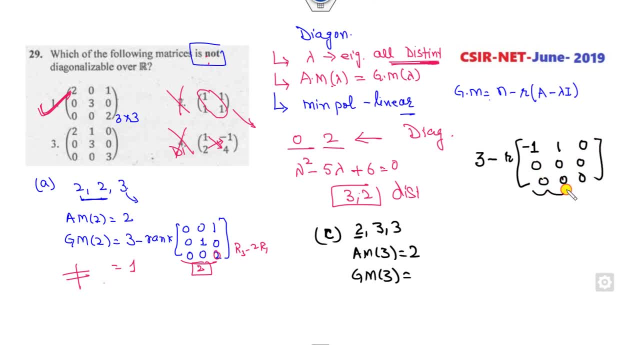 0, 0, 0, 0 0, 0. so rank is my. what is the rank of this matrix? 1, so 3 minus 2 is 2, so once 2, both are same. so this matrix is my diagonal, but we need again a not, so this option is. 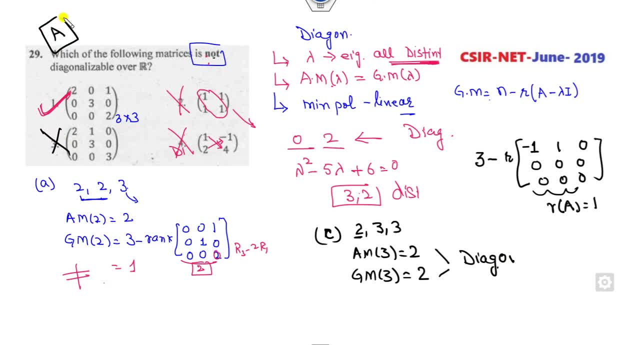 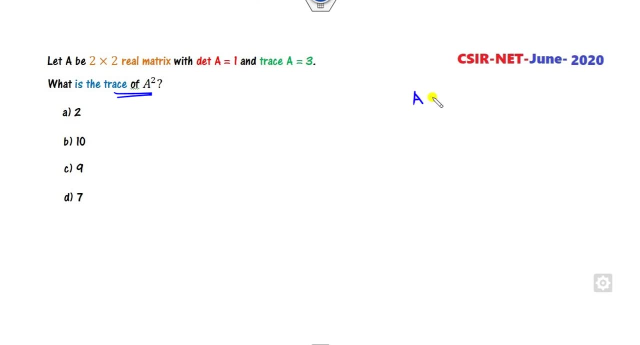 cancelled. right answer is only: a. is my correct option? okay, you have to find that trace of the a. so if i found the eigenvalue of the a here, what is the eigenvalue of the a square? these are my eigenvalue of the a square. then how you can find the eigenvalue of the a square. 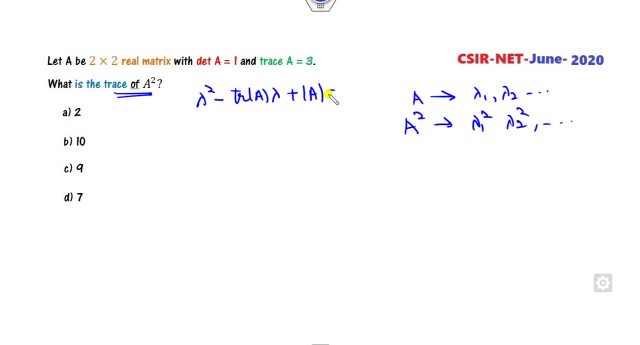 that is the simple trips for you. fine, now, if you substitute here: trace is my 3, determinant is my 1. so what is that? it will be minus b plus minus b square minus 4ac over 2, so trace will be 3 plus 5 by 2. 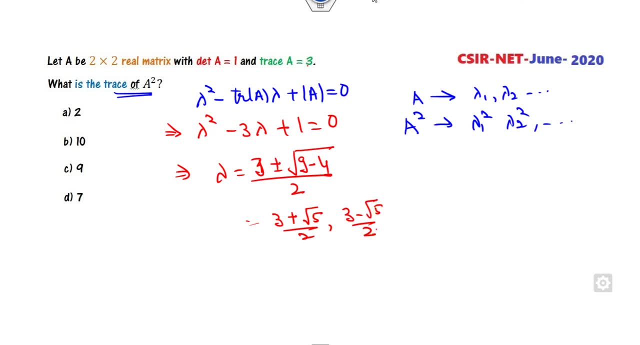 3 minus root 5 by 2. so what are the eigenvalue of the a square? so it is a 9 plus 5 plus 6 root 5 over 4. and second is 9 plus 5 minus 6 root 5 over 4. so what is the trace of this? you can simply: 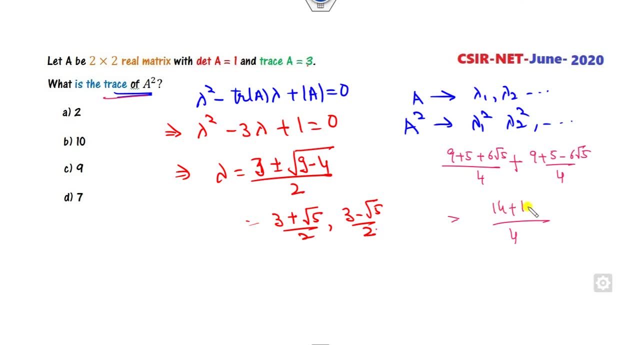 add them, 4 will be lcm. 14 plus 14. 28 by 4: 7 is the right answer. this problem, because you can see easily see this- will be cancelled out. 9 plus 14 plus 14 by 4 is the 8 answer. 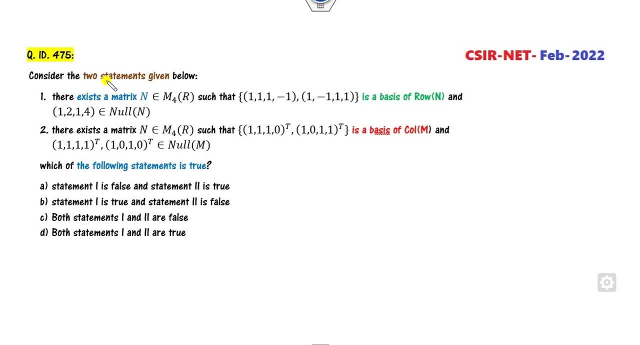 okay, consider the two statement. matrix m4: this is the basis of the row. row means that is the dimension of the rank and this is a nullity. so this is a nullity. statement 1 and 2 are there. that's a very simple. whenever there. 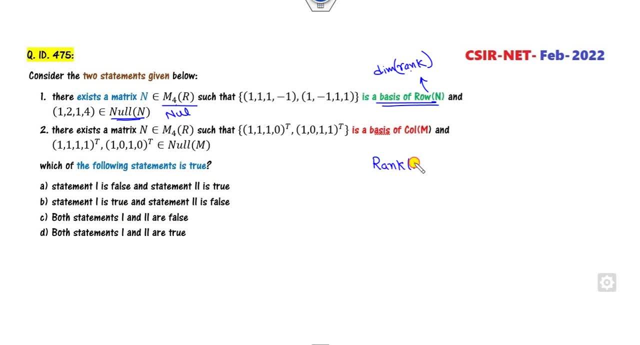 is a rank and nullity. what theorem is applicable? rank of a plus nullity of a is dimension of the vector space. so look at the first case: dimension is my 4. what is the rank? the other two, this is the base, like a nie mal. and here another one. the rank is an addition of 1 and 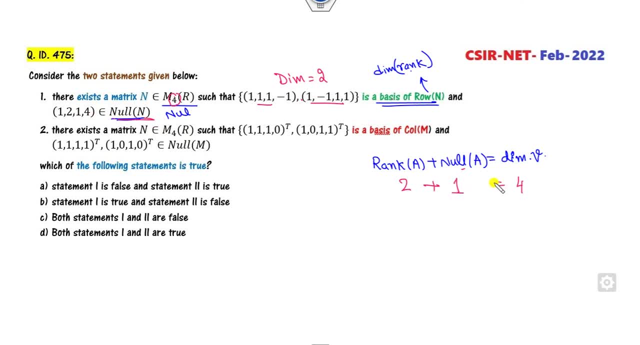 2, so you can see these are known to you as 2 or 0. so at in this case, the dimension is 3 now, which means the kilomani, or volumes, is 4: 4, so 4 express is zero. so, quoting below the value, these are both. these are the blij nous. 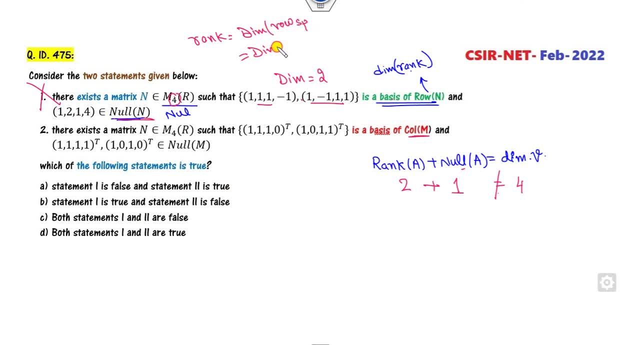 okay, now 0 is equal to 9 and x now mc. we alreadyeff family seats, so similarly, the decimal Zwe 뱉 value say m: 1 to 8 Slim. there are a few variables in the alphabet and you can see it is a column called hash reportance and I see that 2: 0 is equal to 0. 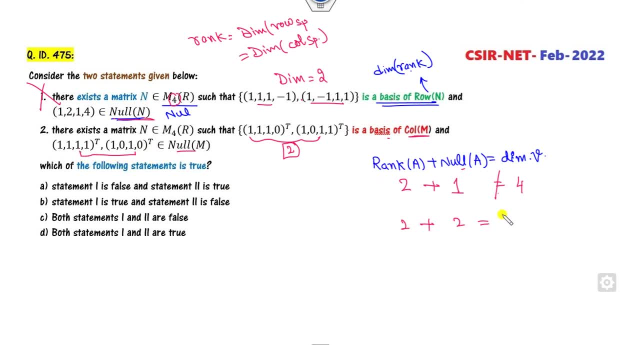 now as follows: R 0, 0 異 Dei is correct to different numbers. My dimension of this is my row space or dimension of column space. so you can see what is that. so 2 plus 2, 4, 2 plus 2 is 4, is a correct statement. so first is my false, second is my correct, first. 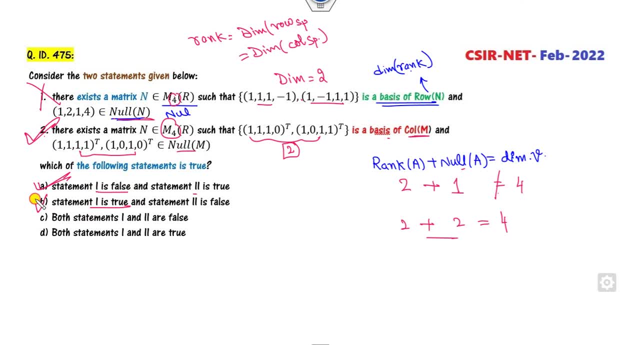 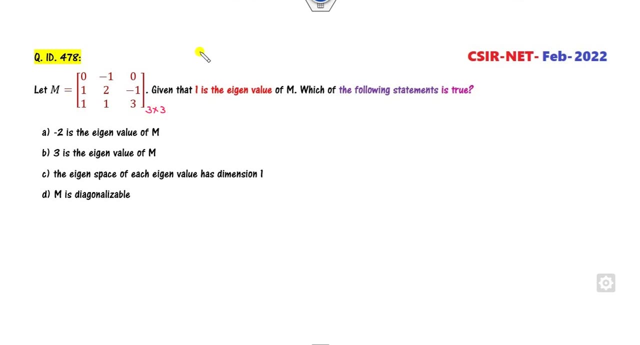 is my false. second is correct. first is to cancel. both the statements are false. cancel, both are to cancel. right answer is my a is the correct option. okay, m is my 3 cross 3. one is eigenvalue, so it has a 3 eigenvalues. one eigenvalue is given to you as a 1, so you need to find the 2 eigenvalue. 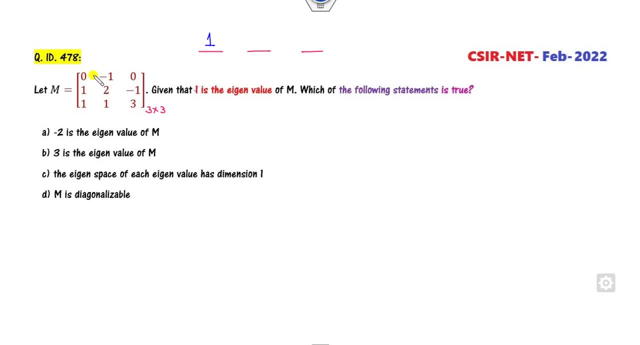 what is the shortcut to x? how you can find the eigenvalue trace of them is 5, but you can see what is the column sum is a 2. column sum is 2. column sum is 2. what is the row sum minus 1, 2, 5? you can see the column sum is same whenever. 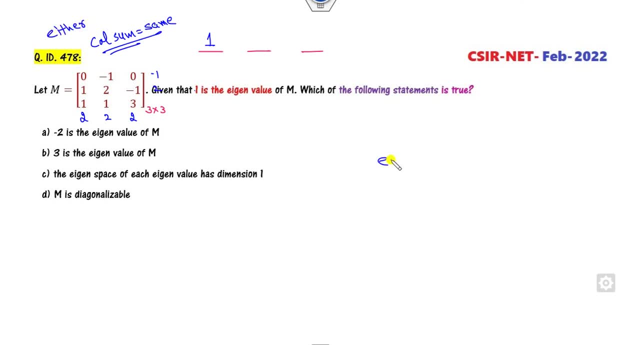 whenever, either whenever either the row sum or column sum are same and say k, then one of the eigenvalue will be my k. in this example, what is the column sum is my 2, so one of the eigenvalue will be my 2, so we know the sum of the eigenvalue will be the trace. trace will be 5, so one, once we know. 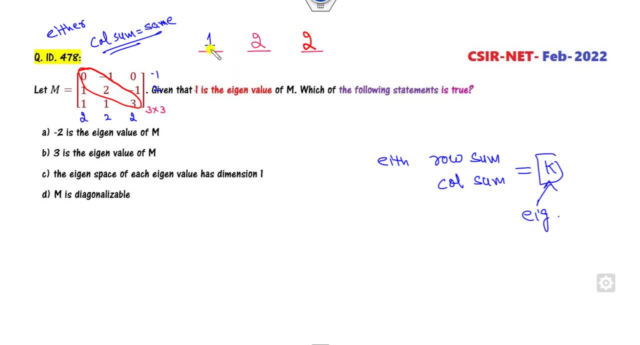 other eigenvalue will be my 2, so the 3 eigenvalues are 1, 2. 2 are my eigens values, so minus 2 is eigenvalue, cancel out. 3 is eigenvalue, is a cancel out. now again how you can check whether it is a diagonal or not. we will apply the same rule. 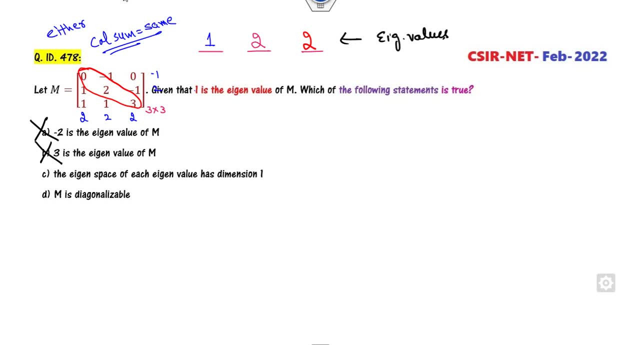 we will check the algebraic multiplicity and the dimension. so this is a single. so algebraic multiplicity of the 2 is my 2, geometric multiplicity of the 2. so how you can check n minus rank. 2 is my 2. so how you can check n minus rank. 2 is my 2. so how you can check n minus rank. 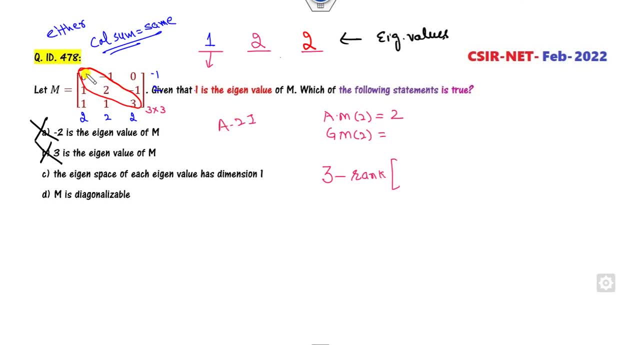 of a minus 2y. so if i take a minus of 2y, what will happen? minus of 2 minus 1: 0. 1 0 minus 1, 1, 1 1. fine, so what is the rank of this? if i separate them here? 1 0 minus 1, it will be 0, it will be 1. 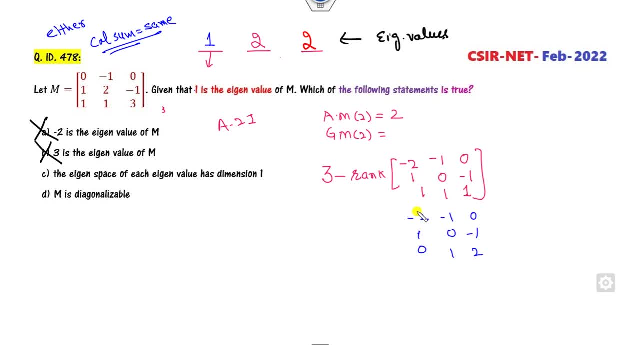 it will be 2 if i multiply by 2 and separate them. so it will be my 0 If I 2 subtract them. same, if I 2 subtract them, it will be my minus of 2.. So if I you can see, so it will be 0, minus 1, minus 2, 1, 0, minus 1, 0, 1, 2.. 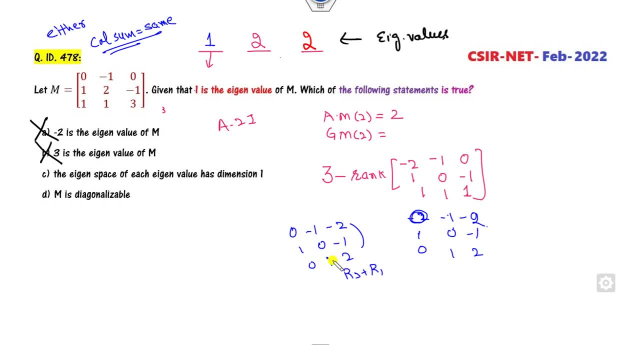 If I add r3 plus r1, this value will be my 0. So the rank will be my 2.. 3 minus 2 is my 1.. So both are not same. So it is not diagonal. So it means m is diagonal. cancel out: only right option is here. 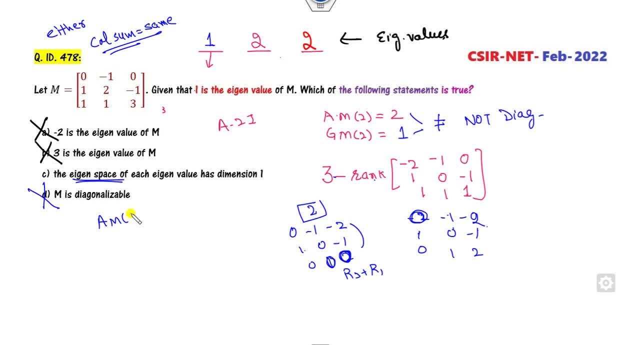 So again, how you can check that? because 1 algebraic multiplicity of 1 is 1.. So since it is a distinct value, so geometric is also 1.. What is the algebraic multiplicity of the? 2 is my 2.. 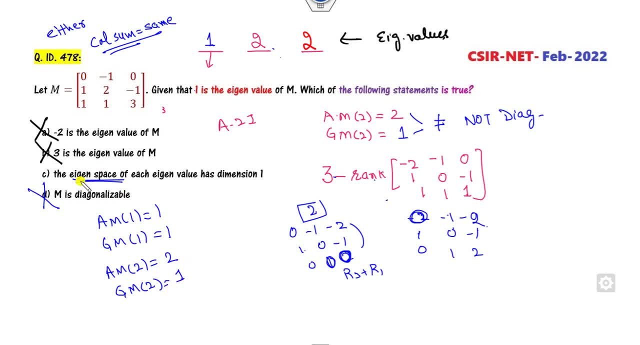 Geometric multiplicity of the 2 is 1. And the eigenspace as each has dimension 1.. What is eigenspace is Eigenspace is called as geometric multiplicity, So you can see Each has the 1 eigenvalues. 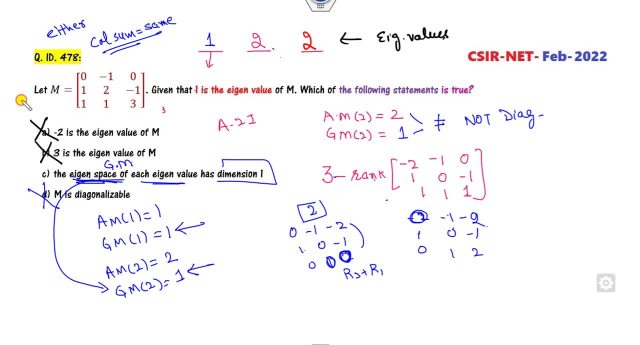 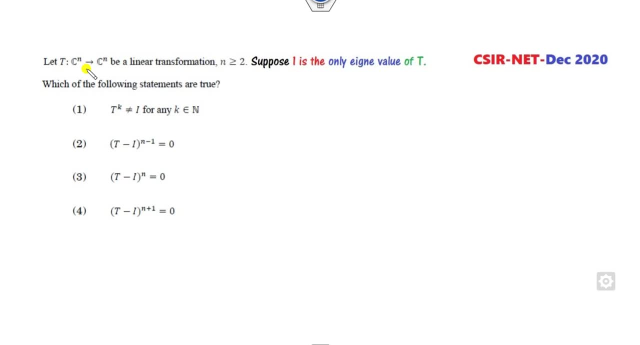 But there is no need to check the third option. The rest of the 3 options, cancel out. So the right answer is: third is the correct answer, Okay. Next option is c: t is my mapping from n greater than equal to 2.. 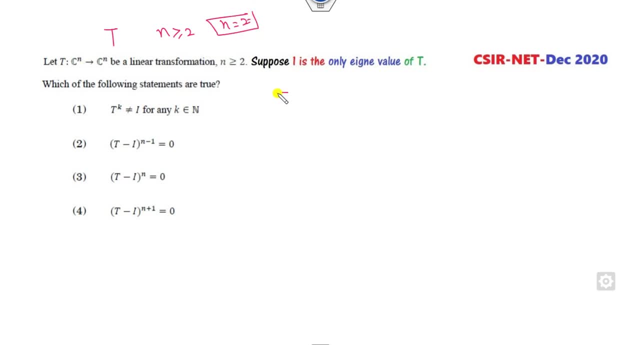 I can simply take: n is my 2.. Fine, So the mapping will be my 2 cross 2.. 1 is the only eigenvalue. 1 is the only eigenvalue. So this is the one count example. That is nothing but my. 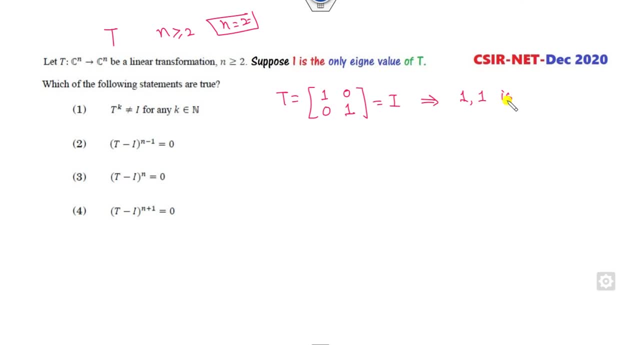 So I can simply say 1 and 1 is the only eigenvalue. Then there does not t raise to power k. Okay, fine, What is that? Whatever the power of the k, you can see this is always 1 or i, But he said not equal to. this option is cancelled. 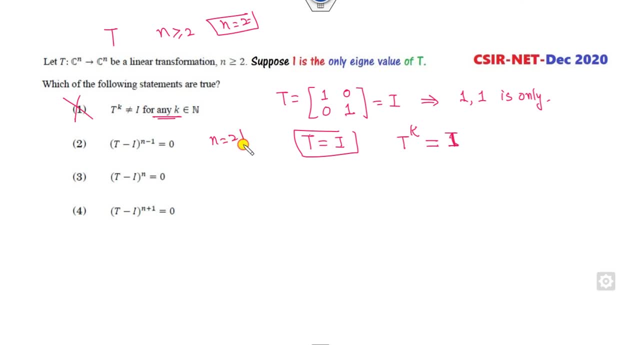 Fine, Now I have taken, n is equal to 2.. So this value will be my 1.. So I have to check whether t minus i or 0 or not. So since this value I have taken as 1i, So it will be 2.. 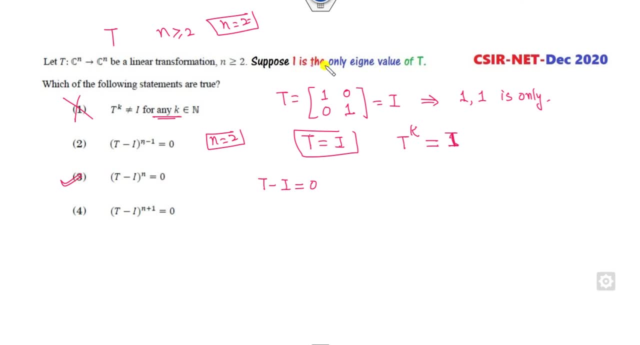 But this is a counter example. Look at this option. If 1 is the only eigenvalue, If 1 is the only eigenvalue of the t, What is the meaning of that? If t has the dimension 2. Then it is a 1 cross 1.. 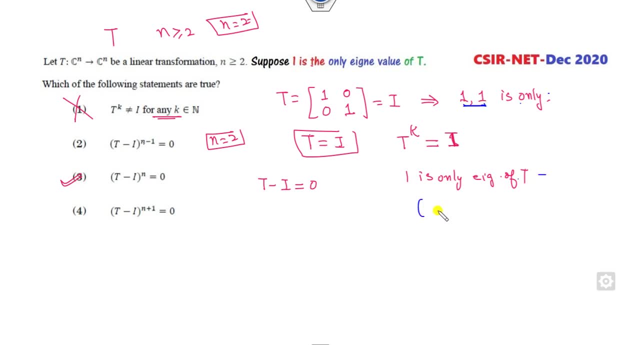 If t has a dimension n, Then it has 1, 1, 1, and here So it means the characteristics polynomial will be my of this, And the Cayley Emerson theorems will say this value will be 0.. So this is the correct option. 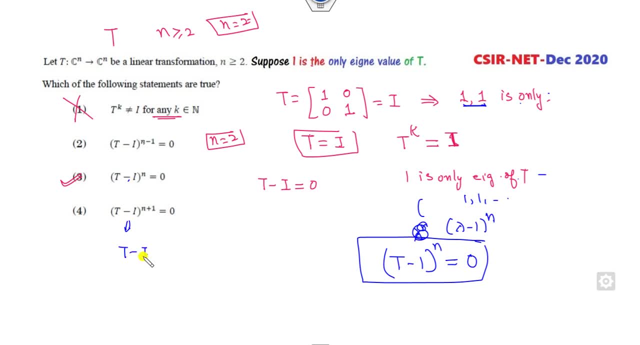 Look at this one. I can return this number as into this of t minus i, So, since this number will be 0. So if you product them, this is also be a 0. How you can check about this option? So now, in case of the 2 cross 2, we can, we can never think about that. 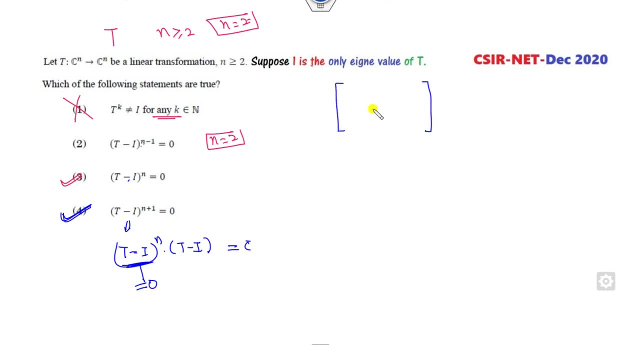 So think about: n is equal to 3.. Say 3 cross 3.. This is my here. If I consider this is my alpha, This is my beta, This is my gamma, Then clearly says: eigenvalues are my 1, 1 and 1.. 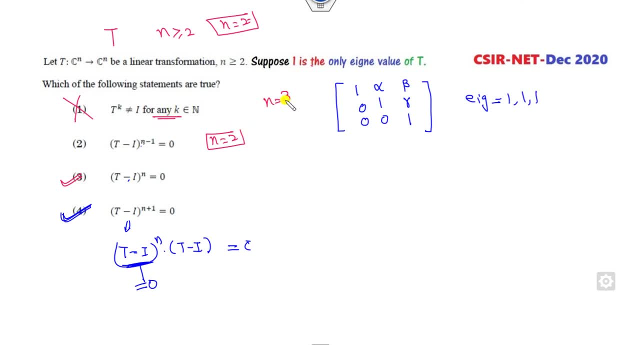 Now, if I take n is my 3.. What will be my n minus 1, 2. It means I need to compute t minus i whole scale. Fine, So firstly, what is a t minus i? 0, alpha, beta, 0, 0, gamma, 0, 0, 1.. 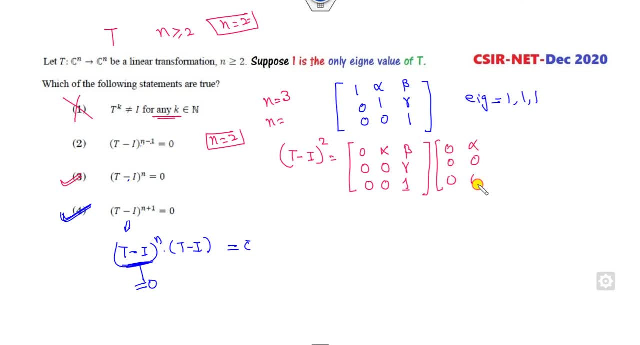 I have to multiply this by here and we need to prove this will be a 0.. Okay, So again, as I discussed you in the previous how you can multiply, the first column will be 0.. This is my a 1: 2 first column here. 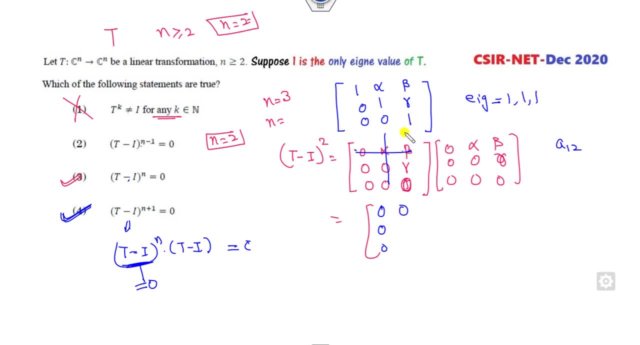 So you can see it's a 0 this value, or you can write this number as here: This is a 0.. Third number will be alpha gamma. This is a 0.. Fine, So clearly say that this will be a non 0, because you can choose any value. 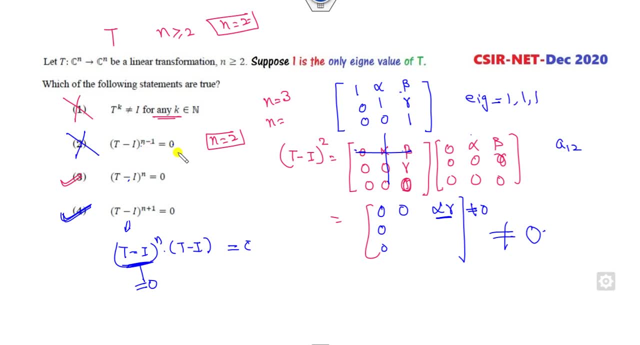 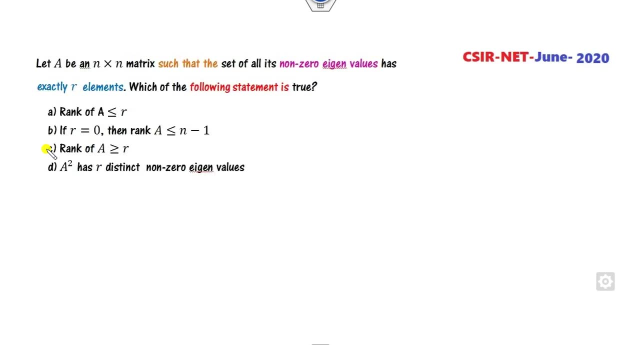 So this value will not be a 0. So this option is a 0 is a cancel out. So right answers are C and D. are the two correct options for this example? Okay Again, a is my n cross n. I consider as a 2 cross 2, such that the set of all the non 0 eigenvalue has exactly r element. 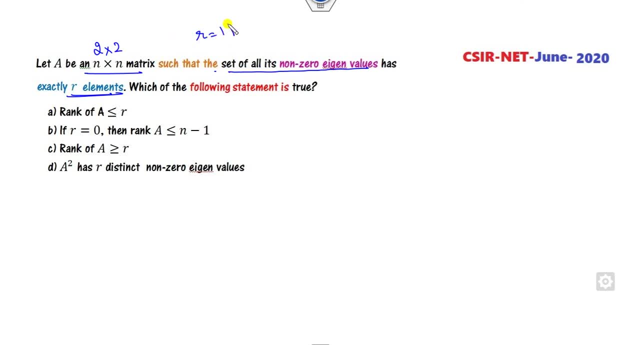 What is the value of the r? R can be anything, So r can be, I think, as a 1.. What is the meaning of that? If I consider that 2 cross 2 matrix, the set of all the non 0 eigenvalues has exactly 1 element. 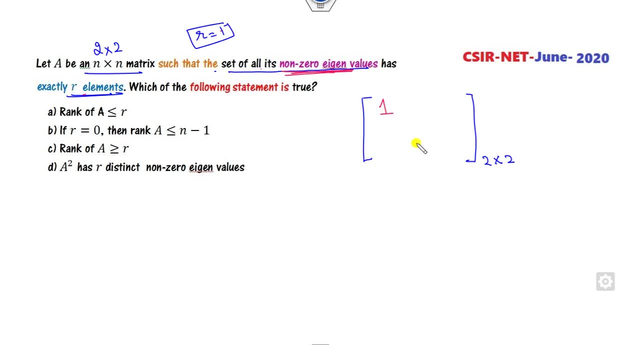 At least one value has a non 0 eigenvalue. Other values may be 0.. Fine, So if I consider this as again 0.. So this is my matrix A, which satisfy this property. What is the rank of this matrix? Rank is my 1.. 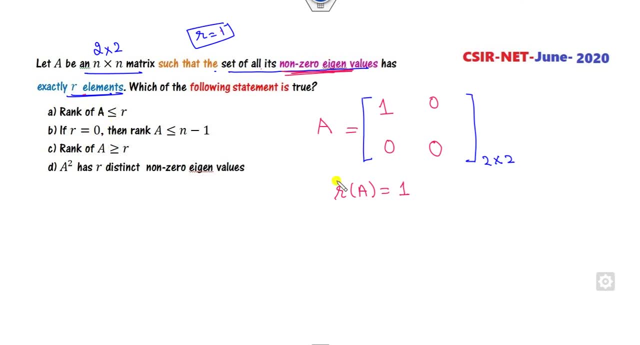 So Rank is my 1.. Okay, But he said less than or greater than. Fine. What will happen if I consider: Is my Say 3 cross 3, because in this case it less than 1 also satisfy greater than. 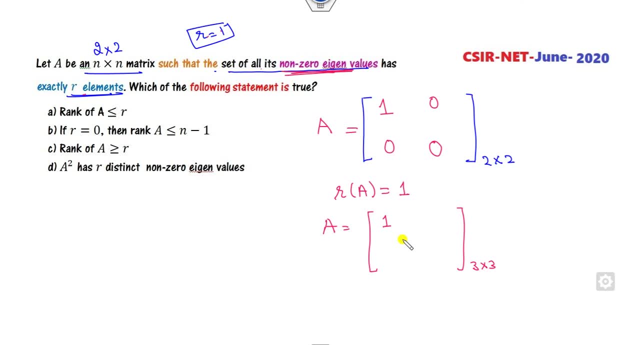 So let's say r is 1, 3 cross 3. it has 1 here. So rest are say my 0. Fine, So this is the set of all its non 0 eigenvalues has exactly r elements. I consider r is my 1.. 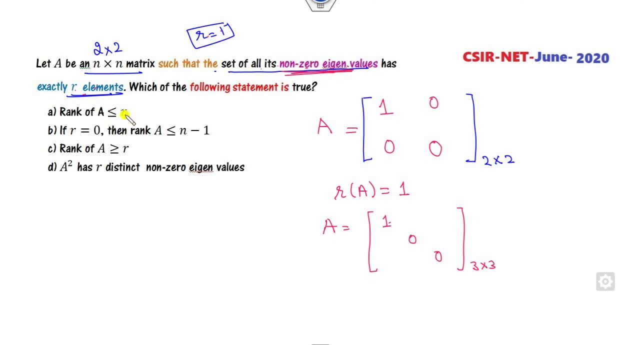 Now, what is the rank of this? Can you say rank is less than equal to 1 or rank is definitely is a greater than equal to 1.. If I say this is alpha, or I can simply take say is a 2, 3, 4, 0, 0, 0.. 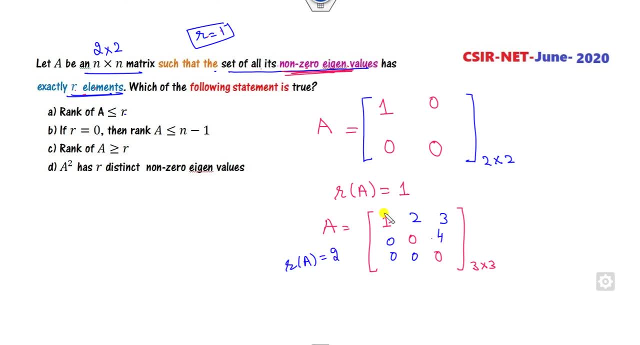 What is the rank of this matrix? It is my 2, which is greater than of the r, So it's a greater than or equal to. if I consider this as a 0, then rank will be 1.. If I consider this as a 10, then it will be greater than or equal to r. 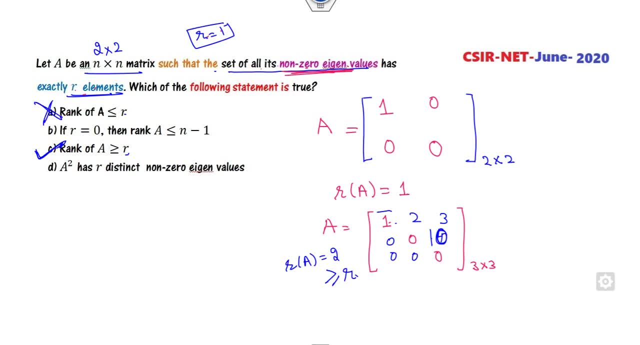 So this option is correct. This option is cancel. A square has the r distinct, non 0, eigenvalue. that's the wrong option. If I consider this value, are there 1 and minus 1.. If I consider r is my 2. these are the distinct eigenvalues, but a square is a 1- 1.. 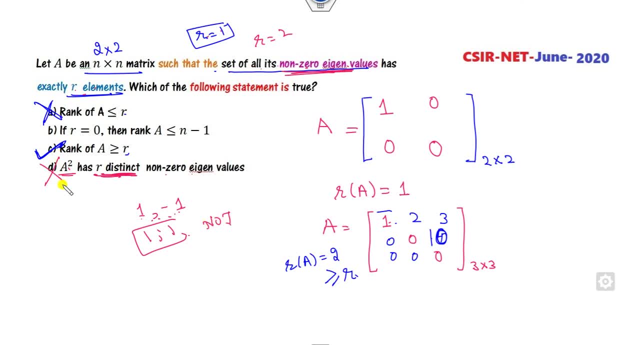 So that's a distinct, it's not a distinct. these are the same is a cancel out. If r is my 0, then the rank will be if I consider n is my 3.. r is 0. It means set of all the it's non 0 eigenvalues has exactly 0 elements, and r is 3.. 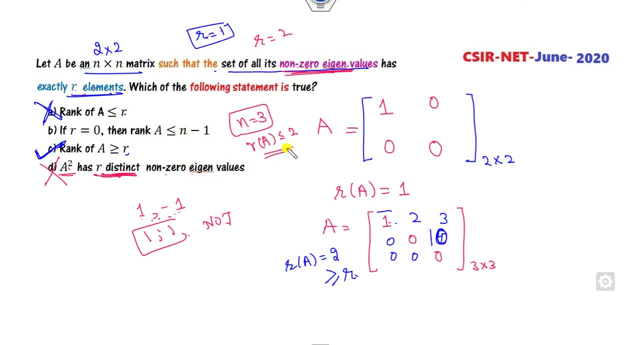 So rank will be less than equal to 2.. What is the meaning of that? If I consider, r is 0, so none of them is there. So what is the rank of this? Rank is always be less than equal to, that's not always 2.. 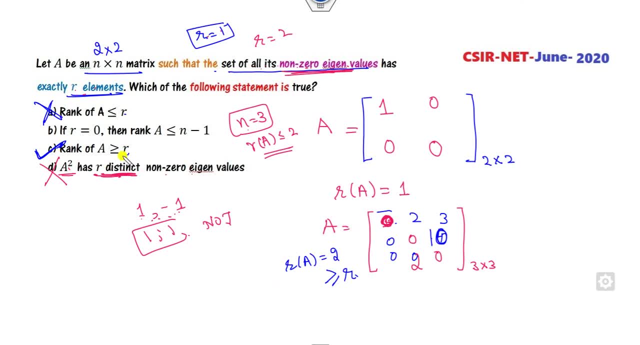 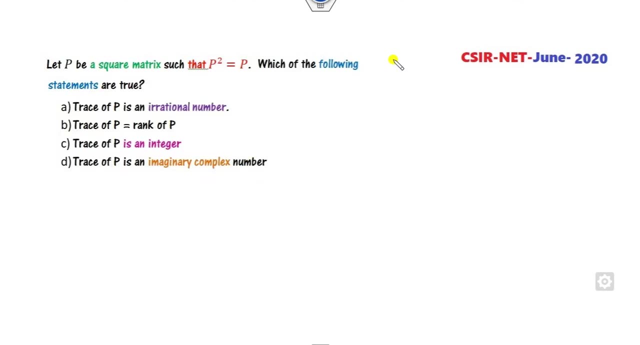 If I consider this value as a 2 here, fine, because in this case it's simply set, So it definitely. this equation will not satisfy for this example. So because there is only one correct option, So c is the only right answer. that's already cancelled. 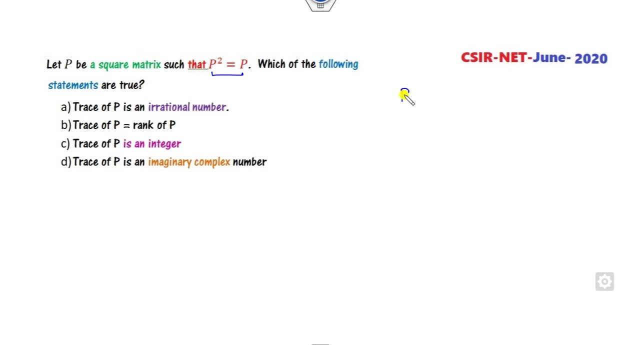 Okay, What is that? p square is equal to p. Do you remember what is that? This is idempotent matrix. Fine, Now what is the tips for you? once this idempotent matrix, Then the rank of the p is always be equal to the trace of the p. 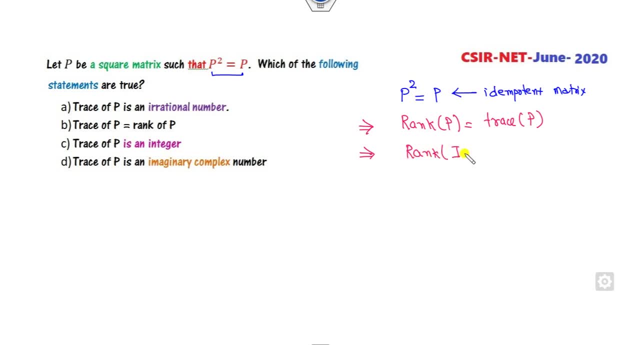 Also, the rank of the I minus p is same as that of the trace of the I minus p. Fine, These are simple tips for you. What are the eigenvalues? What are the eigenvalues of this? Eigenvalues are 0 and 1. fine. 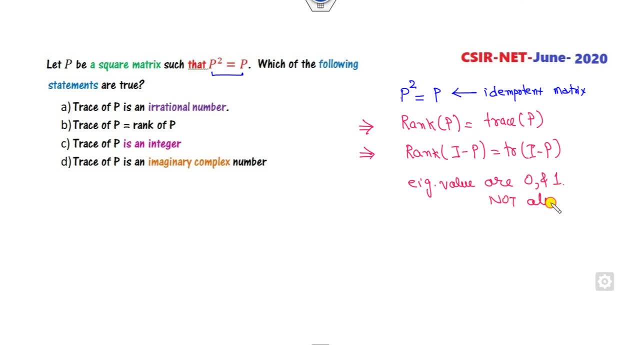 But not always Remember, not always Why? Because if I simply take, It is equal to I. What is that is satisfied? What is the eigenvalue of the? This is a 1: 1.. So that's why this is not for the, not always fine. 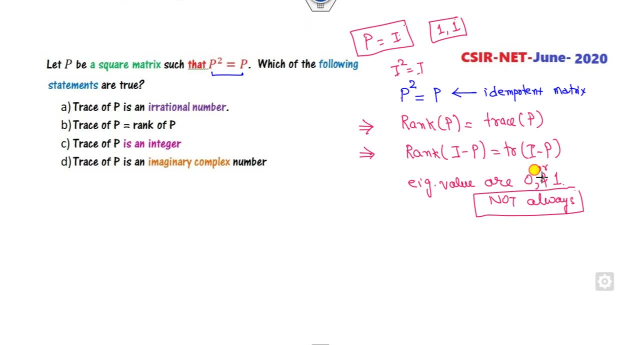 So either 0 or 1. Either 0 or 1.. Now look at the option. trace of the p is irrational number. So what is? that is either the 0 or 1. But the trace will be either 0 or 1.. 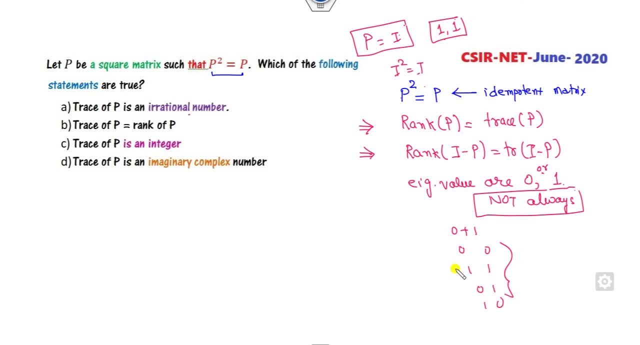 Both are 0, both are 1 or 1 0, 1 are. So in this case, trace will be the rational. So first option: cancel. This is my property. This is the tips for you. This is a satisfied trace is an integer. 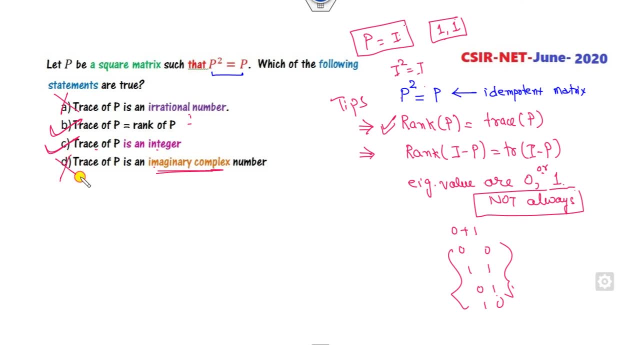 That's true. Trace is an imaginary complex number. That's a wrong option. This is a. So if somebody asks you the trace of I minus p, that's also the correct answer. So B and C are my correct options. OK, A raise to power 20.. 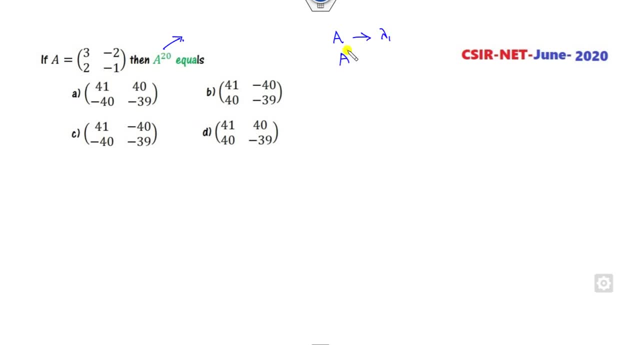 Again, if I found the eigenvalue of the A as this, eigenvalue of this, as Remember, whenever there is a matrix given to you, then always try to find the eigenvalue. So either you can write as a determinant equation, but you can see the column sum is: 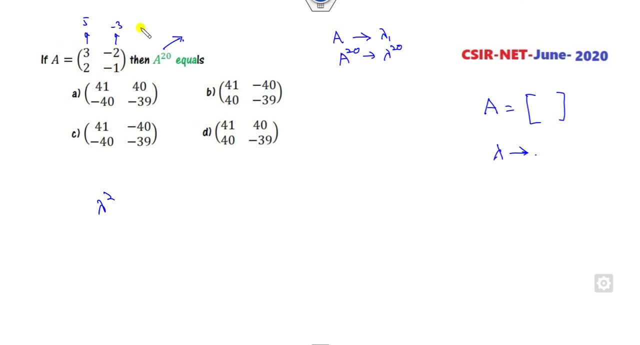 5 column sum is minus in, or same row sum is 1, row sum is 1.. So you can see: row sum is my same, same is 1.. So 1 eigenvalue is my 1.. So since it's a 2 cross 2, the trace will be my 2.. 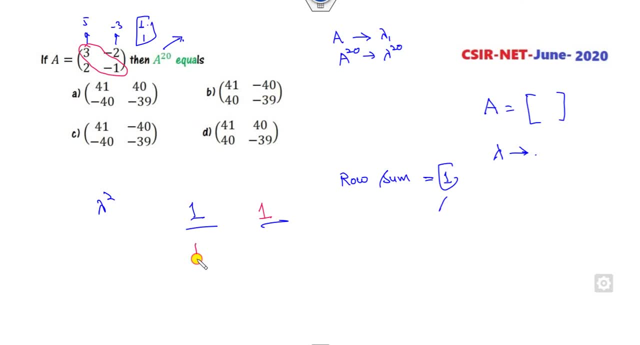 So other eigenvalues also be a 1.. So if it is here, so you can see what is the eigenvalue of the A 20. It is also be a 1 comma 1.. So we can check firstly the row sum, not 1 row sum 1, 1.. 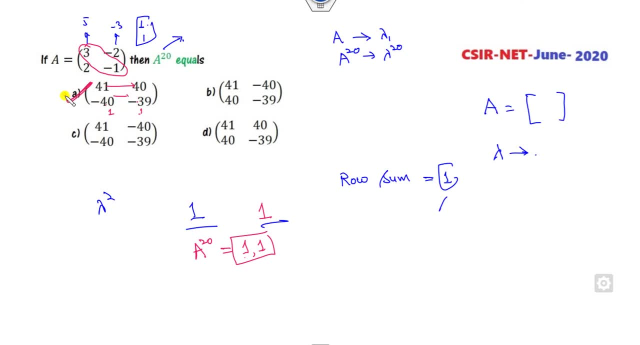 You can see it's a 1: 1.. So 1 eigenvalue will be 1, is this right answer? And, moreover, other eigenvalue trace will be my 2.. So 1 eigenvalue is 1. trace is here. This is my plus 1.. 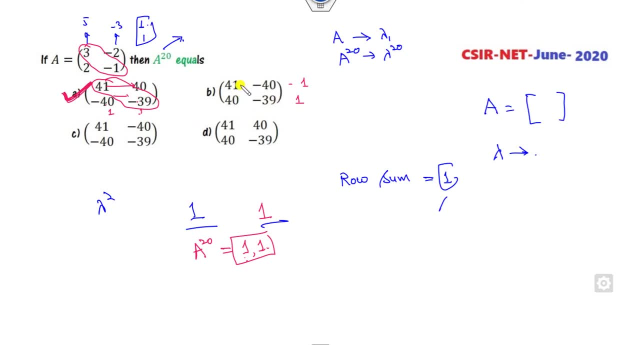 This is my plus 1. that's here, So, but trace f is my 2, that's also there. This is my 1.. This is not 1.. This is 1.. This is not 1.. This is not 1.. This is not 1.. 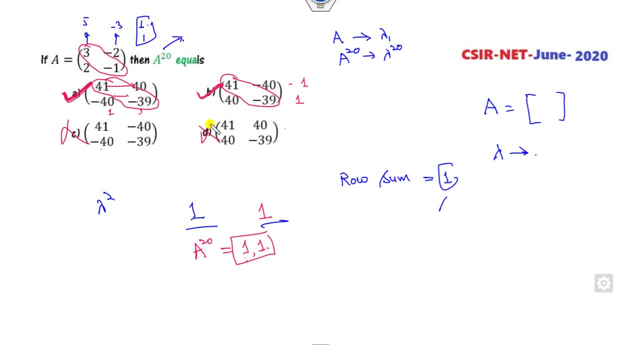 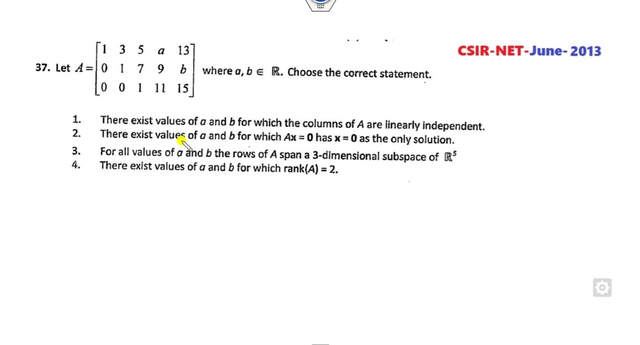 So I think both are the correct options of this problem. You can see two options are my correct. one, Trace, is 1.. Column is 1.. So 1 and 1.. Okay, look at this system. Ax is equal to b. 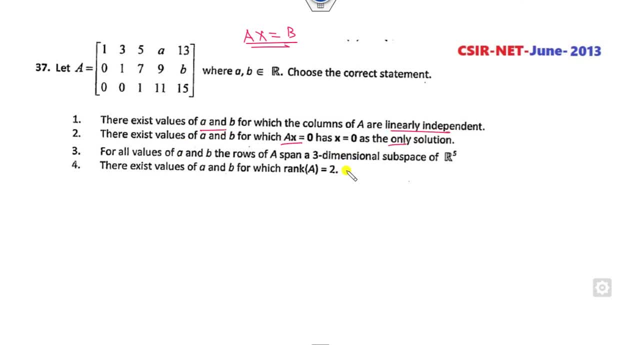 There exists a, b linearly independent a b. no solution are here. Okay, fine, This is a 3 cross 5.. So first property rank is always be less than of the number of the rows, number of the columns, It will be less than equal to 3.. 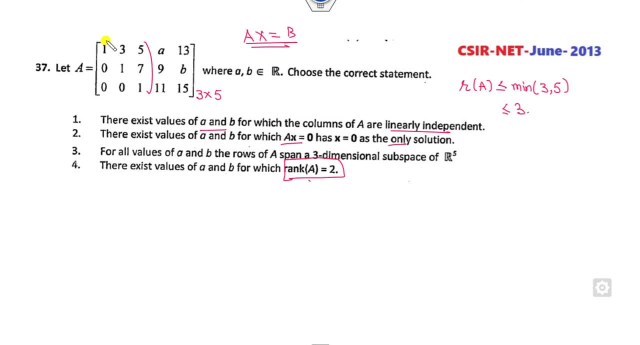 The last one is: rank is 2.. But you can see there is at least one minor whose determinant will be non zero. So rank of this matrix is always be my 3.. So third option is cancelled. So once the rank is my 3, what is the meaning of that? 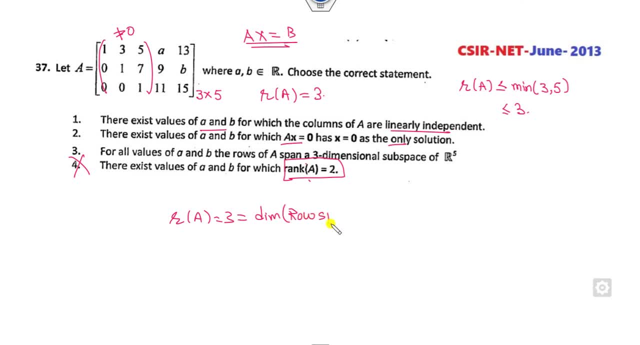 This is my dimension of the row space, as well as dimension of the column space. So if you look about this third option for all the values of the a and b, the row space has a three dimensional subspace. that's the correct statement. If it's a three dimension, then it means it's a rank is my 3.. 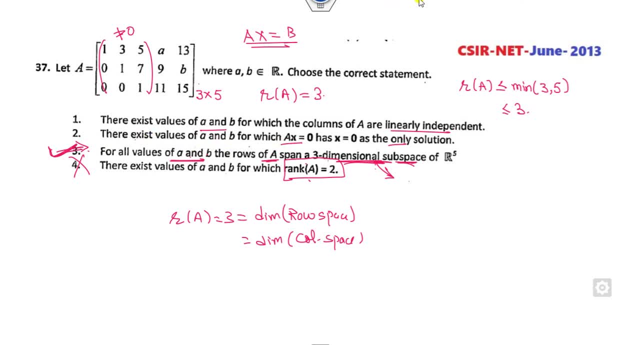 There exists a value of the a and b such that ax Is equal to 0, x is equal to 0, is a solution. So when it will have a solution, then rank of a. rank of this is my number of the column vector. Column vector is my 5, but this is my 3. 3 is not equal to 5.. 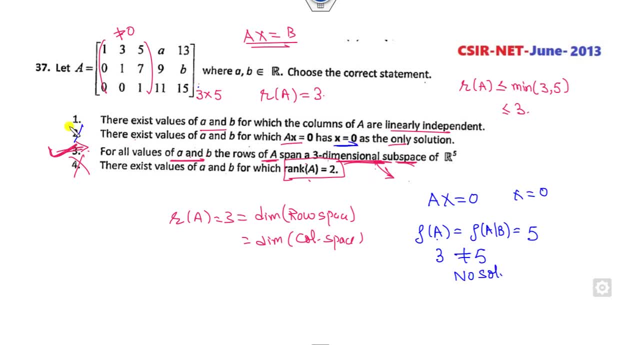 It has no solution. but he said it's a solution, it's a cancel out, For there exists a value of the a and b, for which columns of the a are ally, columns of the a are ally. But When you there exists a value of the a and b, for which column of the a- and there is, there does not exist a and b. 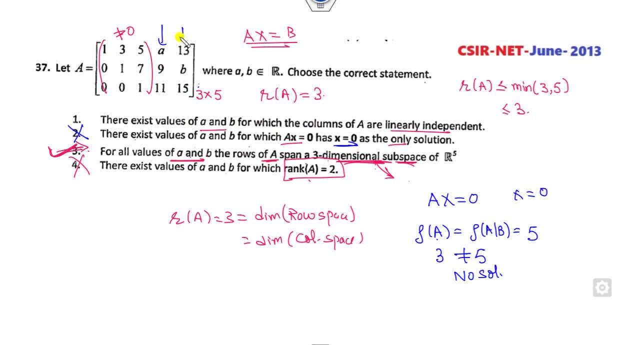 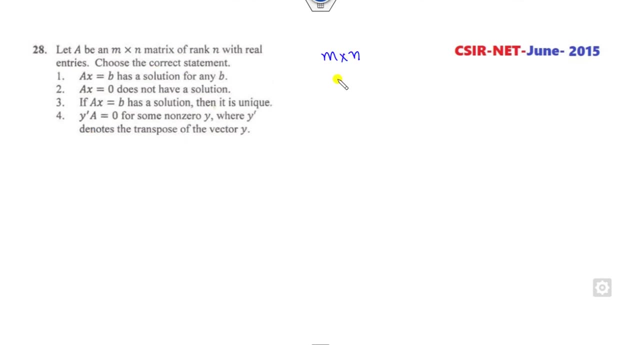 How? because the rank is my 3, so it means this value must be a- 0.. So there is no pair of the a and b for which columns are ally, So this means these are cancel out. right option is third option. Okay, a is my m cross n. 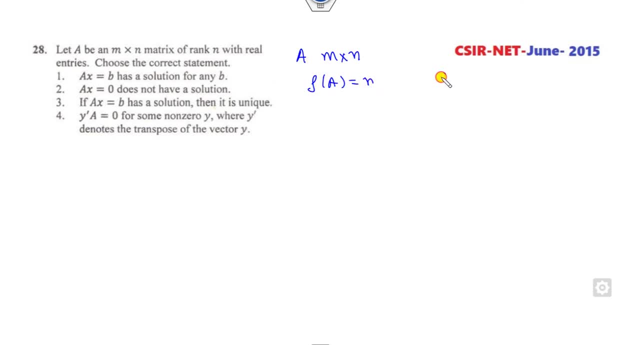 Rank of the a is my n, So I already told you Rank. if it is a m cross n, it must be less than of the m cross n. It is given that it has a rank n. What is the meaning of that? n has less than value. then which of the following is the correct statement? 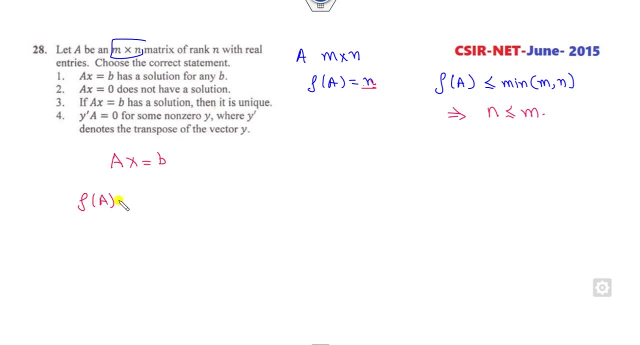 So a, x is equal to b. It has a solution when rank of this is same. here has a solution, either the unique solution or infinite solution. in each of the case It must be equal to the number of the Column vector. column is my. n for the this case is here and for this case is not equal to n. rank is my. 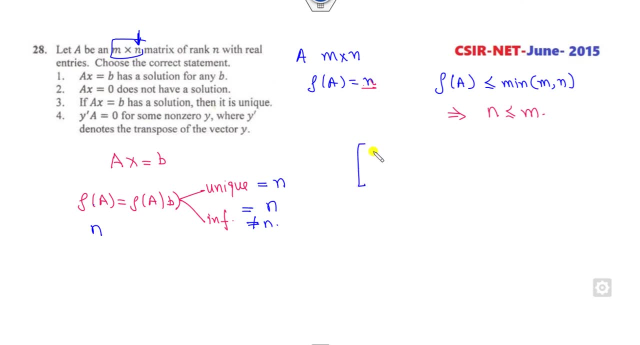 And what is the rank of the a cross b. so you can see these are the values. What is that? this is my m cross n. So if this has a rank m, this has a rank n and n must be less than of this. it means the last value must be 0 and for any b, 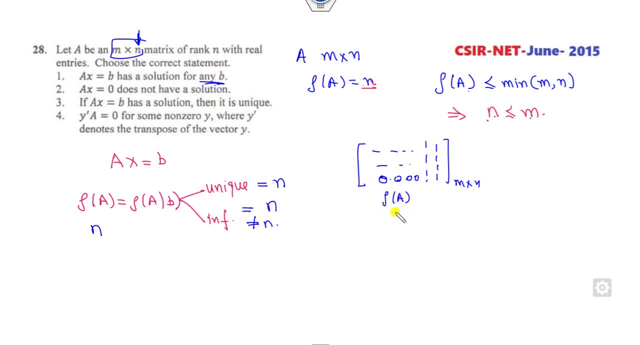 If I simply take the b as my here, what is the rank of this n? Rank of the a condition? b is my m because of this non zero elements, both are not same, so it does not have a solution. A, x is equal to 0, does not have a solution. 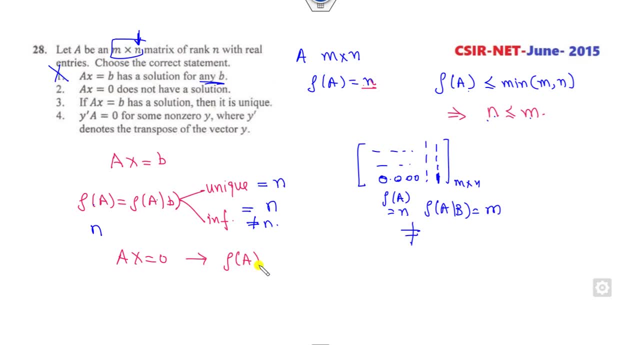 A x is equal to 0 when it have a solution, when the rank of the a is my number of the column vector. So what is the column vector n? but it's the same. So it means it has a solution. it has a unique solution. so this option is cancel out. 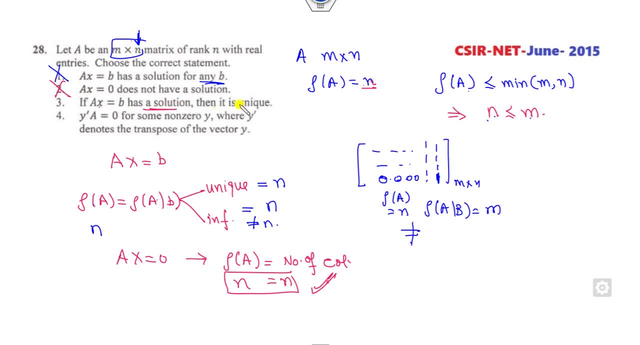 A x is equal to b has a unique solution. has a solution, then it is a solution. So a x is when it will be the solution. when rank of the a is here, it must be n. Fine, then it. then if it is there, then it is a unique solution. that's the correct statement. 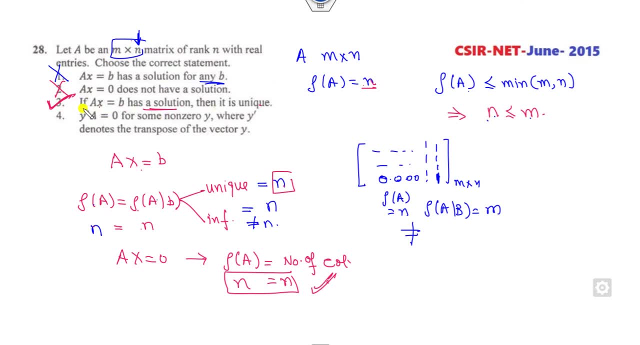 Y transpose a is 0. for some that's not true. this is only true for the symmetric matrix, Because If you have a, x is 0, if you take that transpose, This has a solution only when a transpose must be of the a. 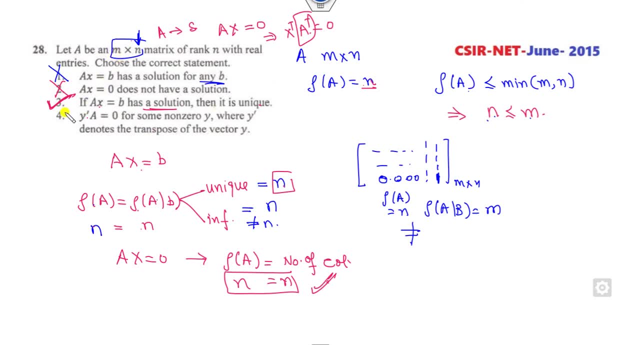 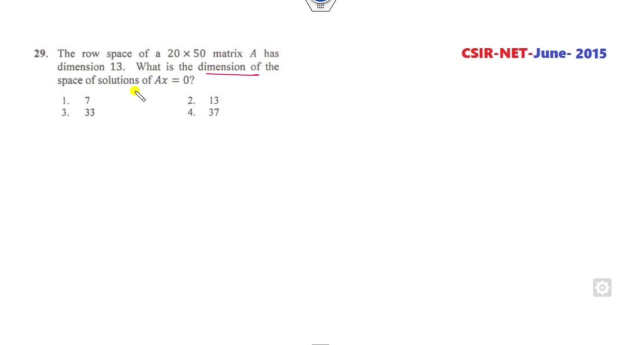 So, but a is any of the matrix need not be the symmetric matrix. So the right answer is c is the right answer. Okay, you have to find the dimension of this A. x is equal to 0.. What is the meaning of that? they are talking about the dimension of the nullity. 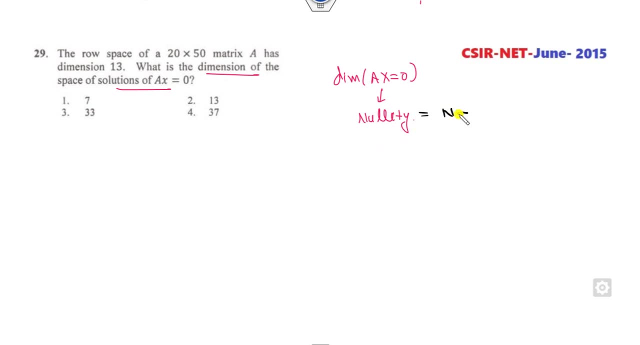 How you find the dimension of the nullity. Dimension of the nullity is my n minus rank of the a by rank nullity theorem. What is the dimension of this 20? what is the n? number of the column vectors? Number of the column is my 50. what is the rank? 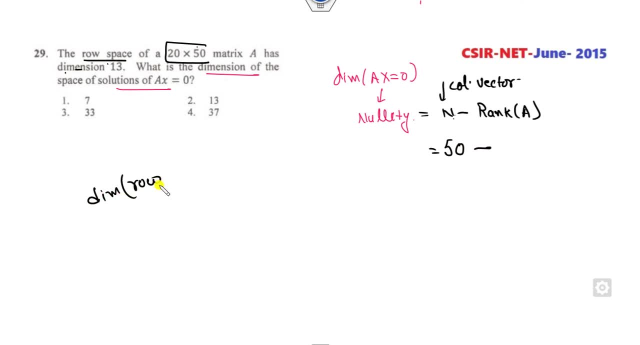 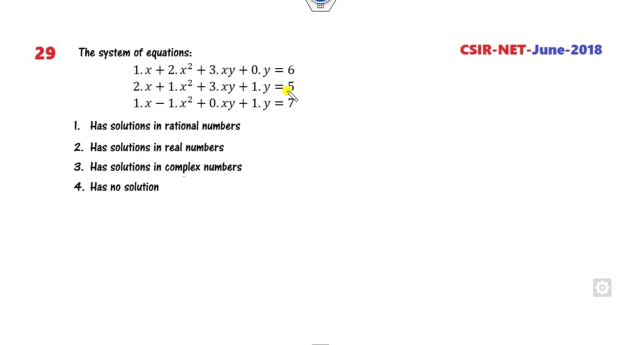 Row space has dimension. dimension of the row space: 13. what is the meaning of that? rank of the is also 13.. So right answer is 37.. So d is my correct answer. Okay, which of the following is here? So that's simply. I can write the matrix. 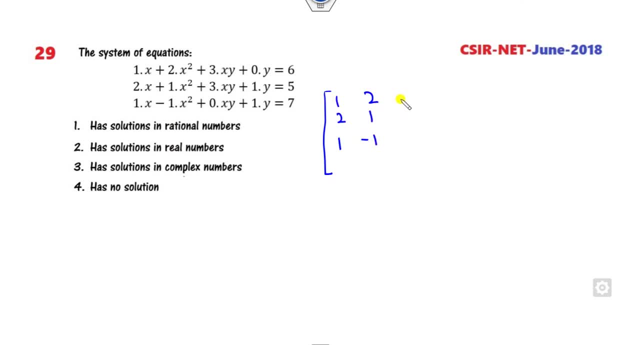 1, 2, 1, 2, 1 minus 1, 3, 3, 0, 0, 1, 1.. And this has a b Fine when it has a solution when the rank of a rank of a condition b are same. 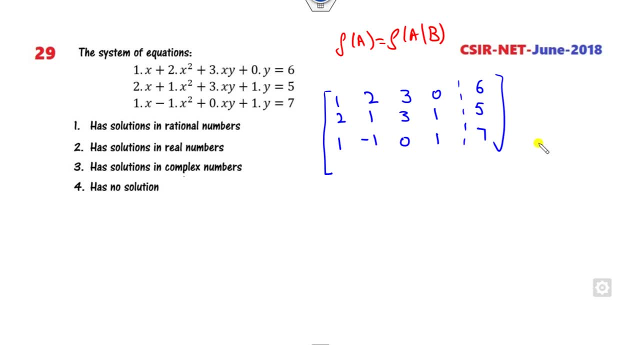 Then it has a solution. So how you can make them? I can simply take R3 minus R1.. So this number will be 0. This number will be my minus 3.. This number will be minus 3, 1, 1.. 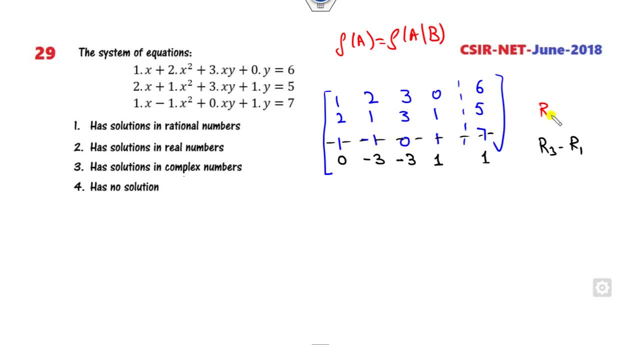 This value will be cancelled If I take 2 minus of 2 R1.. So this value will be 0.. This value will be my minus of 3.. This value will be my minus of 6.. Sorry, 6 minus 3 is a plus of minus of 3.. 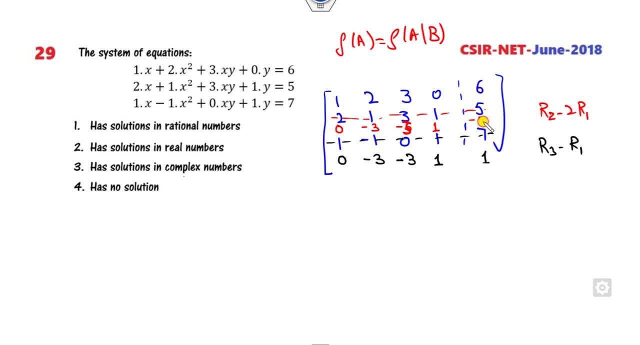 It is plus 1.. It is my. 5 minus of 10 is my minus. 5 minus 10. 5 minus 12 is my minus 7.. Now you can see, if I take now, these two rows are same, So if I subtract them again it will be 0, 0 0, 0.. 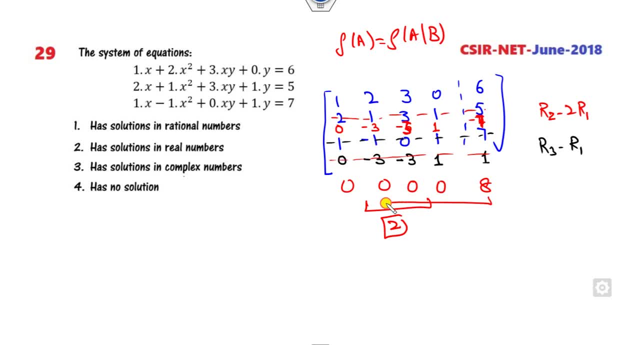 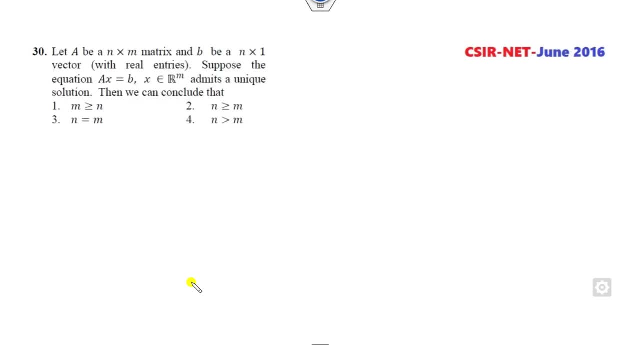 It is 8.. So this has the rank 2.. The complete has a rank 3, which is not same as the. no solution is the right, Fine. Next one is: A is my n cross m. B is my n cross 1.. 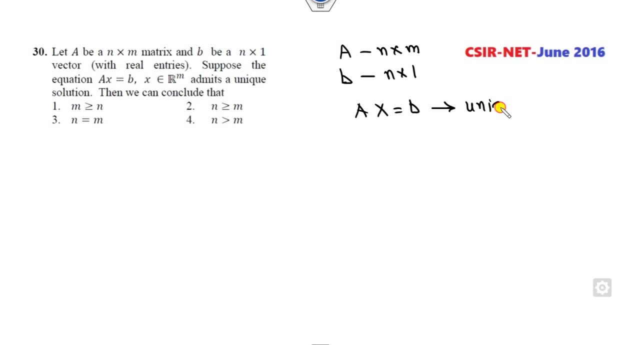 Ax is equal to b, has a unique solution. That's very simple. When it give you a unique solution, when the rank of a, rank of b, is the number of the column. vector column is here. So what is the meaning of that? Now think about here. 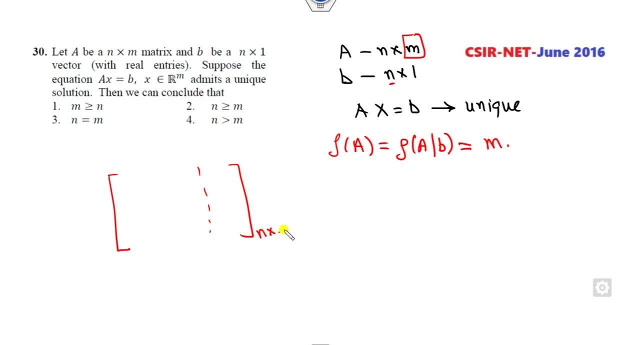 This is my b, is my n cross, 1.. So this is my n cross. So this is my m matrix. Fine, This is 1, 1, something up to here, When it will be m, when it will be m, when the last row of this must be the zero. 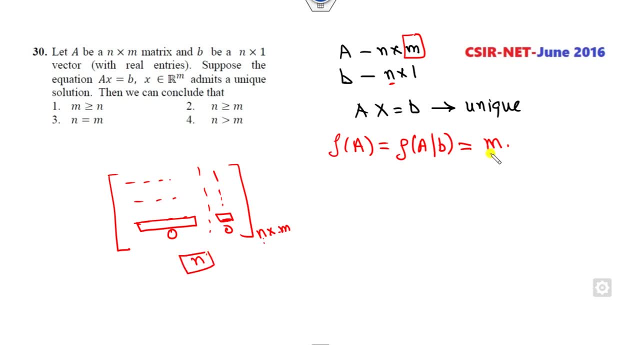 Otherwise the rank will be n, and we need a unique solution. it only it will be the m. So what is the meaning of that? The rank of this matrix will be less than of the n or n, or you can say: we need a m to be here. 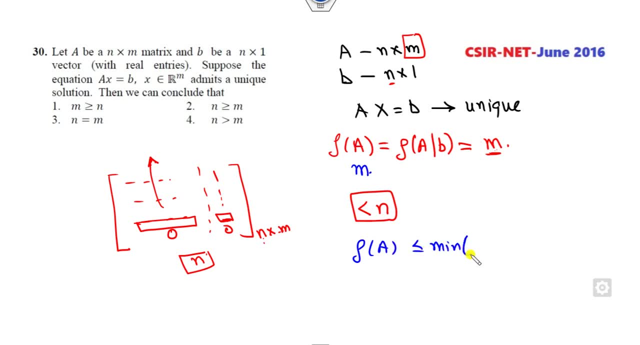 So we all knows This must be rank of the n comma m. So when it will be the m, It will be m only when your m will be less than or equal to the n. So that's the only condition given to you as of this case. 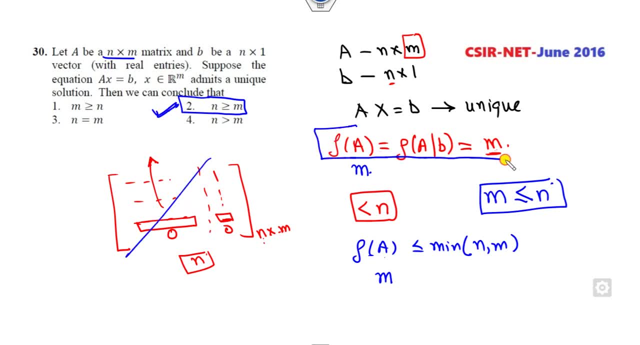 There is a simple. there is no need to write here. You can simply think about here: If a is my n cross m. by using this property, we can easily see when it will be the m. When m has a at least lesser value than of the m. 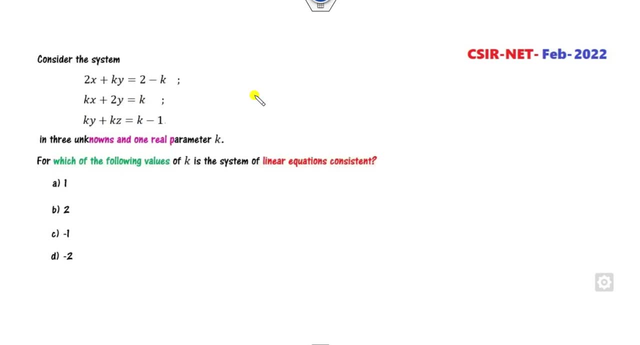 So m is less than equal to m is the right. Okay, which of the following is: the system is consistent. What is the meaning of the consistent? is unique solution or infinite many solution? That means a rank of a, rank of the a condition. b is number of the column vector. 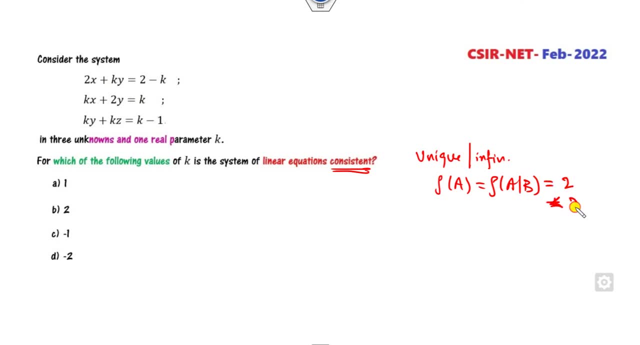 is 2 or less than of the 2, but it must be same. So how you can solve such kind of the case, There is no need to write the rank. I think about that. Firstly, I can take k is equal to 2.. 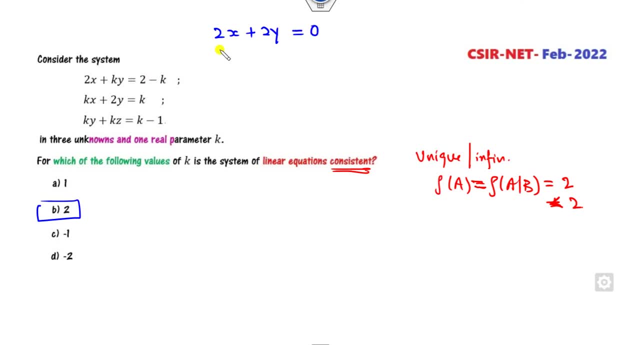 The solution will be: 2x plus 2y is equal to 0.. Second value is: 2x plus 2y is equal to 2.. Is it possible? The first give give you a 0. second, give you 2. that give you a no solution. 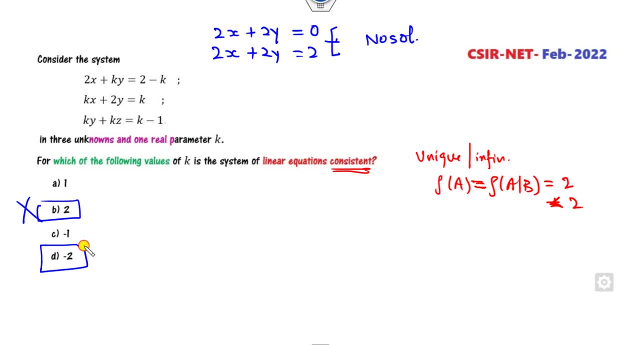 But we need a consistent. This option is cancelled. Look at the minus of 2.. The first one is 2x minus 2y is my 4.. Second is minus of 2x plus of 2y is my minus of 2.. 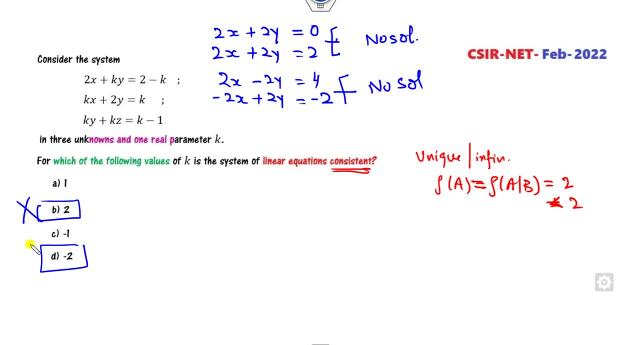 Let me say that again. It will give you no solution, So this option is also cancelled. Look at the first option, when k is equal to 1.. So it's a 2x plus y is equal to 1.. It's a x plus 2y is equal to 1.. 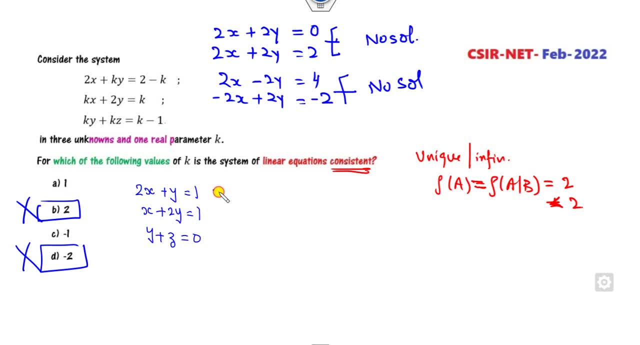 It's a y plus z is equal to 0. Now, from these two, you will get a value of the x. There is no need to find the value of the x, because they are not talking about the. what's the value of x. you will get the value of the x. 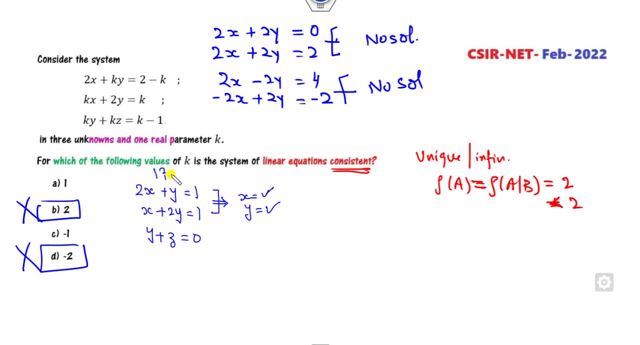 You will get the value of y, because you can see that determinant of this is non-zero. So you will get the unique value of the x and y. Once you know the unique value of the y, you can substitute here. You will get the unique value of the x. 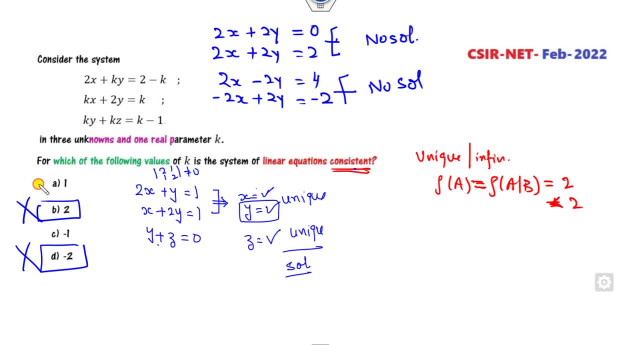 So it means it has a solution that is a consistent. So this is the right answer. Now look at this third option: minus 1.. If you substitute here 2x minus y is equal to 3, minus x plus 2y is equal to minus 3.. 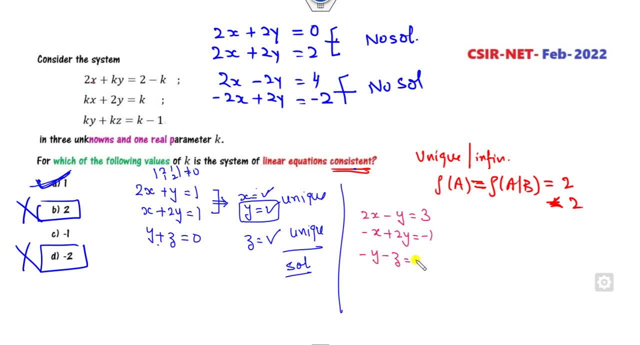 This one, y minus y minus z, is equal to minus of 2.. Again, you can see that determinant will be non-zero. So you will get the value of y. You will get the value of the x as a unique. Once you get a unique here, you can substitute here: 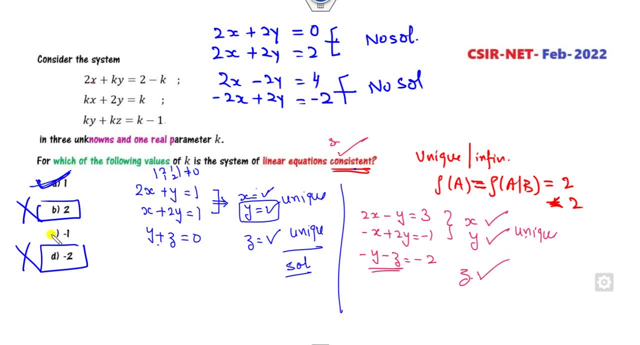 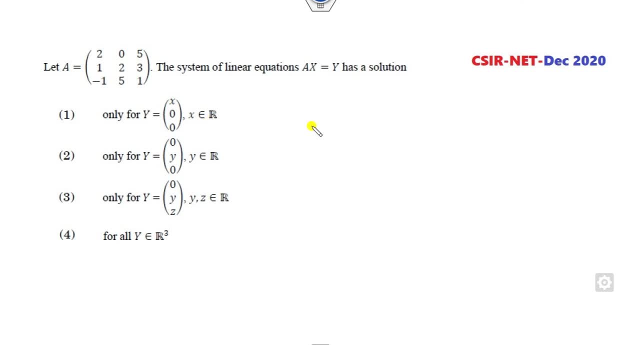 You will get the unique of the z also. It means it's a solvable. So the right answer is a and c. both are the correct answers. Okay, which of the following has for all the values? So when, When the rank of A, rank of B is, number of the column is 3.. 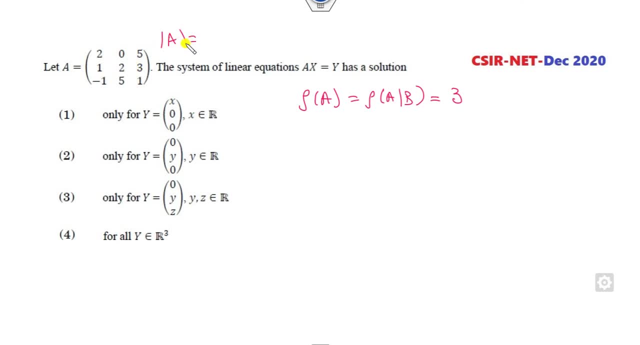 Fine, So we can check the determinant of A. What is that? 2 times 2 minus 15 minus 0 plus 5, 5 plus of 2.. So it is a 13,, 26,, 7, 35, which is a non-zero. 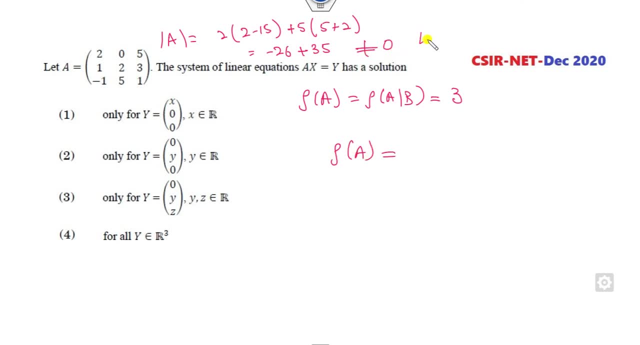 So what is the rank of the A? Once the determinant is a non-zero, it means they are allies or the rank will be my 3. It's satisfied, So it means it has. It has a unique solution. So unique solution for all the pairs of this. 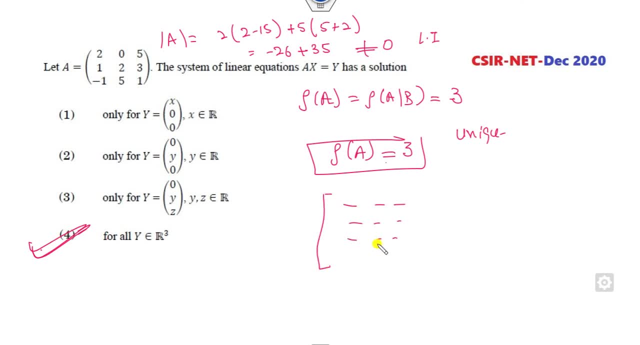 Why? Because if this is my matrix and this is my y1, y2, y3. If this has the rank 3.. If this has a rank 3, whatever the value of the y3, the total will also the rank 3.. 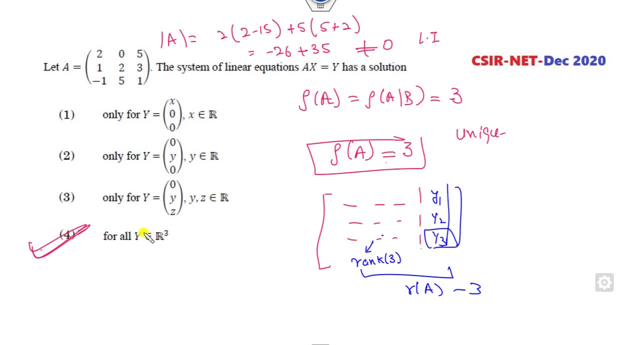 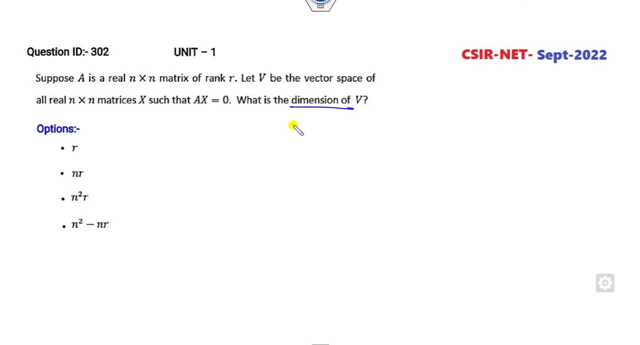 So it means irrespective of the value of the y1,, y2,, y3.. It has all the solutions. This is the right answer. Okay, So you have to find the dimension of the V. What is the V? V is the vector space of all those n cross n matrix, such that ax is equal to 0.. 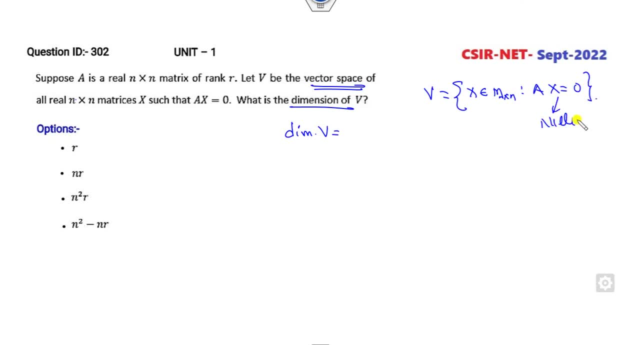 Okay, So this is my nullity. Fine, So you can find, firstly the dimension of the nullity. So what is that? n minus rank of this matrix? So n is number of the column, Here n. What is the rank of this matrix A? 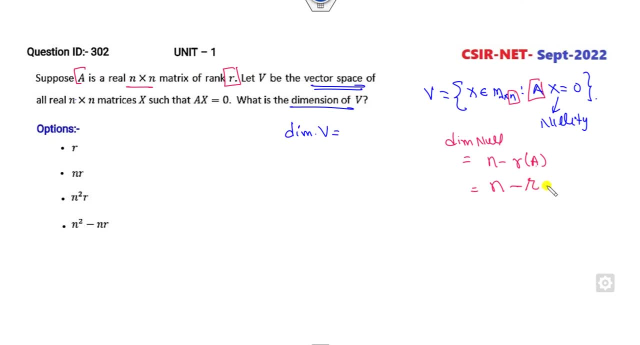 A is n cross 1, whose rank is n minus r, But this is the dimension, nullity of this. How you can find the dimension of V? V is the vector space That is nothing but number of the column vectors multiply by dimension of this. 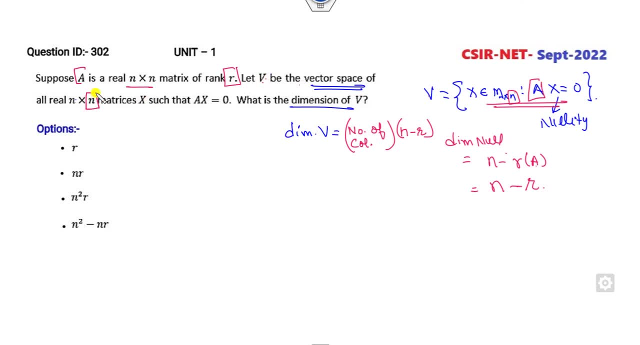 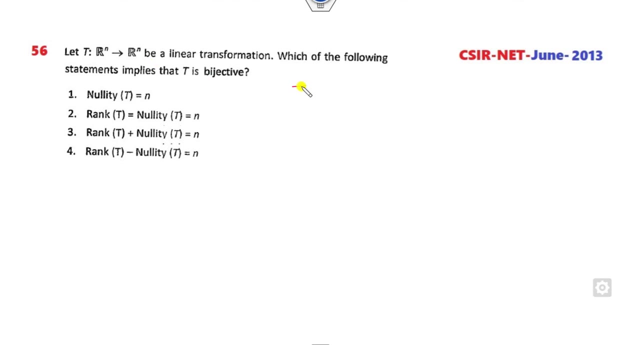 So how many? column vector of the V. What is the column vector of the V? is n, So n into n minus r, So that will be n squared n minus nr is the right answer for this problem. Okay, T is the mapping from Rn to Rn. 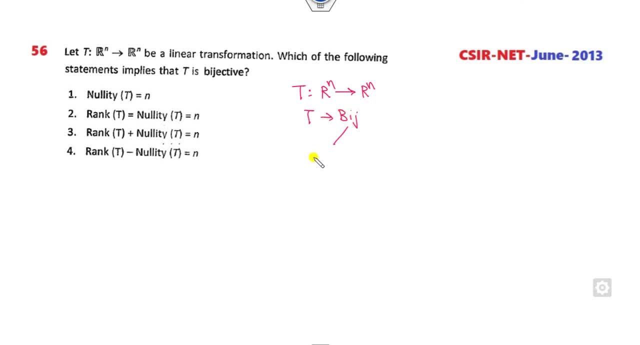 This statement implies the bijective. What is the meaning of the bijective? is 1: 1 onto. What is the meaning of the 1: 1?? 1: 1 means determinant of the matrix is a non-zero. Once determinant of the matrix is a non-zero, rank of the matrix will be n. 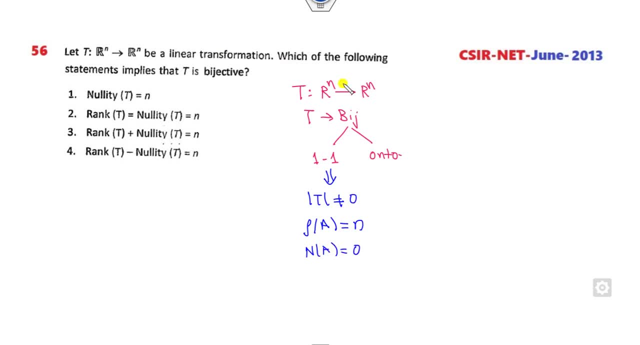 Fine, So nullity will be my 0 by using the rank nullity theorem. So check that Nullity will be n. cancel. Both are same cancel. n plus 0 is 0.. n plus 0 is n. satisfied. Both are satisfied. 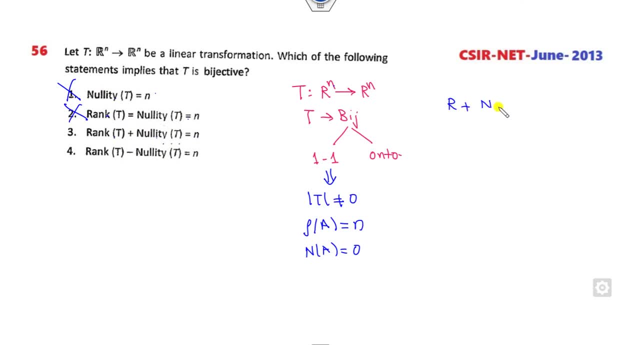 Now, rank plus nullity is my here. This is for all transformation. But whenever this is onto, what is the meaning of that Rank? What is the meaning of the onto Rank minus nullity will be here Or you can see for the nullity. 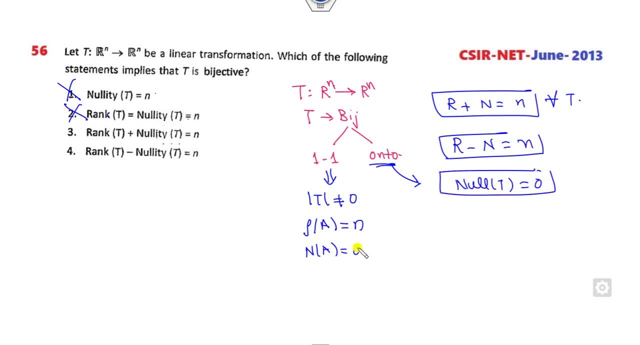 Of this will be 0. So once nullity will be 0 here. So if you simply add them- because this is a general statement, if it is there, So you will get, as cancel out is the right answer. This is for the journal one. 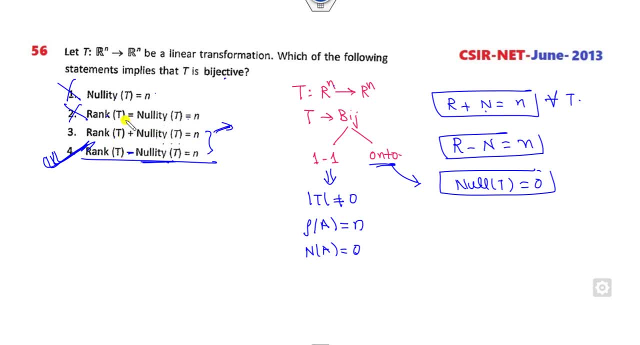 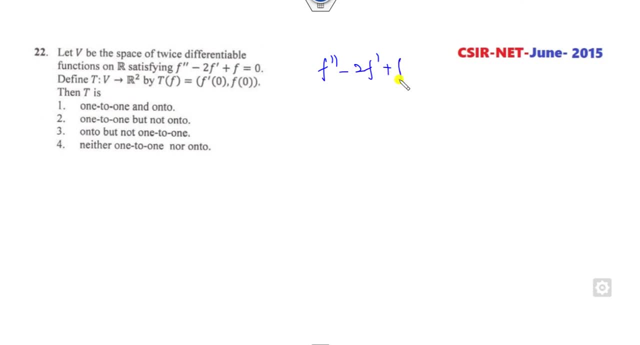 But once is bijective, then it will be the minus of the n. Okay, Look at the next example. V is the vector space of this. So I think that's a very simple. You can simply solve this one. M will be my 1 comma 1.. 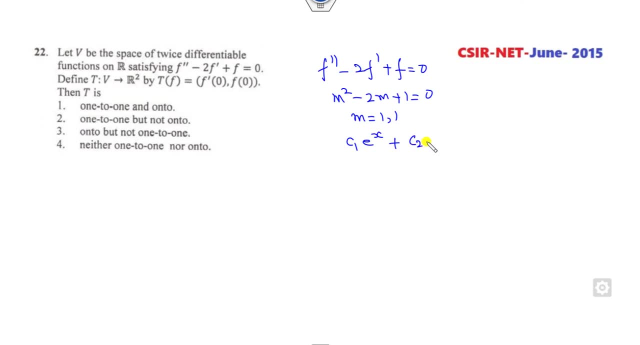 So solution will be here: plus c, 2 x, e raised to power x. So what is that? This is my f. Now you can take the derivative f 1 c x, c 2 x plus 1 of e x. So what is the my transformation? 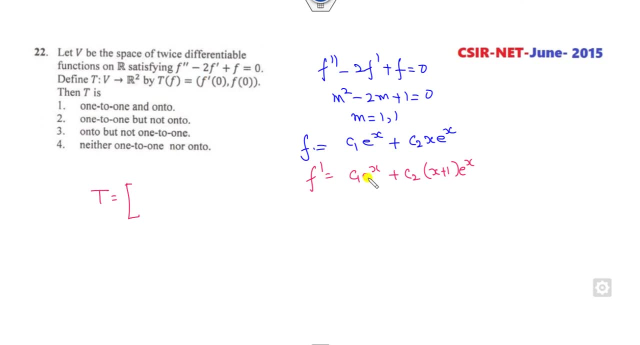 f 1, f dash at the point 0.. So this is my c 1.. So c 1. Plus it will be 0: 0. 1 is here. What is my f of 0?? This is 1.. This is 0 on this c 1.. 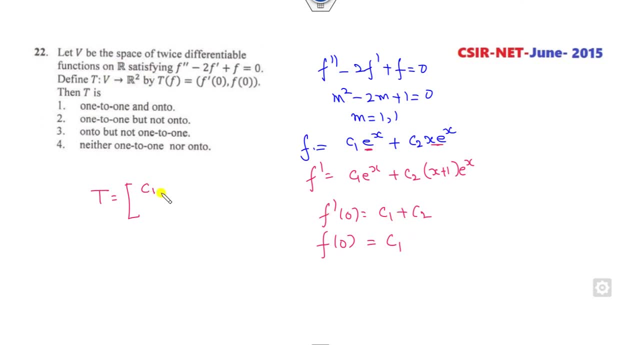 So, since it's a transformation, we can write the vector as a column. So c 1 coefficient of the c 1 is c 2.. So 1 1 1, 0.. This is my matrix T. Fine, Now you can clearly see that determinant is a non-zero. 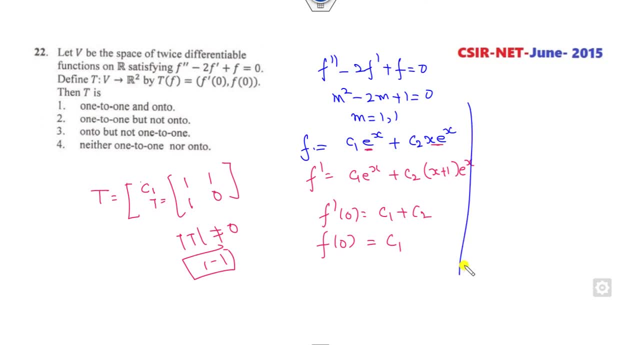 So it's a 1, 1.. Then how you can check whether it's onto or not. So corresponding to the each pair, a comma b, If I take this pair as c 1 plus c 2 and c 1.. So c 1 plus c 2 and c 1.. 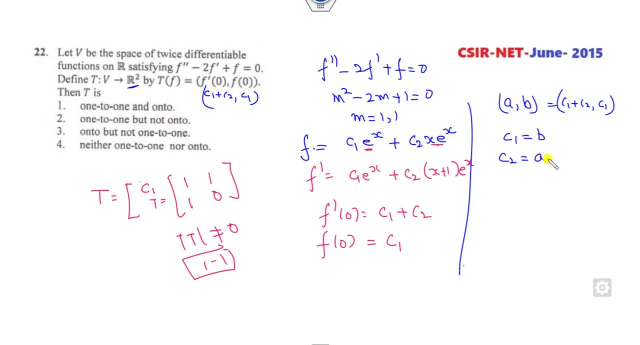 So clearly see that c 1 is b. c 2 will be a minus b, So I can substitute here: This is b, e raised to power x, a minus b, e raised to power x. So for each pair of the a comma b there exists a function. 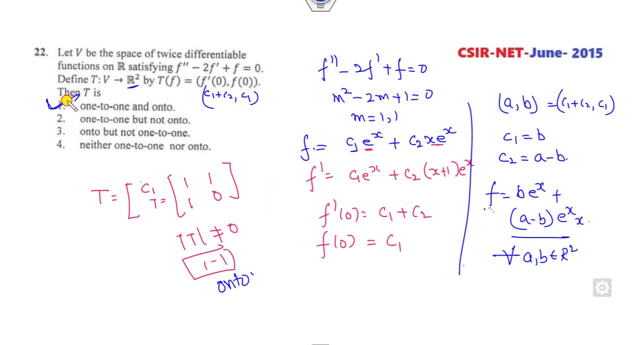 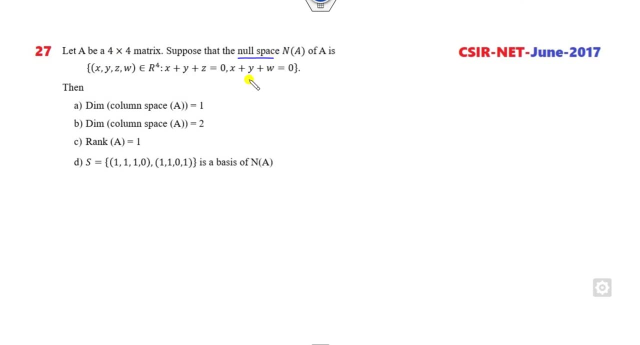 So it is onto as well. So that is a bijective Rest. all are Okay. A is a 4 cross, 4.. Null space is given to you. You have to find the dimension of the null space. How you can find the dimension. 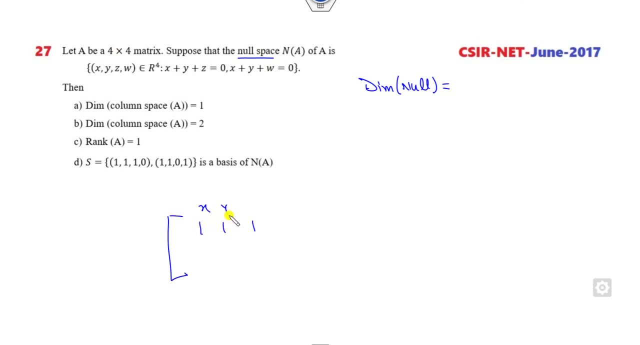 The first method is you can write in this form: x, y, z, w, x, y, w here and write in the row reduce. But there is no need Look at that. Check about the nullity. dimension of the nullity means That is free variable. number of the free variables. 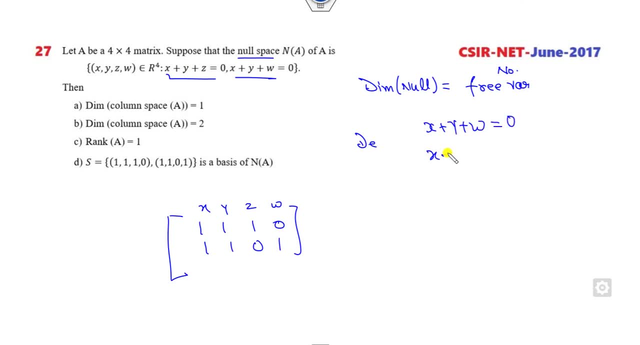 So in the first line Here and in this line, x plus of this, x and y are my dependent variable. w and z are my free variables. So it means how many number of the free variables 2.. So that dimension is my 2 and the dimension of the null space is that is a nullity, is my 2.. 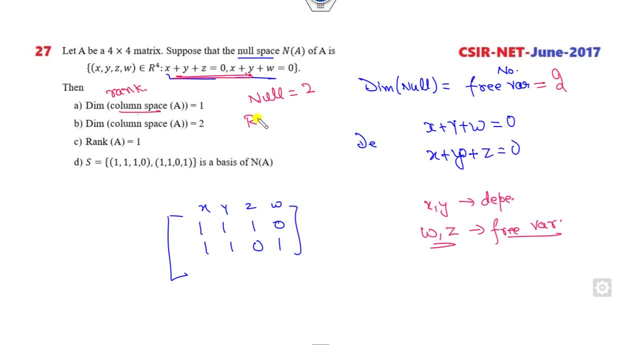 But he said dimension of the column. That means they are talking about the rank. What is the rank column vector 4 minus 2 is my 2.. So dimension of the column space is my. 2 is the right answer. So rank is 1. cancel this cancel. 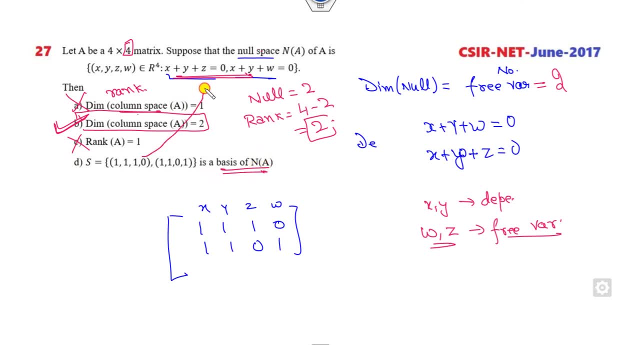 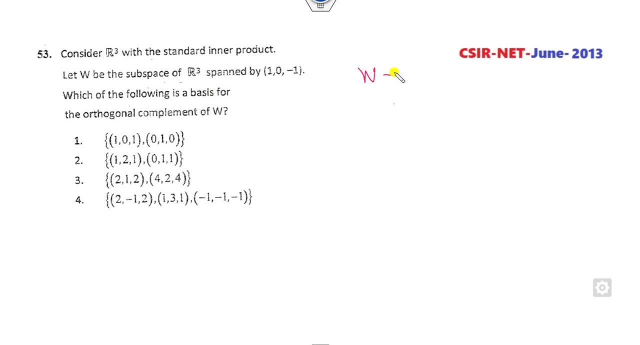 Is it the basis? when? it will be the basis if it satisfied. here check: is it satisfied? No, So the right answer is only because this is the basis of them, It must satisfy this condition. Okay, So r3 is the inner product space. w is spanned by 1, 0 minus 1.. 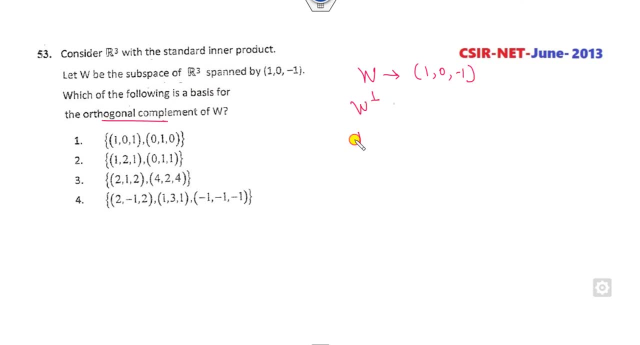 Which of the following is the subspace of the orthogonal? So remember, we all knows the orthogonal properties. dimension of this is my n. What is the n is 3.. So dimension of w is my 1.. So it must has a dimension 2, but it has a dimension 3.. 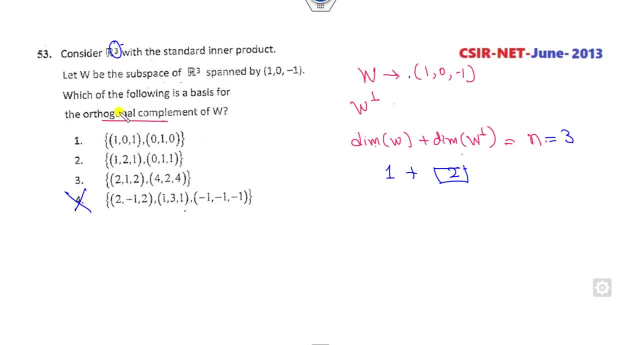 Cancel. So all are correct. Now which one of them orthogonal? What is the meaning of the orthogonal is? inner product will be 0. So check about the dot product: 1 plus 0 minus 1, 0 satisfied. 0, 1 sorry. 0 0, 0 satisfied is the right answer. 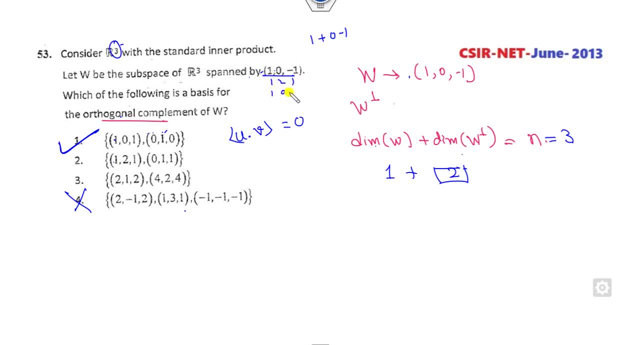 1 2 1. if you multiply them is a 1, 0 minus 1 satisfied 0 1 0 0. 1 1 0 0 minus 1, which is non-zero. So cancel out 2 1 2.. 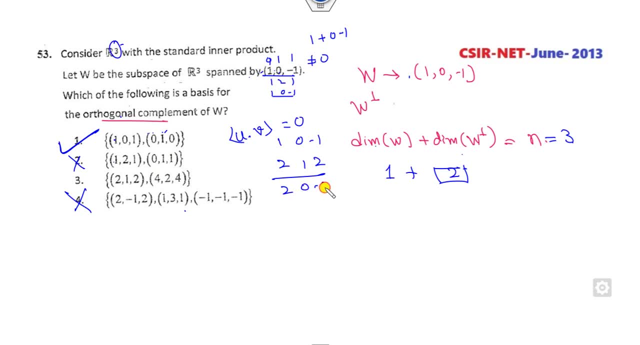 If I take the orthogonal pair of this: 2 0 minus 2 satisfied, 4 2 4 4. 2 4 4 0 minus 4 is also satisfied. So this is also the right answers. So right answers are first and the third are the correct options of this example. 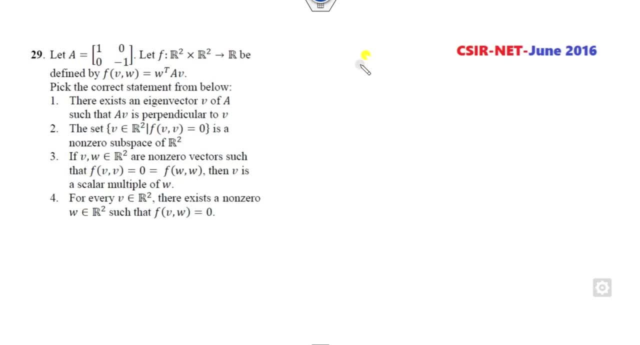 Okay, Look at this one. A is my 1 0, 0 minus 1.. F is my here. Fine, I can also return this as, or because this is a symmetric matrix. Okay, So I can also return this in terms of the inner product, fine. 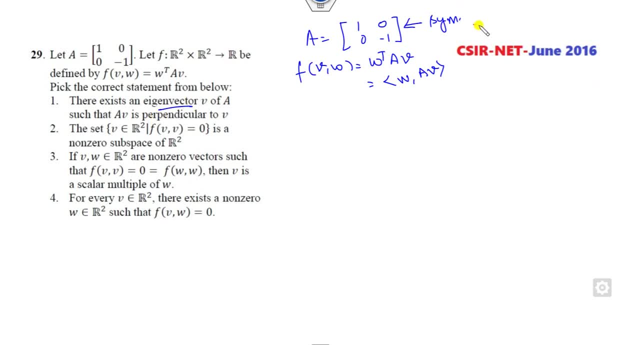 There exists the eigenvector of this. So, firstly, we can check about the eigenvector. eigenvalues are 1 and minus 1.. So, corresponding to the 1, this is the eigenvector. corresponding to 0, this is the eigenvector. 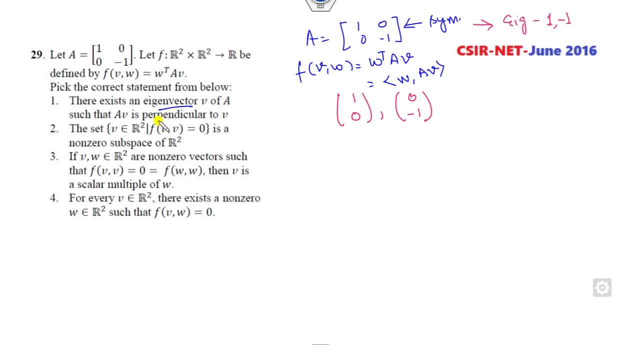 Fine, These are the eigenvector given to you. So we will check what A is perpendicular. This must be the 0.. Fine, Or you can say W transpose, that is a V transpose of AV must be 0.. So if I take about here 1, 0, A is my 1, 0, 0 minus 1 and this is 1 comma 0. 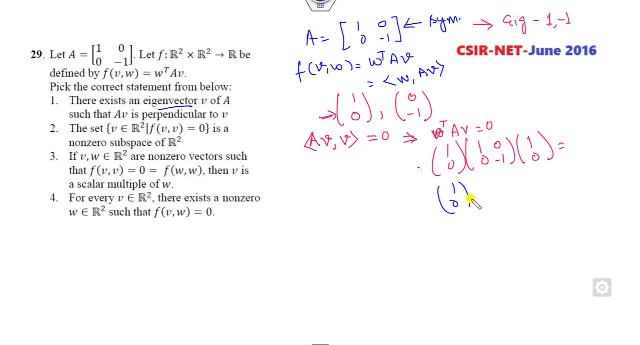 So check whether this will be the 0 or not. So clearly see that it will be 1. first value will be: is a 2 cross. 2 is a 2 cross 1.. So it will be 2 cross is a transpose. 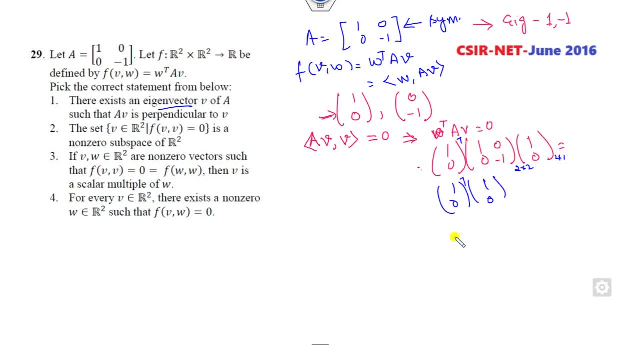 Sorry. So it's a 0 is a 1, is a 0.. So what is that? It's a 1, 0 is a 1, 0.. It's a 1, which is non-zero, But it's a perpendicular. first option: cancel out. 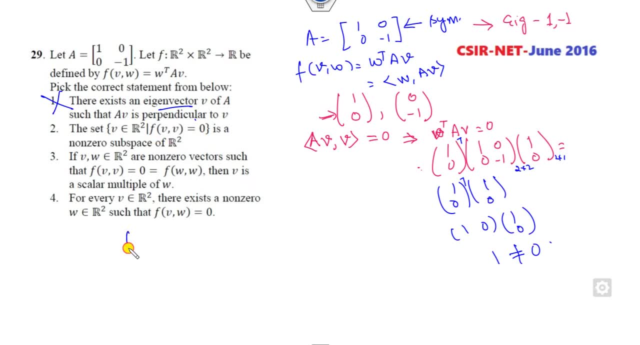 F of V is 0 is a non-zero subspace. What is the meaning of that? This is my here. What is the meaning of that? is V transpose, AV is my 0.. So if I consider V is my XY, So this is my XY is my 1 minus 1.. 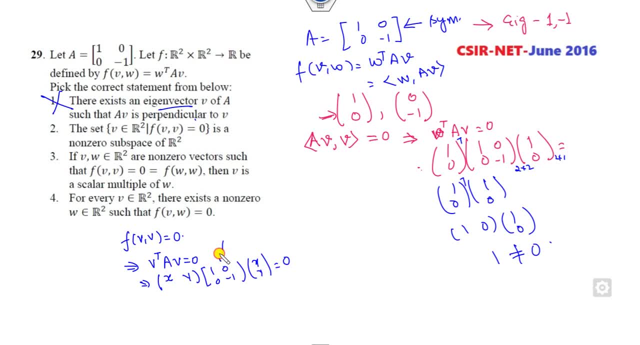 And this is my XY. So what is that? again, because of this matrix is a quadratic form, So we can write directly: This is X square, This is my minus Y square. So what is the meaning of that? X is my plus minus Y. 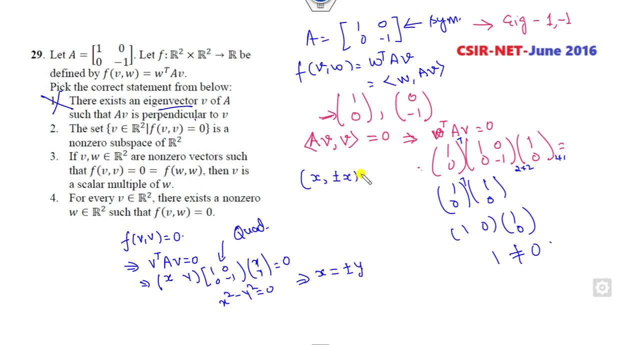 So subspace will be my X plus minus X. Fine, Now you can see 1 comma minus 1 satisfied, 1 comma 1 satisfied. But if you add them because subspace properties U plus V also belongs to them. So 2 comma 0, which is not of the form of here. 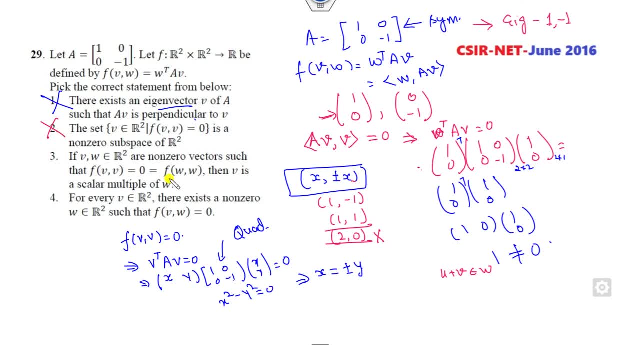 So this option is also yes. Third option is again. third option is similar to the first one. If this satisfied, it means I have the pair of X comma plus minus X. if WW is there, Then I can say it's a plus minus a fine. 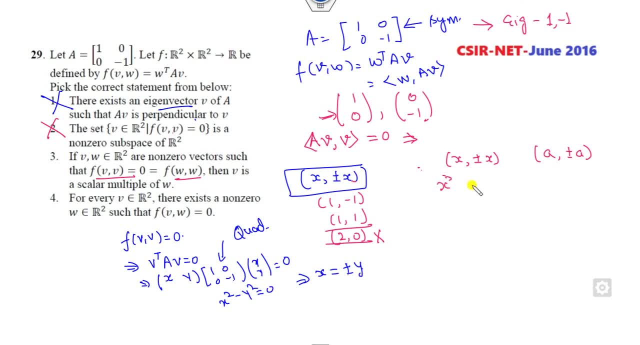 Now, what is the meaning of that? if I say this means, if I simply take 1 or 1 is satisfied, 2 and 2 satisfied, But one of them is a scalar multiple of the other. Is it true? This is true? 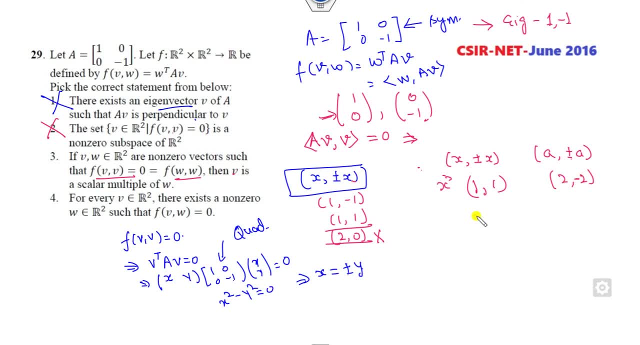 But if I second pair, I consider as a 2, and minus 2 clearly says this can never be written as the scalar multiple of the year. So it is not of this. So the right answer is: fourth is the correct answer. Okay, Look at this one. 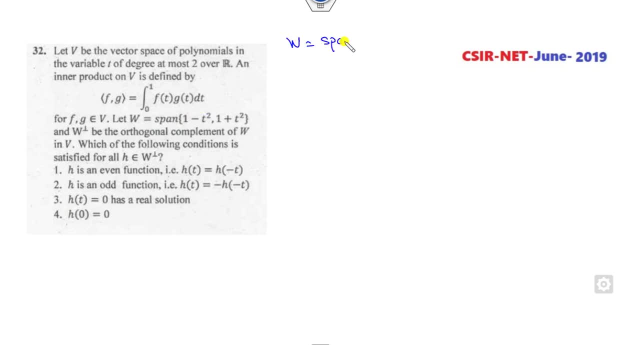 This inner product space. W is my span of 1 minus T square 1 plus T square V is a vector space of degree 2, at most 2. It has the dimension of 3.. Fine of this, W is the orthogonal complement. So which of the following is there? 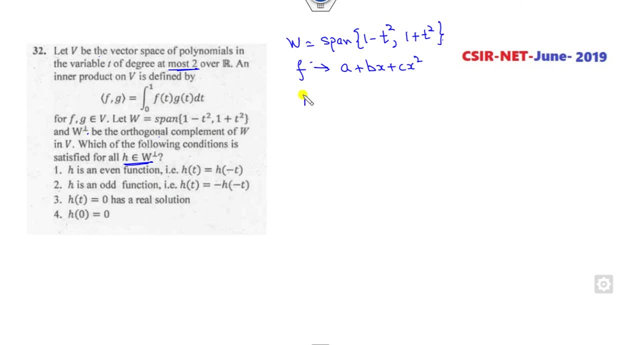 H is even And so it's a polynomial. Firstly, I can think about any of the polynomials. This is my even polynomial, So check about whether this property holds. I can take F, F and G belongs to this. If I take X here, 1 minus X here, check whether this will be the orthogonal property. 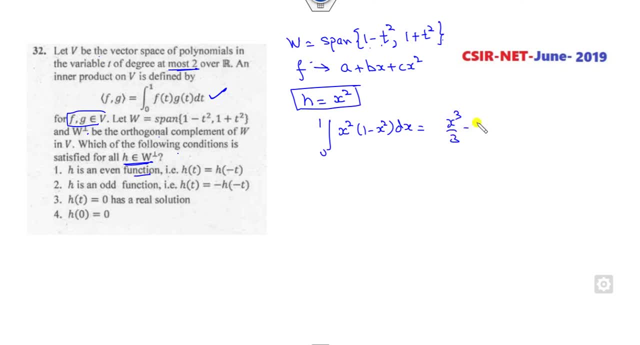 It must be the 0. So it's a X cube by 3 X 5 by 5.. So clearly says it will not be 0. So it means even is not satisfied If I simply take or function. So H is my say, X. 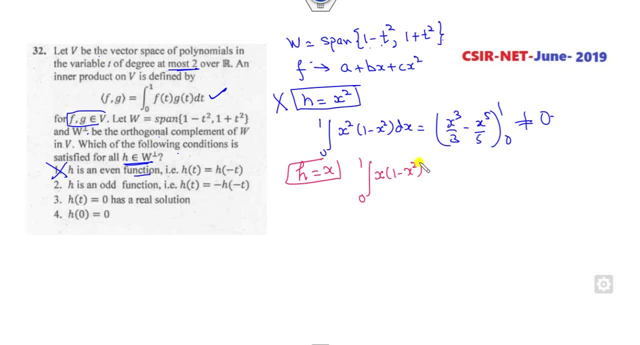 So again, this property- X of 1 minus X- here It will be X squared by 2 and it's X, 4 by 4- clearly says again It will not be 0. So this also cancel H of 0, H of 0 is my 0, H of 0 again. 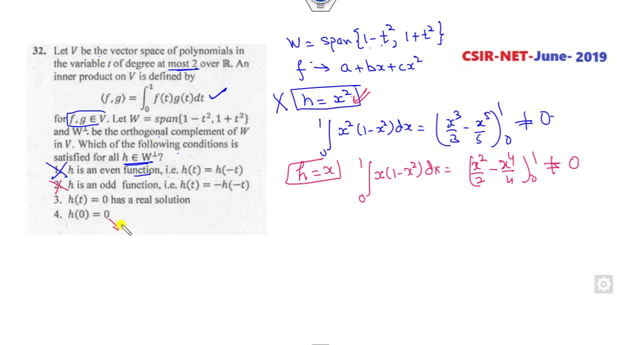 If we think about here, this is not satisfied. 0 is my even function, So this is also not satisfied. So the right answer is only C, because we discard the rest of them. Okay, look at, this is the inner product. which of the following is the inner product? 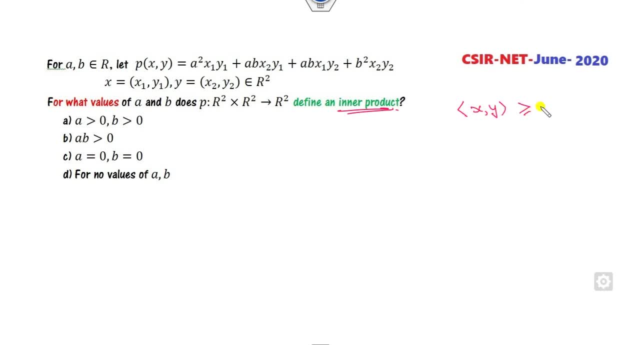 We all knows what is the property of the inner product is, it is always greater than 0.. This is equal to 0 if, and only if, X is equal to Y. Okay, which of them? so look at the option firstly, first We will see- is equal to 0. what will happen of my P? 0, 0, 0. 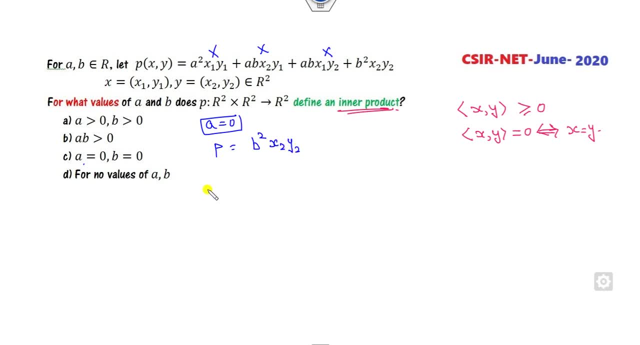 So this is my B square: X, 2, Y, 2.. So my property will be in: a product must be greater than equal to 0 for all the pairs of the R2.. Is it possible? No, because if I simply take the pair as minus 3 plus 4, which belongs to the R2, X, 2 is my minus 3 here. 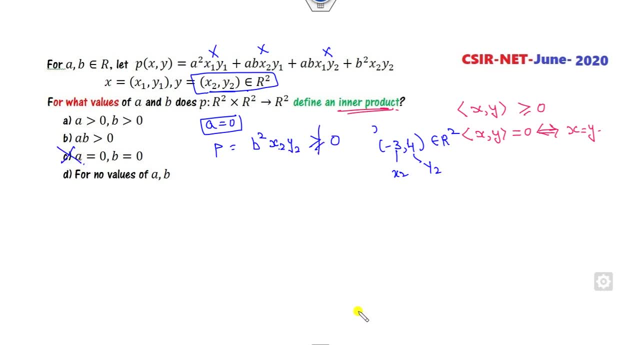 So you can see the product will Not be 0.. So a cancer, If a is my greater than 0, B is is greater than 0.. Okay, you can think about any of the number. So if I think about any of the number, okay, I can simply take: X is equal to Y means X 1 is equal to X 2, Y 1 is equal to Y 2.. 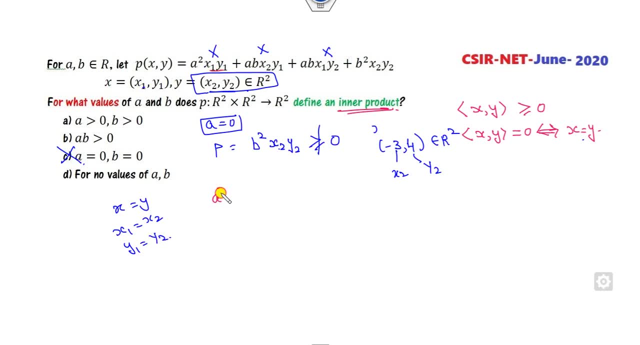 So what is the result is this will be my a square: X 1. Y 1.. This is my X 1 Y 1.. This is my X 1 Y 1.. So it's a 2 times AB- X 1 Y 1.. 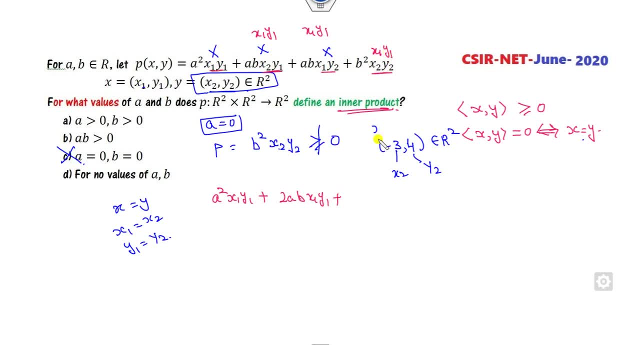 This is my X 1.. This is my Y 1. So it is my B square, Sorry. X 2 will be my X 1, Y 2 will be my Y 1.. So it's X 1, Y 1.. 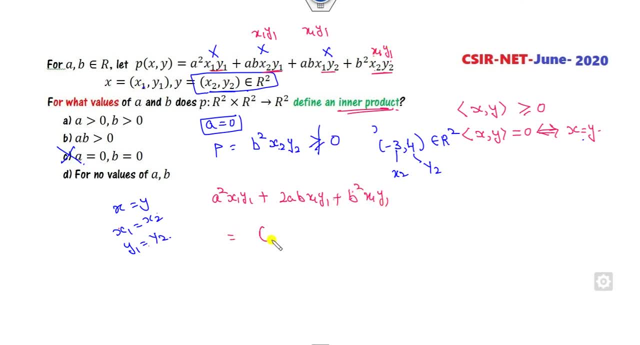 So it is my B square X, 1 Y 1.. So it is a plus B whole square X 1 Y 1.. So if I say, can it be 0 already? Always? No, it can never be 0 for different pair. 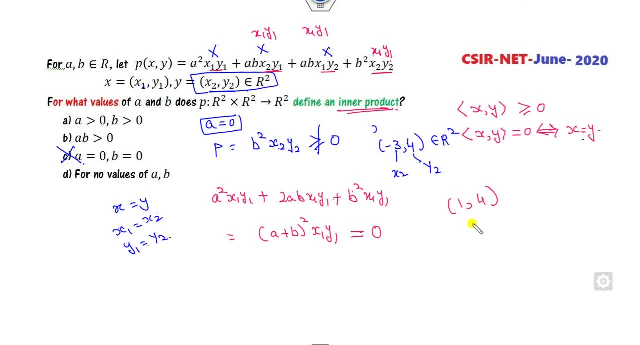 If I simply pair X comma- Y is my here and a is my greater than 0, say 10, B is my, say, 11, clearly say that it will not be 0. It will not be 0. So it will this option cancel out. 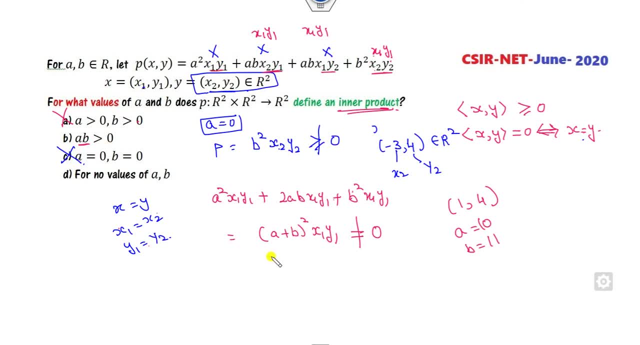 Similarly, if you look about that, AB is greater than 0, so it will be 0. if I take, a is my 4, B is my say, my minus 4.. So, product of them, This will be 0. satisfied. It will be 0 when X and Y. 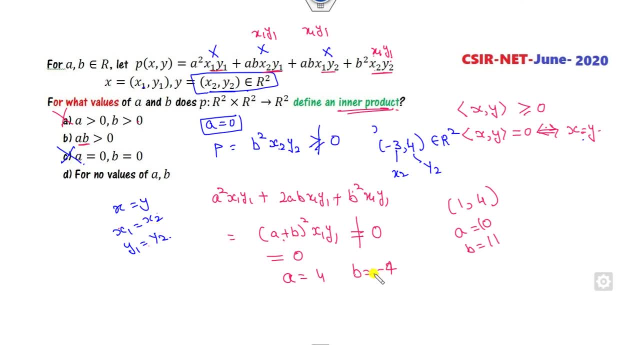 It will be happen only when A is equal to minus, A is equal to minus B, But the product is non-zero, is not be less than, not a greater than, 0. So the right answer is only the rest. options are cancelled. Look at this. another one here. 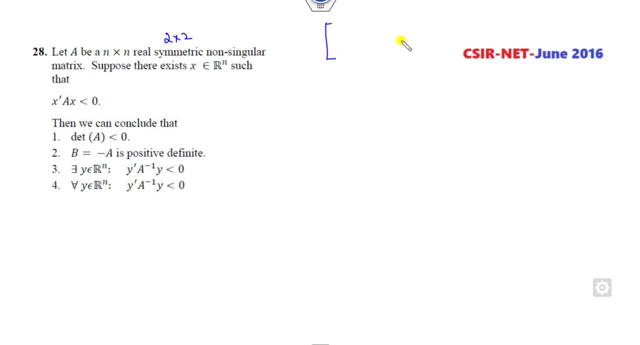 A is my Smith-Wick matrix. I simply take 2 cross 2.. Any of that, 2 cross 2 Smith-Wick matrix. So here is my. then there exists X. Remember they are not talking about that for all X. So this: if you look about this property, what is that? 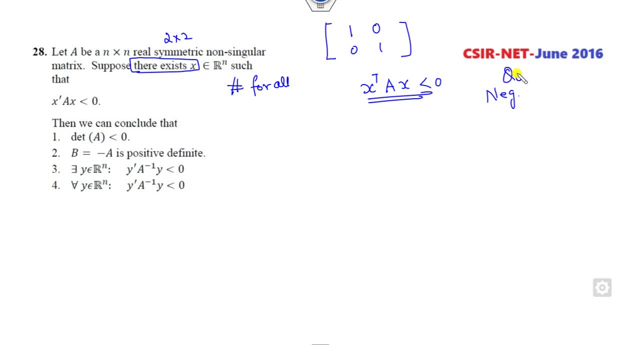 It look like say it's a negative definite quadratic form, But I, as I told you in the first two examples, if this is for all X, but it is not for all X, It means It is not a quadratic form. If you think about that, this the quadratic form, then definitely this is a negative definite and you will get the wrong answers. 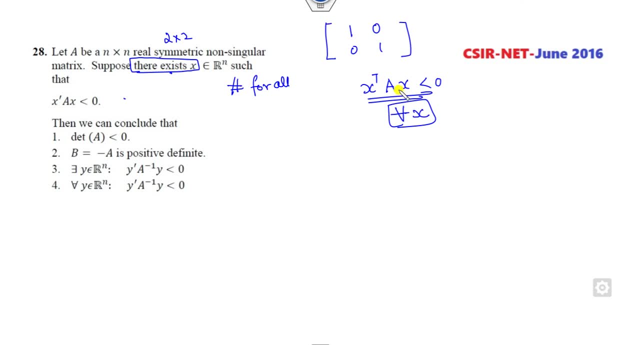 So look at that. if I consider this as Smith-Wick, if I consider this value, there exists a X such that this value will be satisfied. So what is that? if I say this pair will be here, No, this will not be satisfied. if I take this as a negative, again, this is Smith-Wick, how you can take the quadratic. 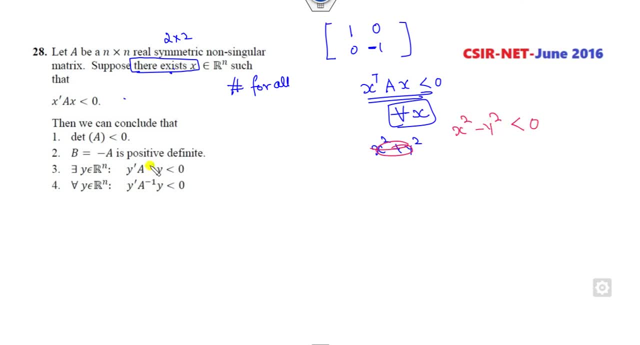 This is my X square minus Y square, It can be less than 0.. So what is the determinant of this? is either less than 0 in this particular example, Yes, it is true. Okay, but because I consider this one particular example. 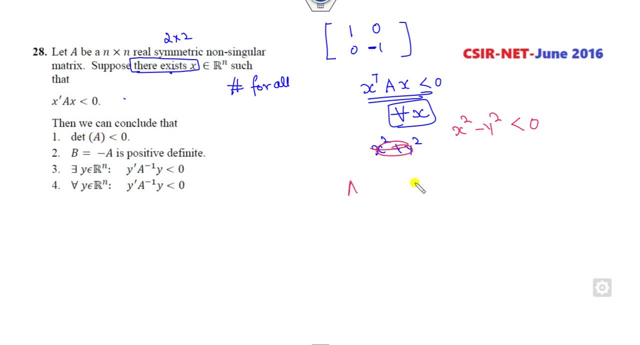 Can you think about any of the other example whose determinant will be, if I simply say minus 1, minus 1.. Fine, So now this is the quadratic form. how you multiply the quadratic form, this the a 1, 1.. So if I consider the pair as X comma Y, this is a 1, 1.. 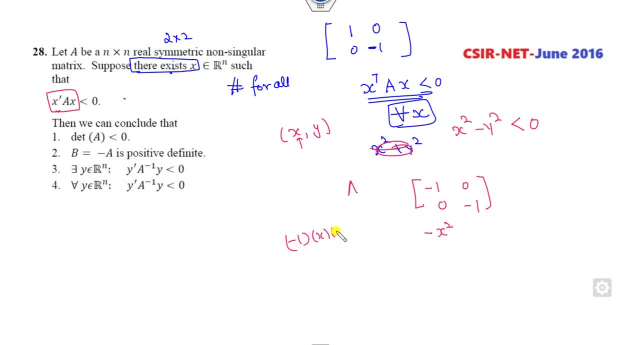 So this is the X square, like minus 1.. X- X, this is a 2, 2 minus 1, Y, Y, Y. So what is that? this is minus X here, minus Y square, which is always less than 0.. So this property satisfied for this. 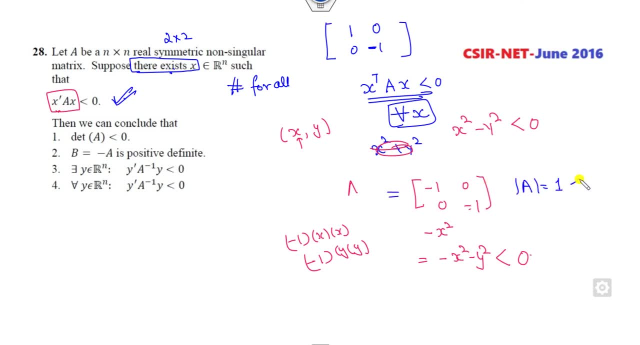 So what is the determinant of this? determinant of this is my plus 1, which is not less than 0.. Fine, What is the minus of a if I consider this as a minus of this? So 1 0, 0, 1, is it positive? definite how you can check whether it's a positive definite. 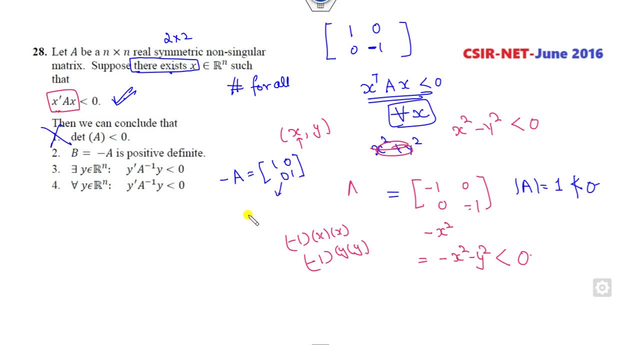 What is the property of the positive definite? all the eigenvalues are greater than equal to 0.. Fine, So how you can check that. if I simply take a matrix, like of the previous value I have taken here, What is that? this case? So, if I think about, can this be less than 0? there exists definitely. if I take, X is 1, Y is equal to 2.. 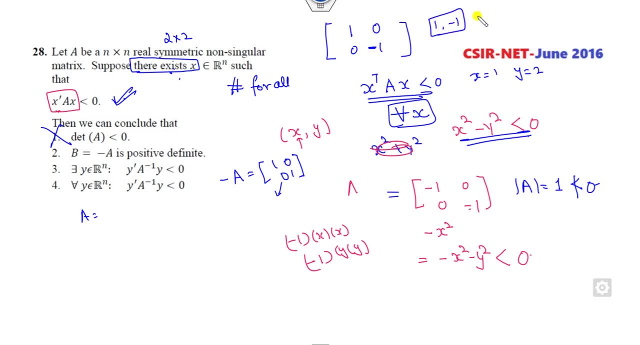 Fine, So what is the eigenvalue of this? eigenvalues are 1 and minus 1, which is not greater than 0. So it means, if this is my a, what is the minus of a Is my minus 1, 0, 1, 0. what is the eigenvalue minus 1 and 1, which is not greater than 0. 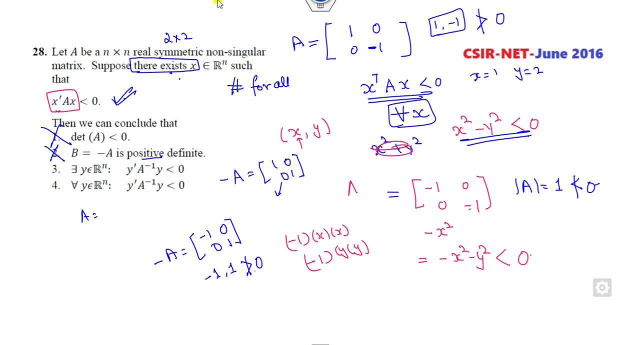 So if it is not greater than 0, it is not a positive definite. There exists Y and this is for all Y. Fine, So what is the a inverse? how you can find the a inverse? that's again a very simple, I same example I have considered. 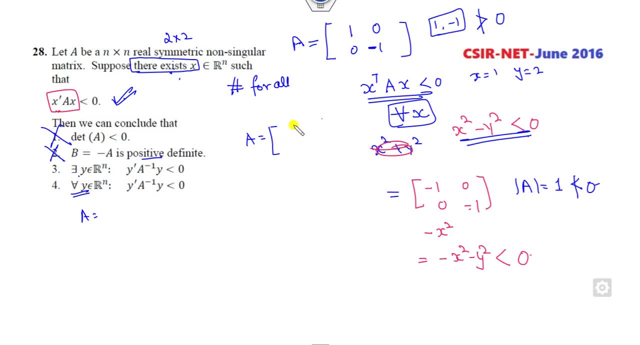 Look at that. if I take the same example like of this: 1 0 minus 1 0.. What is the a inverse of this? minus 1 0, 1 0.. Fine, This is my a inverse, sorry, divided by minus 1 also. 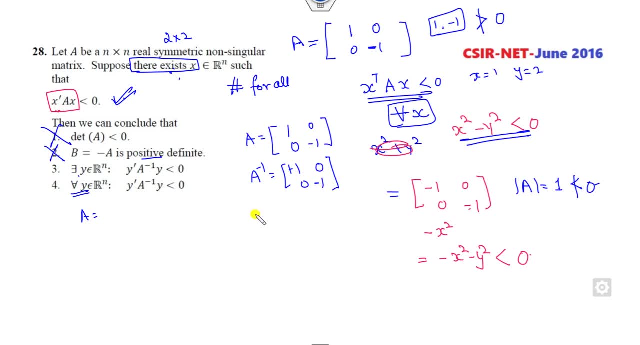 So a inverse is same. Now, if I consider the any of the vector X comma Y, then X transpose of X of this, It is my X square minus Y square. Fine, Now there exists Y means, if you can, you think about the pair of the X comma Y such that this will be less than 0.. 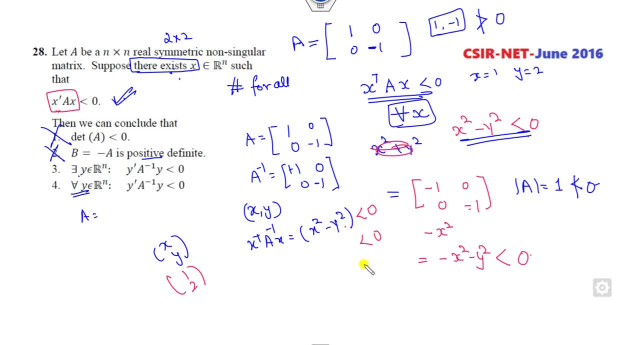 Yes, You can easily take 1 comma 2.. This is a less than 0.. That's a correct statement. But he said: for all that is not true. If you take the vector as a 2 comma 1, then it will be 4 minus 1 greater than 0.. 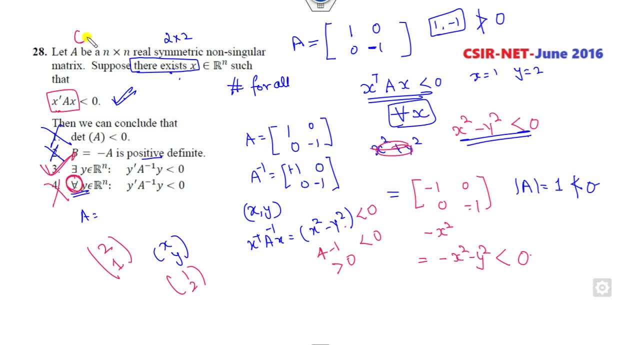 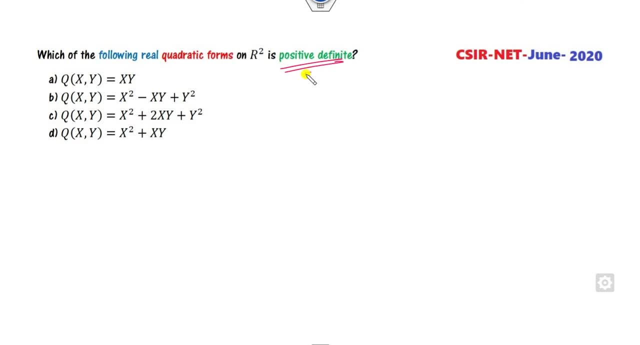 So this option is cancelled out because of this for all is my. third is the right- Okay again- is a quadratic form. What is the meaning of the quadratic form? You can write the matrix and if you find that all the eigenvalues are greater than 0.. 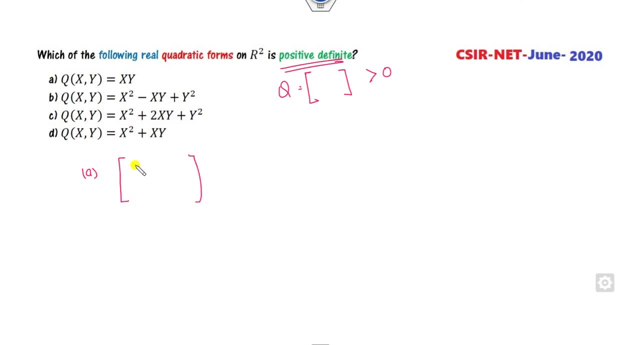 How you write the quadratic matrix, All the union variables that the original matrix called the automatic matrix. The new matrix, that is, the new matrix of the matrix called the automatic matrix That is a random matrix. What is the matrix? The matrix that is a random matrix or the random matrix? 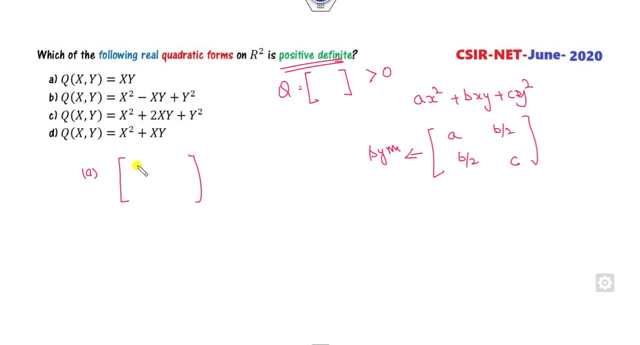 The random matrix of the matrix is in general, if it is a square plus bxy plus c of y scale, then it is a and it is C coefficient of the y, S And half of the half of the. Remember, if you find the principal minor, if it is greater than 0 means the first principal minor. what is? 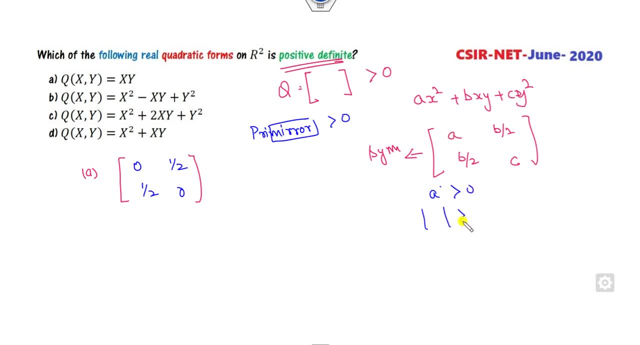 that first value must be greater than 0 and determinant of them will be greater than 0, strictly greater than 0, but the first value will be 0, so first option is cancelled. look at that how you can write the matrix: 1 minus half minus half, 1, the first value is 1 greater than 0. second, 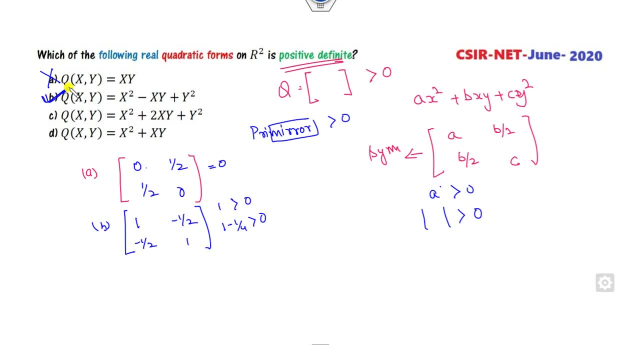 is 1 minus 1 by 4, which is greater than 0, is the right answer. look at the third pair: 1, 1, 1, 1. first value is 1 greater than 0. second is 0. which is not greater than 0 is a cancel out. 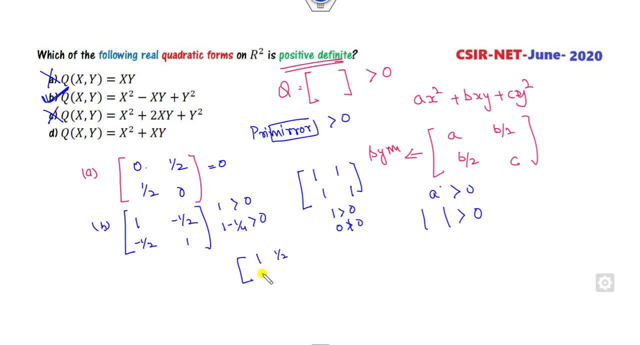 look at the fourth option: 1 half half 0. first value greater than 0: satisfied. next value is minus 1 by 4, which is less than 0, not a positive definite. this is a negative definite. once they are opposite sign, that is a negative definite or otherwise, you can. 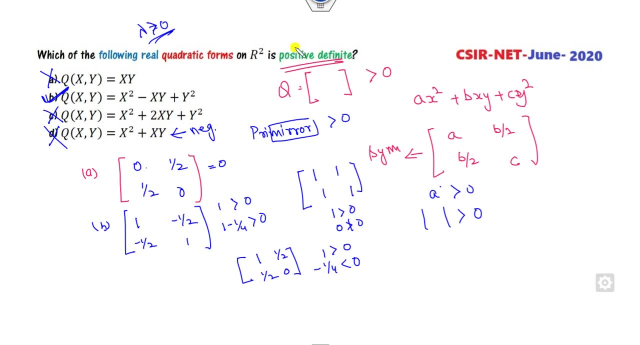 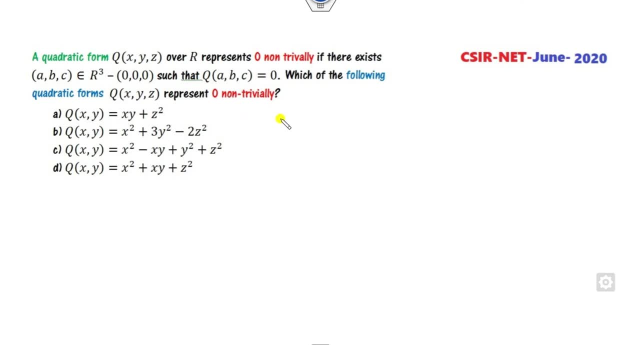 find the eigenvalues. if you find that all are my greater than 0, then it's a positive definite. so the right answer is my d. so again this is the same case. you have to find a non-zero trivial. so now it's a 3, so it's a ax square plus bxy plus cyz plus dzx plus y square plus z square fe, so a e f. 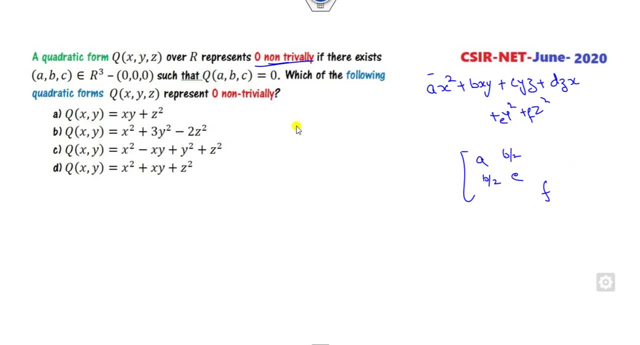 rest pair are b by 2, b by 2 and so on. so look at the first pair, x, y, z, x, y, half half rest values are 0, fine. so now can you find first pair is a 0 fine. second pair- is the determinant of this- is a minus. 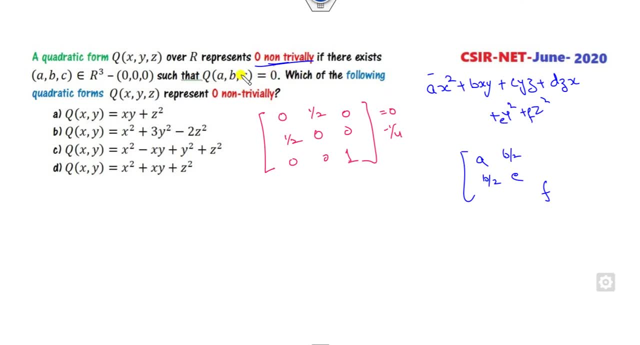 1 by 4. you have to find an, you have to find the pair a, b, c, such that this value will be whole. so you can see because we need a 0. so you can see because we need a 0. so one value of the 0 satisfied here. look at this value: 1 3 minus 2, rest values are 0. so clearly, 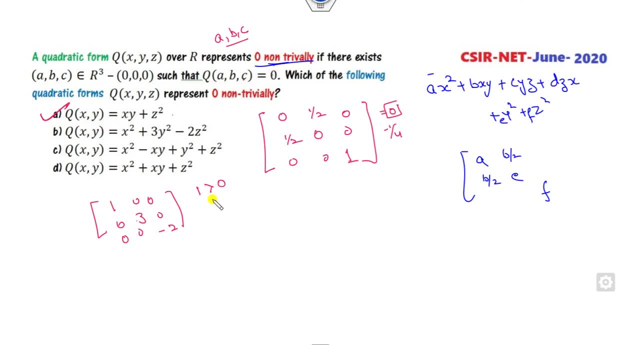 sees, the first pair is 1, which is greater than 0. second is 3 minus 0, 3 greater than 0. third is my minus 6, less than 0, but none of the value is my 0, so this option is cancelled. look at the another. 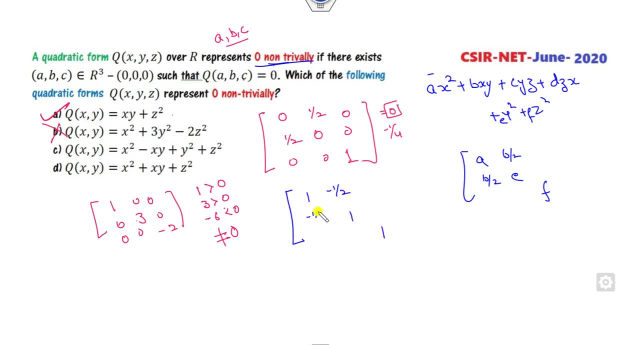 one: 1, 1, 1 minus half minus half, 0, 0 0, 0. first value is 1 greater than 0. second value is 1 minus 1 by 4, again greater than 0. third value is my itself, 1. 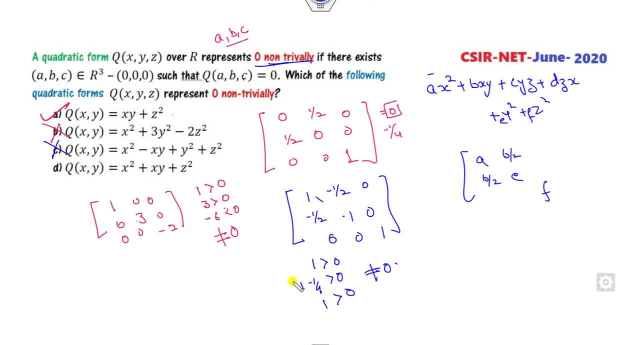 which is greater than 0. none of the value is 0, so this option is cancel. look at the last option: 1: 1 0. 1 half 0. 0. 0. 0. clearly say that one is greater than 0. second pair is 1 minus 0 greater than 0. third pair is 3rd pair is minus 1. 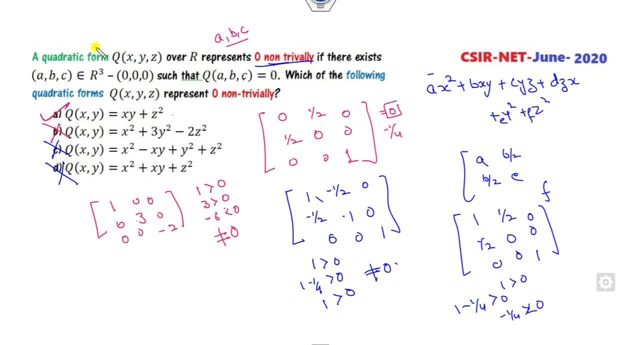 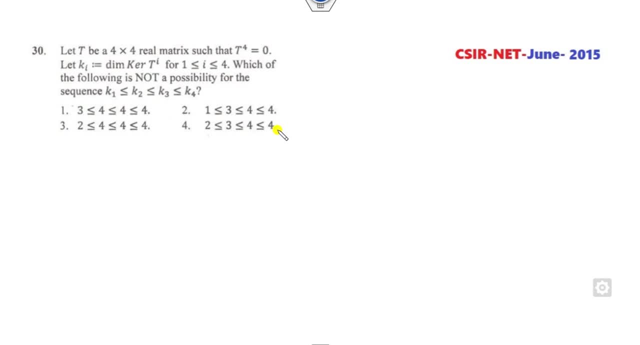 by 4 is less than 0, but it is not 0, so it is a cancel out. right answer is only a. is the correct answer? okay, which of the following is my here? this is the last question. i think yes, this is the last question. what is given to you? t4 is my, 0. what is the meaning of that? t4 is 0. it means 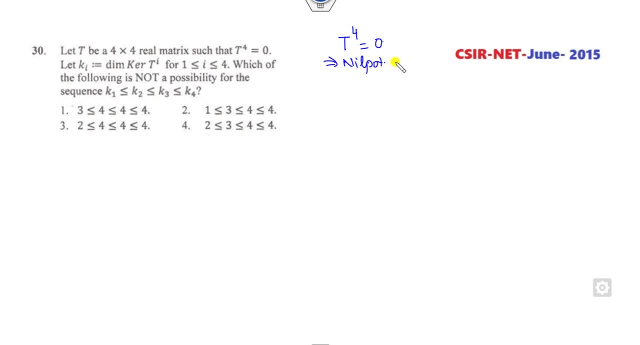 this is a nirpotent matrix. all the eigen values are my 0. it is not a diagon. k i is my dimension of the kernel of t i. that means nullity of t i. which of the following is not the possible values for the pair of x, k1, k2, k3 and so on. okay, what is the k1 dimension of the nullity? 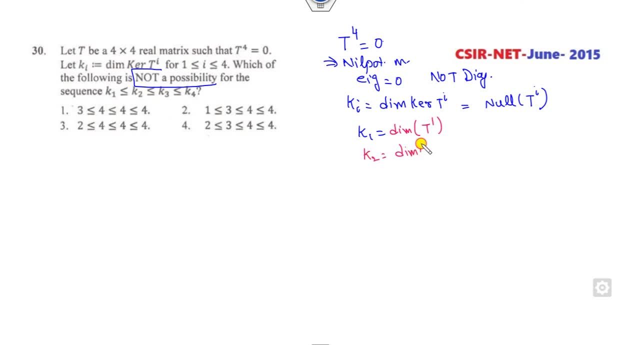 of t1, k2, dimension of the nullity of t2. this is nullity, and so on: k3, k4. which of the following is not? look at that. if you think about the k3 and k4 are always same. there is no need to check. 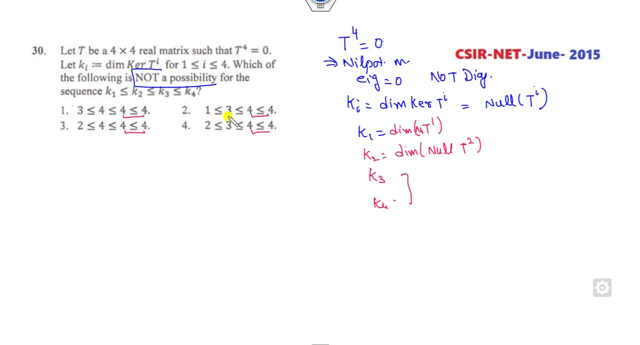 about that. we will check whether k. firstly, we will check about k1 here. so it means k1 is the dimension of nullity of the t raised to power 1. we will check whether it means. i have to check what is that size is 4, 4 minus dimension of the rank of t raised to power 1. so if it is a 3, 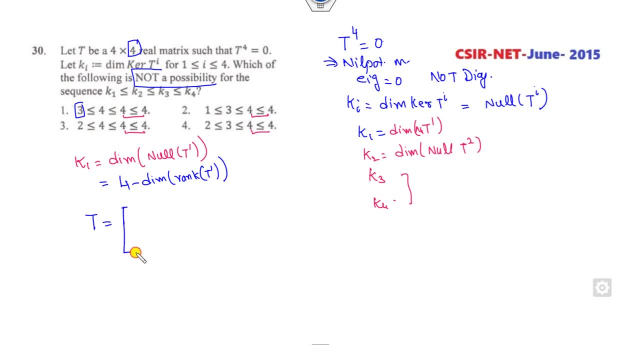 it means you have to think a matrix such that whose dimension will be whose rank will be 1, then only it will be 3 and t4 will be my 0. so can you think about that? that's very simple. you can take four rows and last value are here clearly see the rank of. 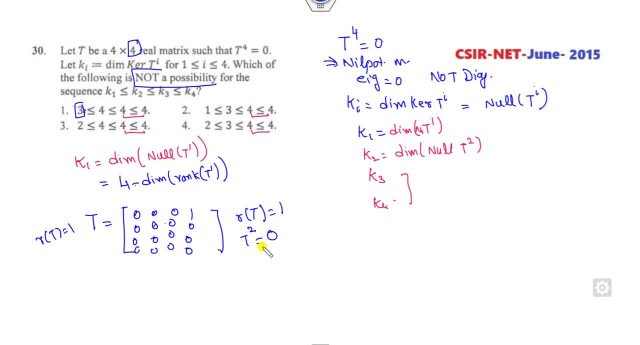 this matrix is 1, if i found the t square 0, t cube 0, t4, 0, so rank is 1, 4 minus 1, 3, so k1 will be 3. that satisfied, but we need a node, so this option is cancelled. fine, now we will check whether the 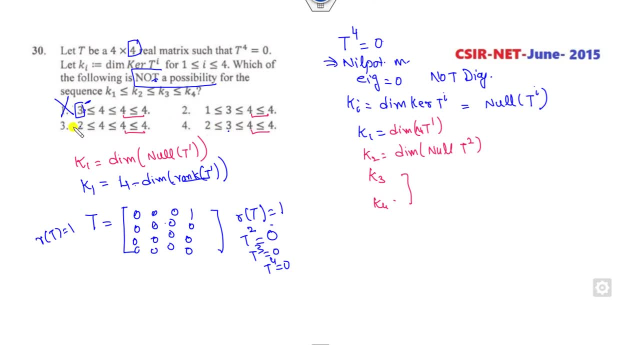 k2 how you can check what is a 2. if i check about that 2, if this option cancel out, then it is the right answer. can you think about the matrix whose 2 it means the dimension will be 2? so we can think about here. 2 row column. i can. 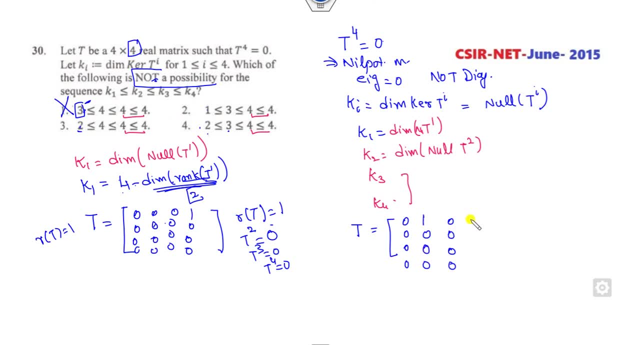 consider as a 0 and 1 here, and in this case i can consider somewhere, as this clearly says that the rank of this matrix is my 2, nullity will be my 4 minus 2 is my 2. fine, what is a t square? 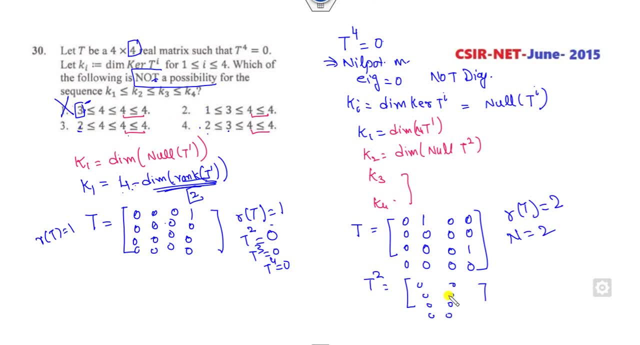 so this values are my 0- 0. so if i multiply this first row by second column, this value will be 0. second row: also 0. fourth row is also 0. now we need to check. only these values are there. so what is the answer of this? if you multiply t square into t, what will be the answer of this? it is again my.